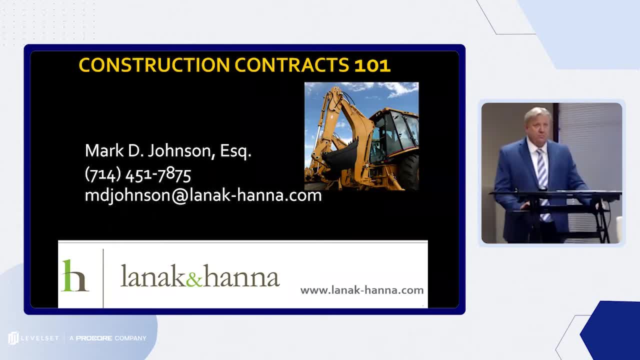 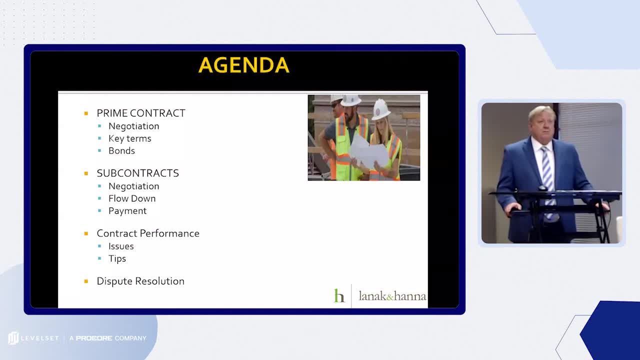 Celia, And then I'll go over fiscal contracts and contracts themselves and things to know about it. So the next slide will tell us what we're going to be talking about here today. I'm going to talk about basically the two major types of contracts, which are first, prime contracts. 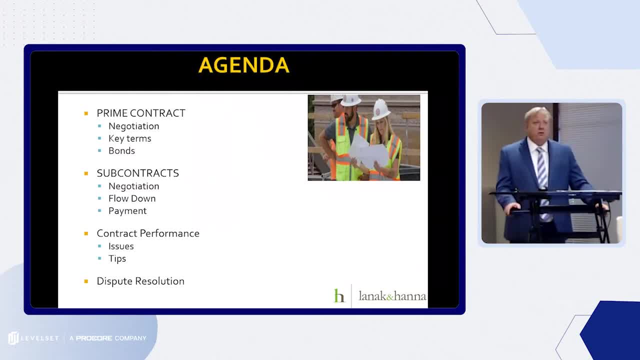 which is, prime contracts being contracts between the owner and the GC or general contractors, Sometimes referred to as a prime contract, sometimes referred to as a general contract or direct contract. Same thing, different terms. So we'll talk about the negotiation stage, key terms and a little bit about bonds. 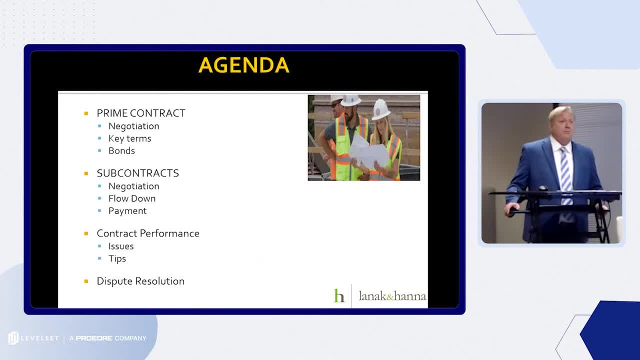 We could probably do a program on bonds by himself, but we'll mention those as we go along. Next, depending on where you are in the chain, so to speak, of construction, we're going to talk about subcontracts, which may or may not be more relevant than the prime contract topic. 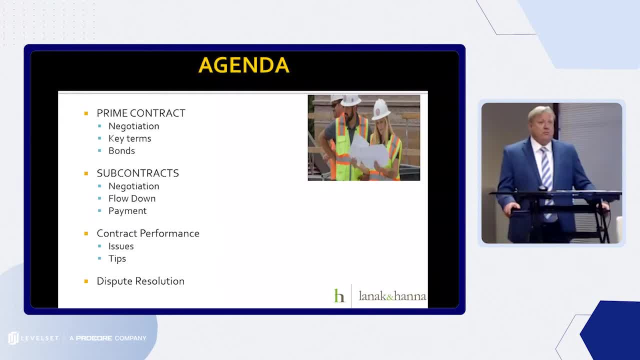 As I said, depending on where you are in the chain. So again, negotiation. the ever-popular and very, in my opinion, misused term flow down. In other words, how does the prime contract relate to or incorporate the prime contract? 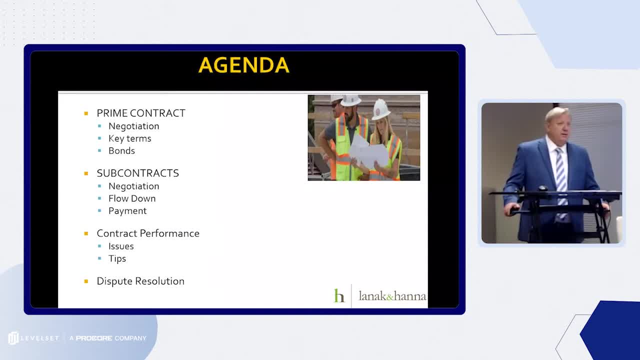 I'm sorry I may have misspoke, but how the subcontract incorporates and relates to the prime contract, And I said that wrong the first time. Payment, which of course is the lifeblood of any construction project: How to get paid? 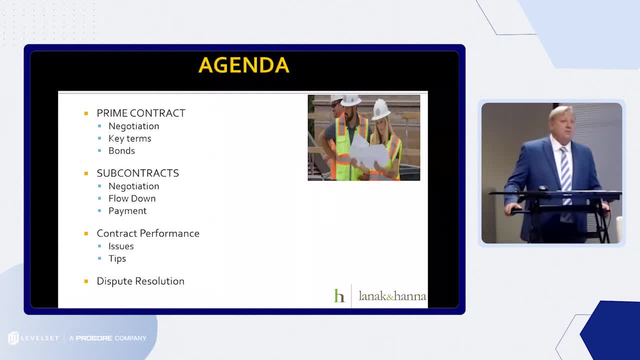 How to get that cash flow in so you can pay your folks, pay your supplies and keep on working. The next topic is contract performance: Some brief issues that obviously come up during the construction stage, the actual implementing, the scope of work and some tips on how to make your performance be set up to identify issues and prepare you if you need to actually get involved in the speed resolution process. 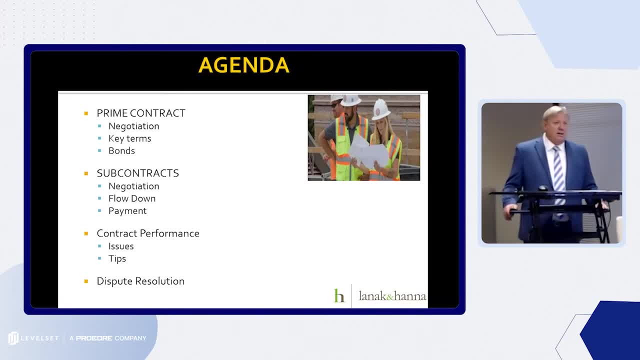 Which takes us right into the last topic, which is dispute resolution. That certainly can be its own webinar itself, but we will talk about the various ways that disputes can be resolved and pros, and a little bit of pros and cons about those ways and some issues that you can expect. 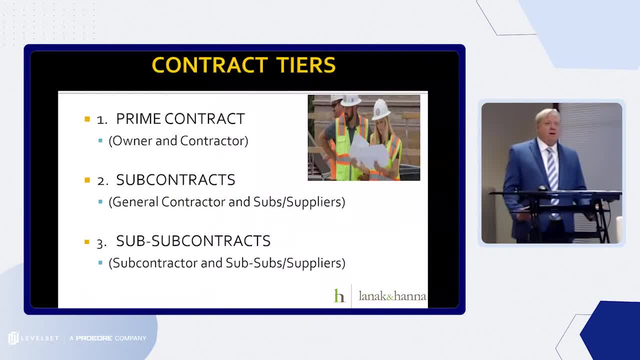 So we'll move on first to the prime contracts. As I just said, I got pretty much covered in my own slide here with my little rambling there. But The first one is the prime contract, direct contract, general contract- which is between owner and contractor. 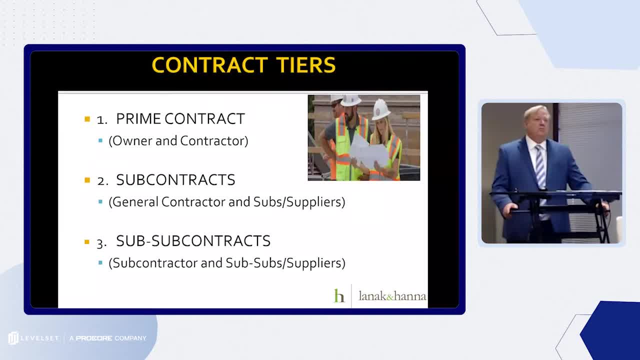 Next, sometimes called tier two contracts, which is a subcontract between the general and a sub or a supplier. And the last one is sometimes called tier three contracts, which are sub subcontract between sub subcontractor and lower tier subcontractors of lower tier suppliers. 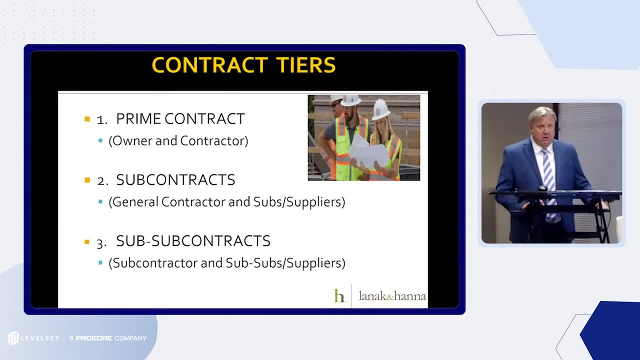 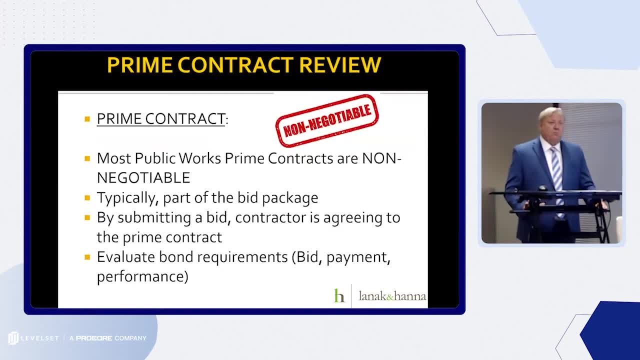 Those are the types of contracts We're going to talk about. we've kind of probably lumped the last two together, but those are the major three areas. All right, So prime contract, let's talk about negotiations. That's always the first stage. 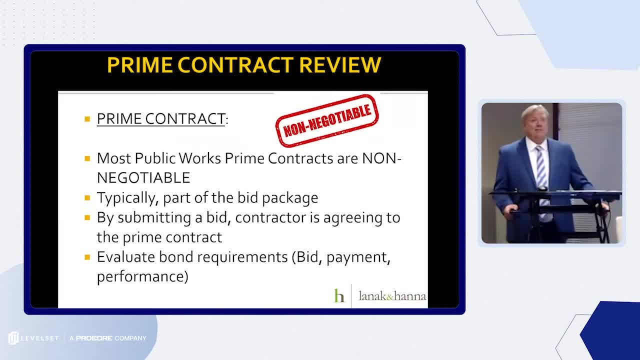 So reality is most- if frankly, very few public works contracts are negotiable. You will typically on prime contracts on a government job, a public works job, whether it's state or federal money. you're going to get a actual Exemplar of the actual contract including in your bid package. 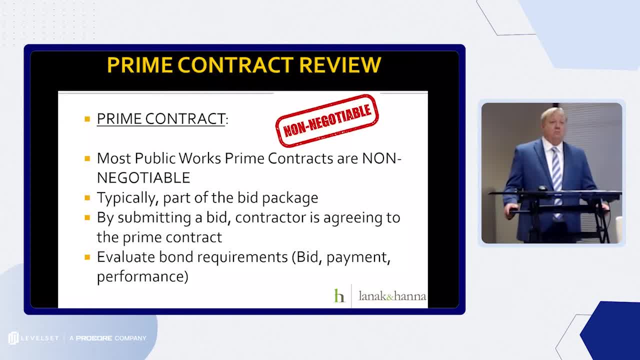 And when you submit the bid, you are agreeing to be bound to the prime contract. In other words, when you, if you are selected as the lowest responsive bidder, Which is a requirement of public contracting- you will then be accepted to sign the actual contract that was included with the prime contract. So 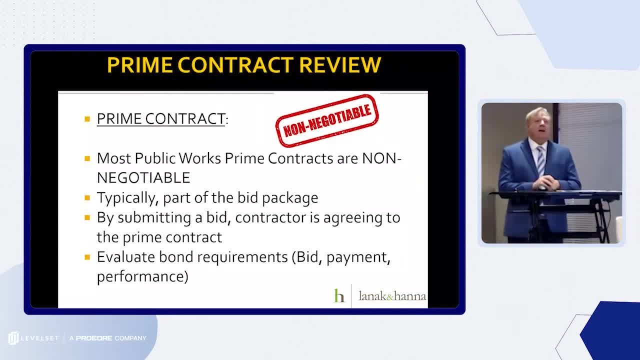 There is no negotiation, you're stuck with it, so you have to evaluate that risk when you place your bid. A couple of other things to think about when you're actually placing that bid Is: what are the bond requirements? all- virtually all- except for, in California, for example, all public work contracts that are above 25,000 dollars. 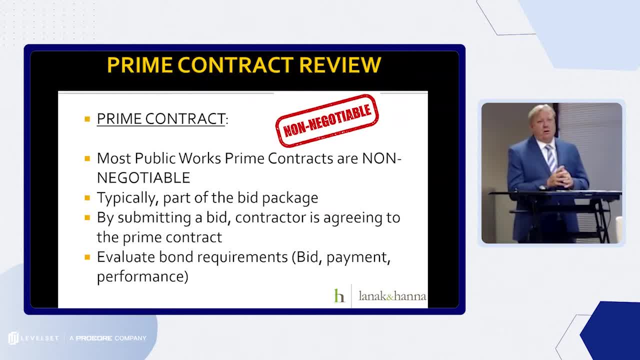 Require both payment bonds and performance bonds. They also typically require a bid bond, which basically says you're going to be bound by the bid. So when you're placing a bid on a prime contract, Make sure that you can meet all the bonding requirements that are they're set for. In other words, you have the financial wherewithal to get a bond. 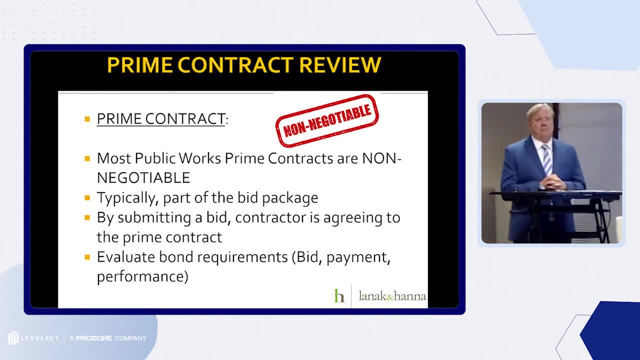 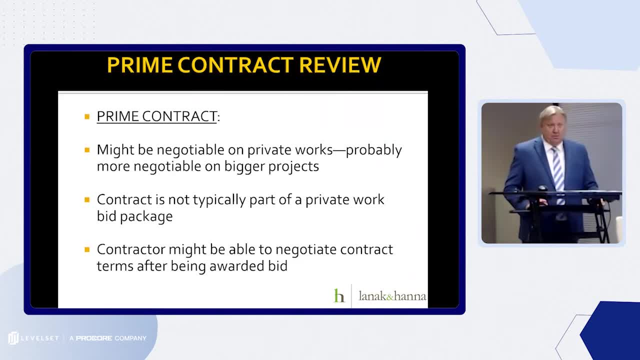 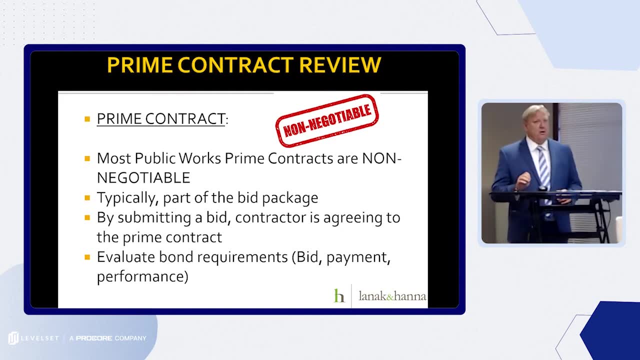 For the scope of work you're actually getting bidding on. That's and I look at the next slide, but I'll cover another topic. Let me go back to that one. The other thing to think about, including what I just said on the bond requirements: think about your subs too, because they're going to have bond requirements. They're going to flow down to them. So when you're picking your subs, 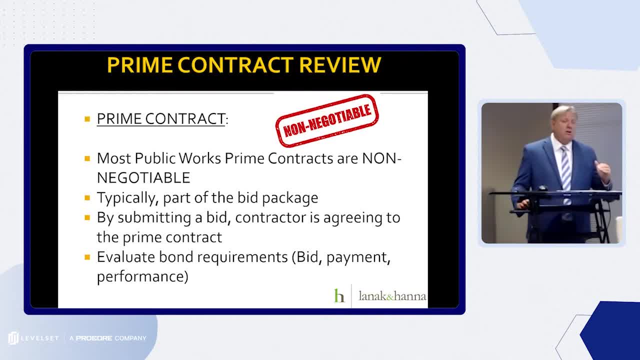 They're going to have to be. They're going to have to be, And typically in a prime contract, above a certain public work contract, Excuse me, Above a certain dollar level. you're going to have to designate who those subs are. 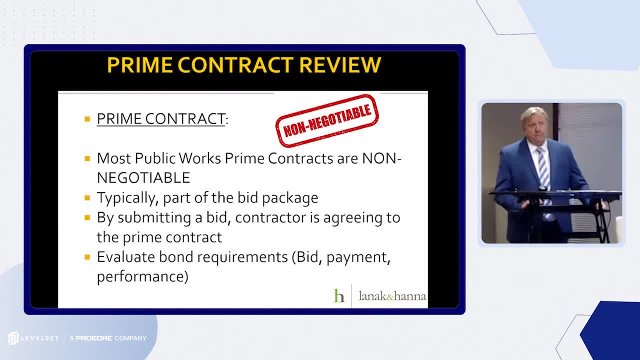 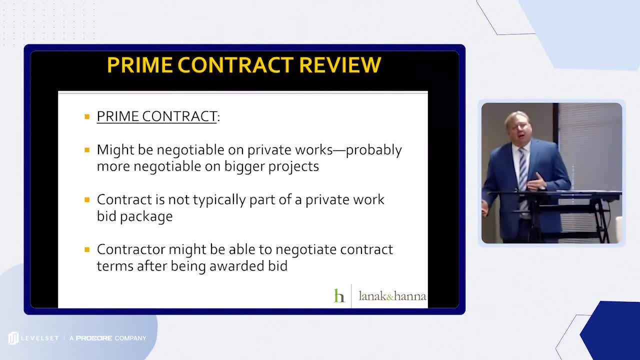 Make sure you're designating a sub that, like you, can meet the bonding requirements of the contracts. All right, now let's go with it. now to a little bit about private works. They're different Again, I think, on prime contracts. 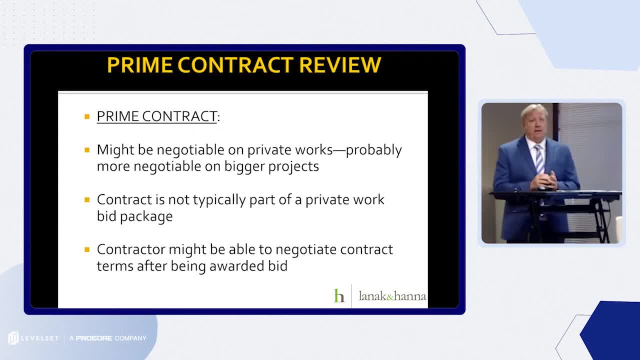 The depending on the dollar are not negotiable is probably a case-by-case basis and probably has mostly to do with your relationship with the private work developer or owner If they are submitting to bid, probably less of a negotiation If it's kind of a sole source or negotiated project as the team term. 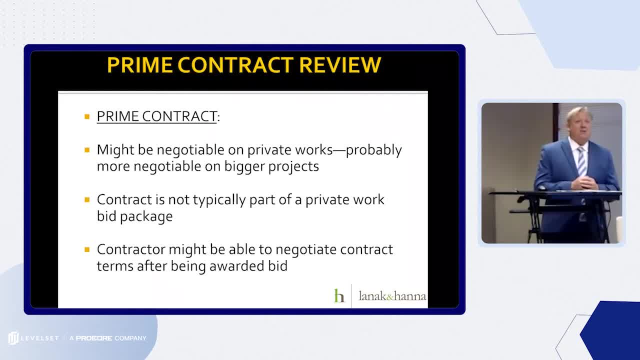 implies you're probably going to have more room. I think you're more likely to find greater negotiations, positions or bargaining power if you're talking about a bigger project, a smaller project. They're just going to say: you know, take it or leave it. 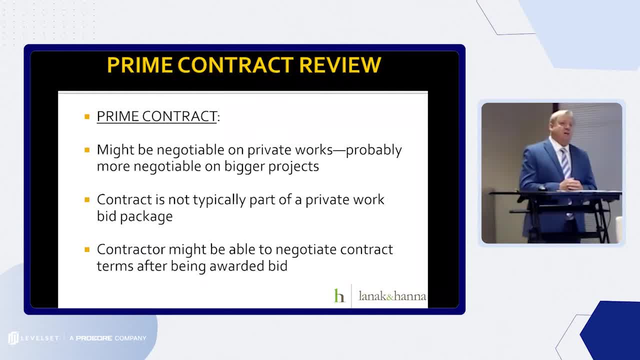 Example I like to give here. if you walk into Bank of America and you want to get a car loan, you're going to be told you're going to sign up this document right here. If you happen to be Google and you walk in and you want a $300 million loan, that's going to be a negotiation. 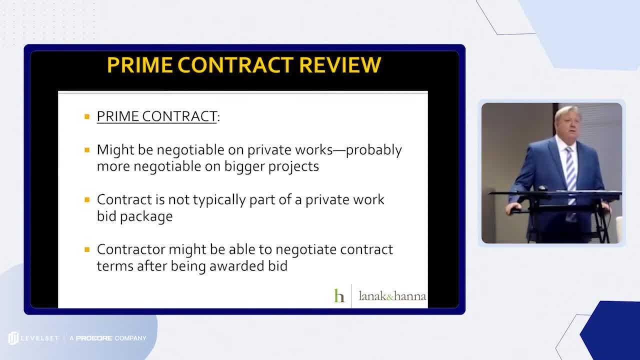 The same kind of concept applies to a contract, in my experience Again. so when you're bidding a job, rarely do you see the actual contract. when you're bidding a private work, It's more of a you know, bid the work and then we'll work on the contract, type of thing. 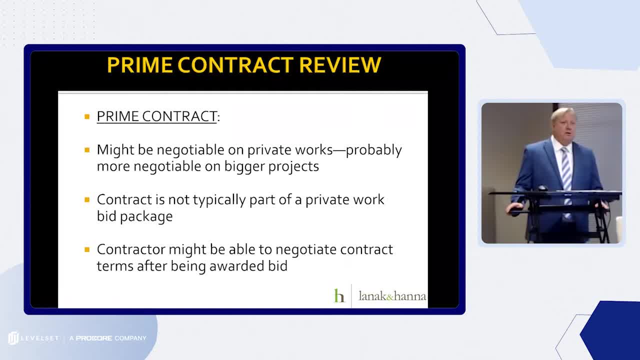 I'm just giving it typical. Of course, things can always change And you might be able to negotiate stuff after being awarded the bid, because unlike a public works developer- I'm sorry, public works owner, developer, whatever you want to call them- a private owner can certainly. 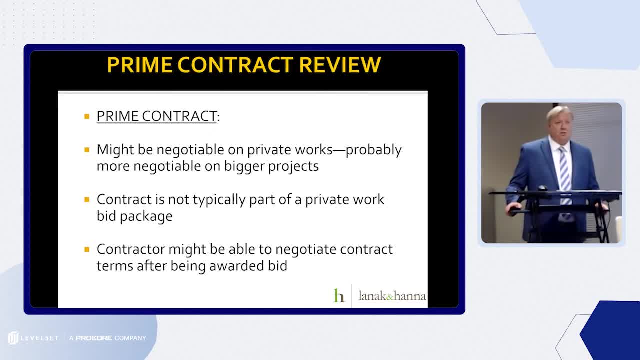 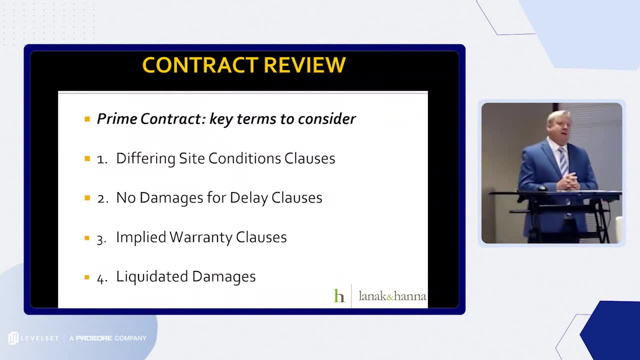 change the terms of the contract or do whatever they want. If you want to do it or not, they're not subject to the contracting laws that the federal government or state governments or local governments are typically subject to, All right. So obviously there's a gazillion clauses in a private contract that that you 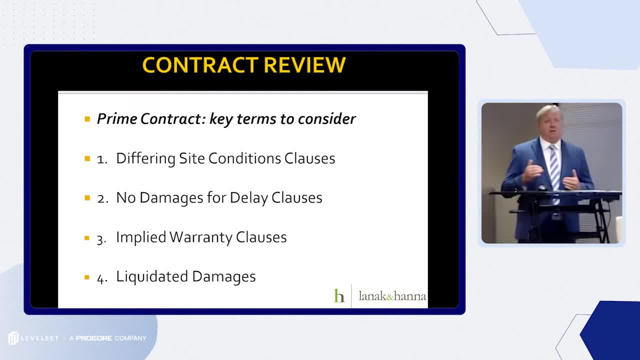 should pay attention to. These things are typically very large. It's going to have general conditions that go on for 30,, 40,, 50 pages And obviously we're not going to talk about all of them here. Just a couple of things that you know. 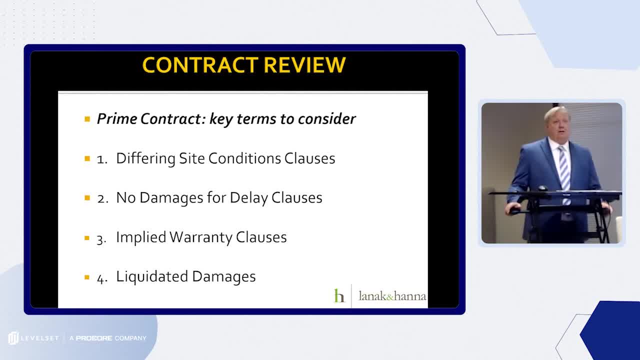 I see as being conditions that are routinely subject to dispute in prime contract situations. One is differing site conditions clauses. differing site conditions I'm sure you folks all know. but I'll just say differing site condition is: hey, we know that the contract requires us to go out here and trench. 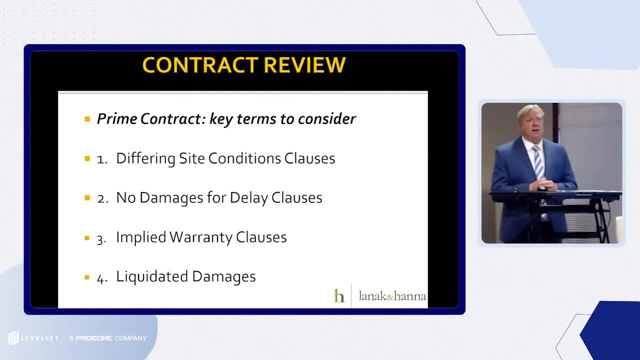 You gave me a geotechnical survey report that I relied on in terms of soil conditions And, contrary to that report, there's a bunch of dang granite boulders out here that I got to deal with. That's a differing site condition. I want money. I want time. 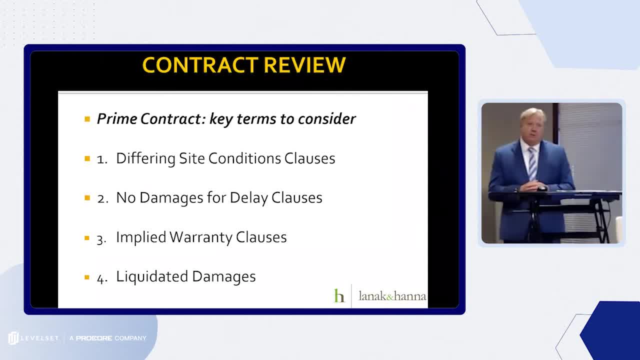 The next clause that ties right into that is: you'll typically see in a lot of public contracts, a lot of private contracts, you'll see the ever popular no damage for delay clause which says: hey, contractor, if you get delayed for whatever reason, 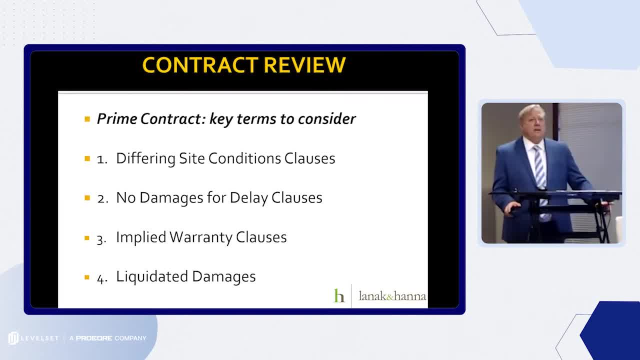 you are entitled to a time extension, but there is no damages. Interestingly enough, that clause is also kind of the corollary of that is a flip pause, which says that if the contractor delays the owner, then the contractor is liable for damages. 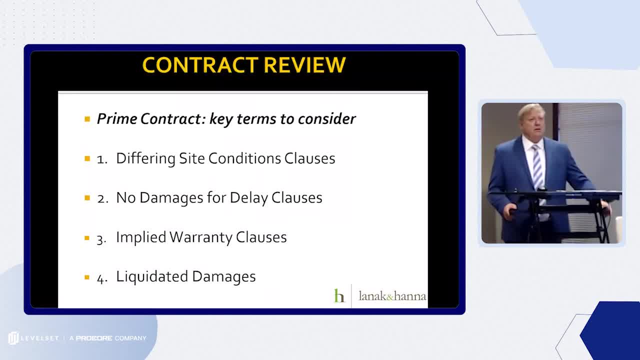 So again, if you're talking public work, these things are probably not negotiable, So you've got to assess the risk before you sign these contracts. Five warranty clauses, And we'll talk about what. some of these are, in fact, illegal in some states. 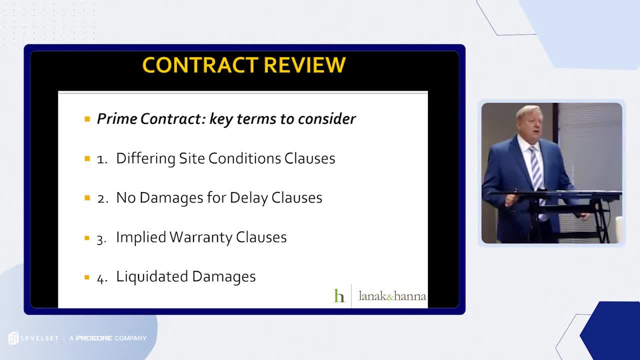 But let me talk about implied warranty contracts. It says: implied warranty contract clause says: look, we're going to give you a bunch of plans and specs, but you know what? We're not guaranteeing they're good. They might be a bunch of junk. 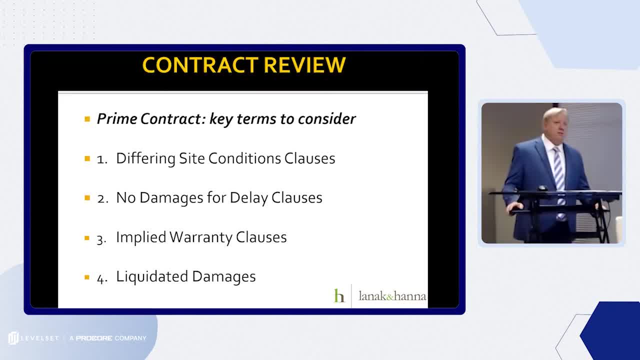 And if they're bad, that's on you, contractor. Another clause to consider when you're signing up things: Liquidated damages. These can be big bucks. So typically that clause, those clauses- are: you don't finish your scope of work yourself. 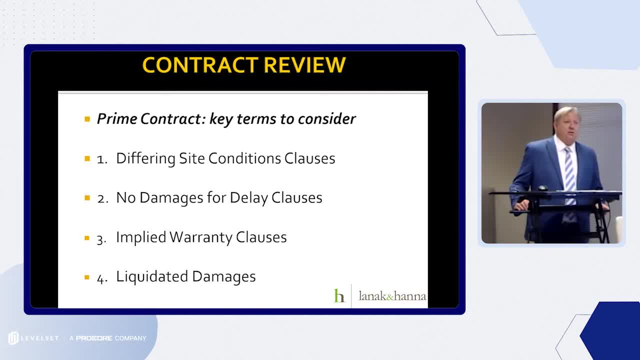 You use a construction lingo term By a certain fixed period of time set forth in the contract you are liable. You're liable for liquidated damages at a fixed dollar amount Again. so that's something to think about when you're looking at. 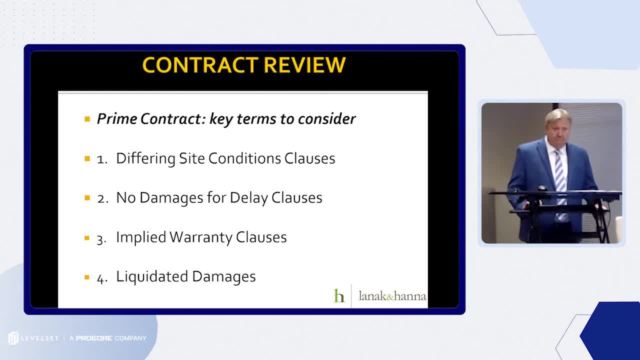 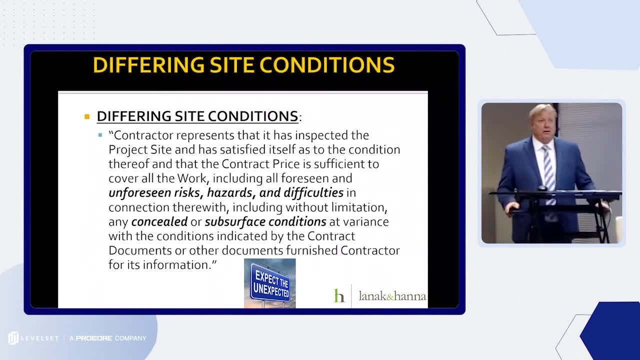 do I really want to take the risk of this contract. There we go, All right. So just this is just an example of a different site condition. I don't need to read it. It kind of it kind of goes through. 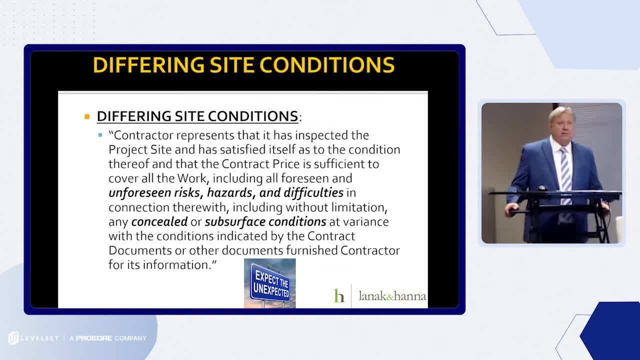 You'll see this on a lot of contracts: Contractor represents it as inspected. yada, yada, yada. I'm taking the risk, as the contractor, of unforeseen risk hazard. I also take the risk of areas where all these individual contracts have been. 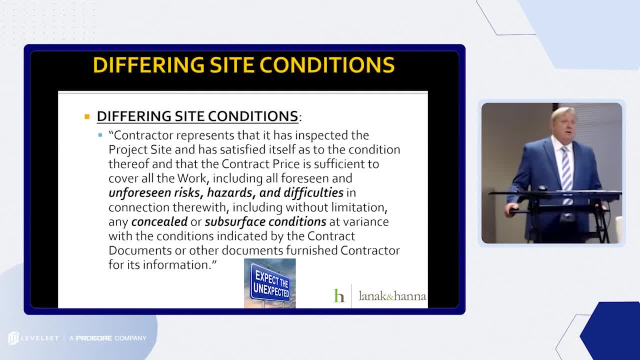 disbanded. all these contracts have been disbanded because there's been some difficulty and even stuff in the subservice that there's no dang way I can figure out right. So you're buying that you know all these causes. I'll say: 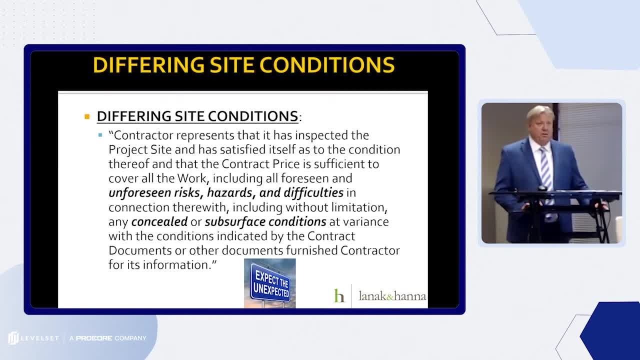 You know you might be able to if you've actually got to the speed. there might be some arguments, but these are clauses you're gonna have to deal with. I don't know if the next slide deals with this, but I'll tell you. another thing to be concerned about here is there's going to 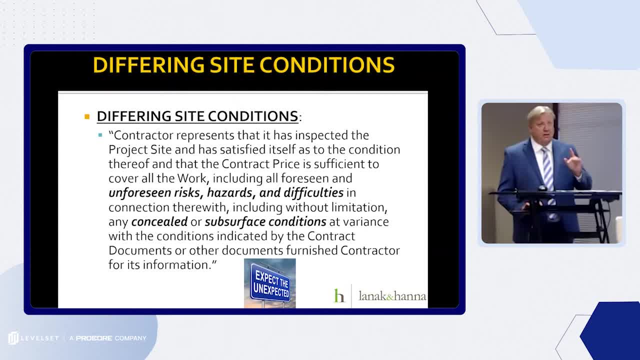 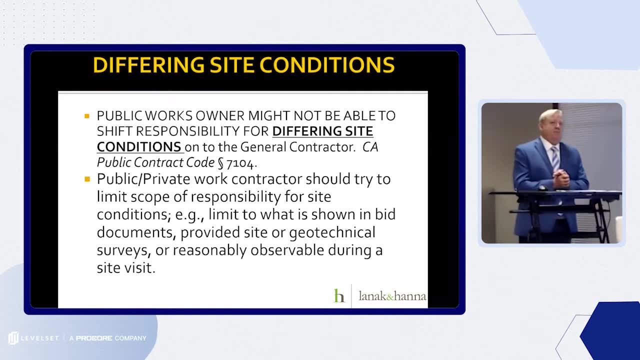 be a notice provision in all these contracts that says you did encounter certain conditions, you've got a certain period of time to provide notice. um, i think we get into detail about that a few slides later. all right, so public works owners might not be able to shift responsibility for differing 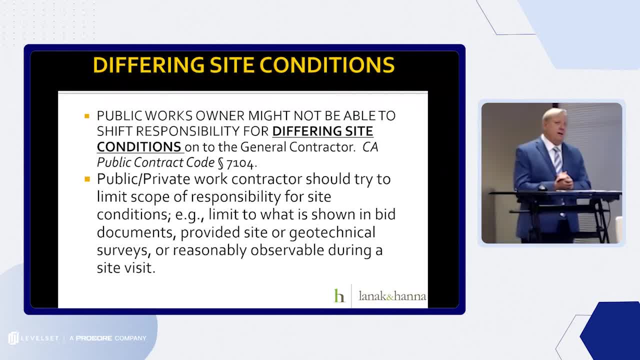 site condition onto the general contractor. for example, california public contract code section 7104 makes those illegal in california. i don't know about other states, i know about california. public private contractors should try to limit scope of responsibility. if you've got any ability to negotiate, try to limit it with clauses such as you know. um, i'm relying on what's in the 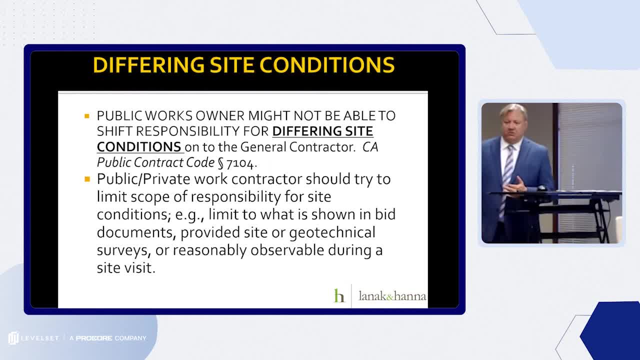 big documents. i'm relying on what's in the geotechnical survey, sometimes referred to as the gdsr, or reasonably observable during a site visit. you know the topic of that last bullet. there was public, private. obviously, on a private work, you're going to have a much better idea that you. 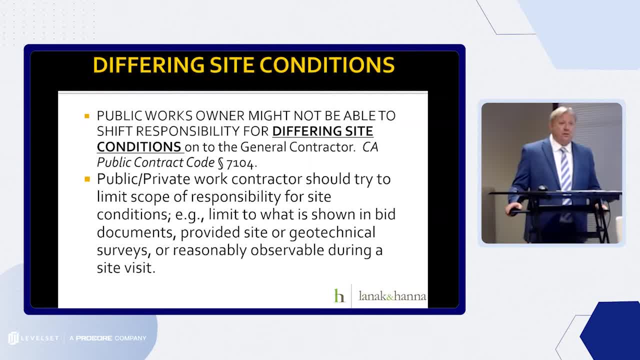 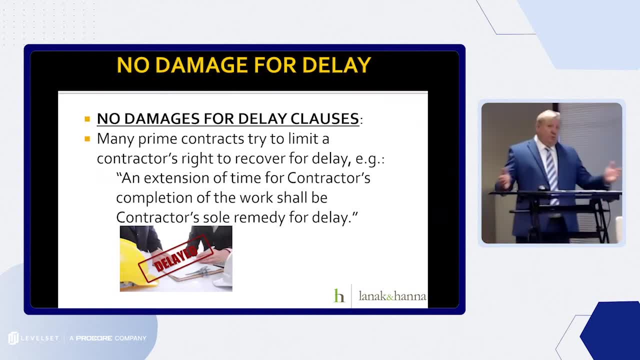 can negotiate that are much more likely, that you can negotiate that clause: no damages for for delay. so this is uh, i you know, obviously grace. we talked about it second, but here's an example of the clause: an extension of time for contractor completions of work shall be. 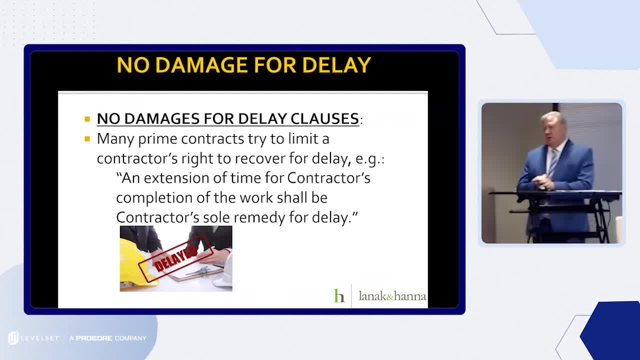 contractor's sole remedy for delay. so the owner's going to take a position that it doesn't really matter what the heck happens. um, they could, you know, delay the project, clearly delay the project. they could fail again. give you power to the site. it could be, you know, all kinds of things. they could decide that you. 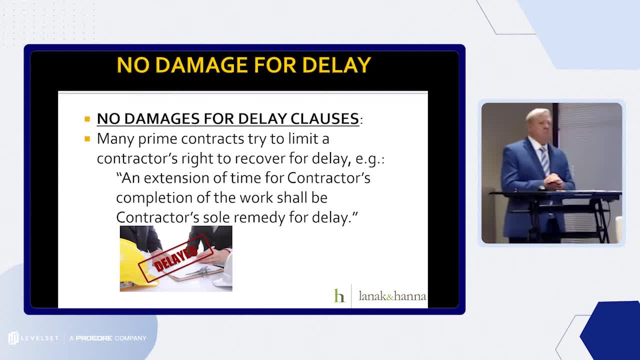 know, we're not going to build a two-story building, we're going to build an eight-story building. and hey, you know what buddy contractor, you're going to build it and it takes you longer. that's your tough luck, um. so let's talk about what to do with those clauses. so again, california's going to help. 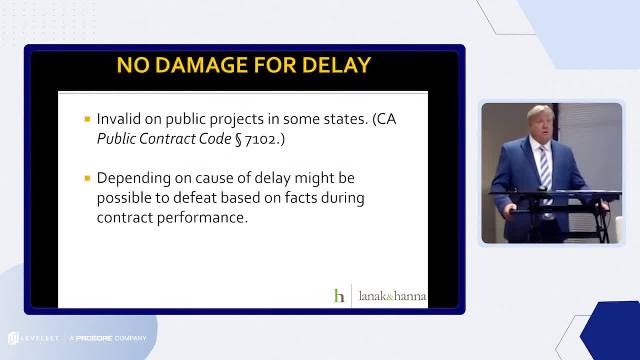 you out here. so california public contract code 7102 says that's invalid on public projects. so you have to check your own state and see if it's valid on your state for those clauses. if it's not, if it's just if it's, if it's a clause, it's not invalid. 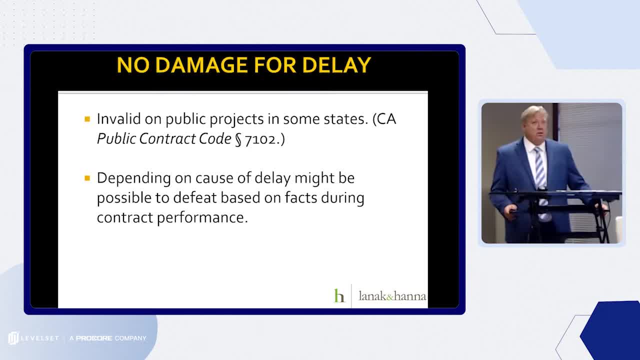 you've got. you've got arguments. the way these clauses really work out if you look at the case law is you got to figure out what the facts are and whether there's really an equity situation that that comes into play here that makes it unreasonable and unjust to enforce the clause. 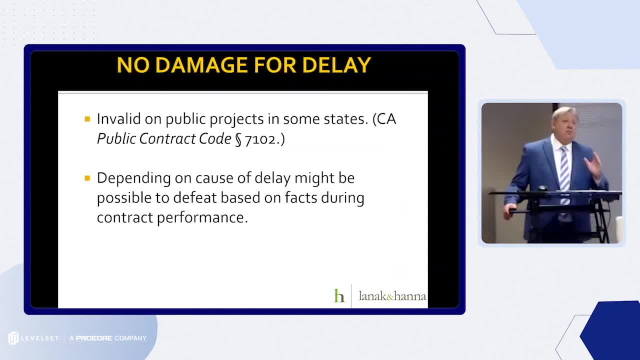 my example of going from a two-story structure to an eight-story structure, i think would fit within that clause. if you've got a project and there are, you know, 150 design changes and your price to complete goes from, you know, presently doubled, you've got a really good. 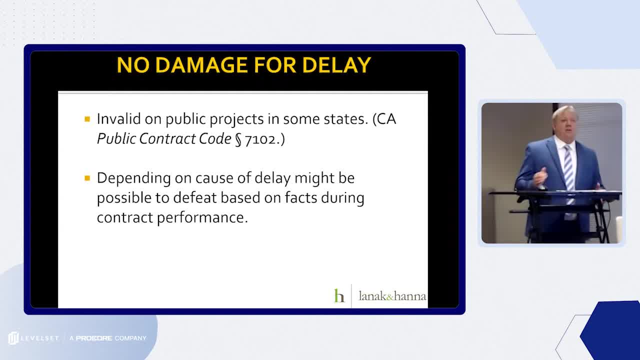 argument that clause is invalid. big picture concept for me is that in all the cases, whether it's a judge, it's a jury, it's an arbitrator, at some level there is a decision that's going to be made by those folks: who is right, who is wrong, who's the good guy, who's the bad guy, and i can. 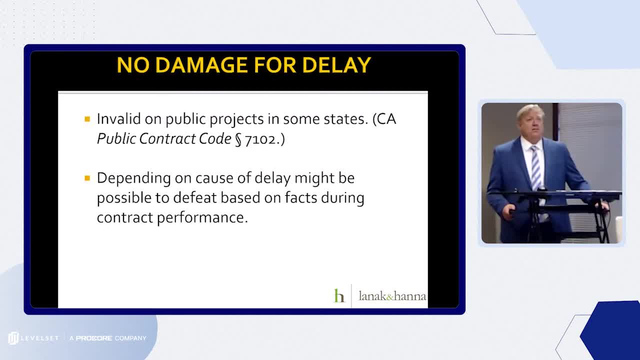 say in a large times their morality plays and they pick the good guy, they pick the bad guy and they do right by the good guy and they screw the bad guy. you got to be on the right side. that's going to be very fact-dependent. if you're going to try to get out of that, no damage for delay clause. 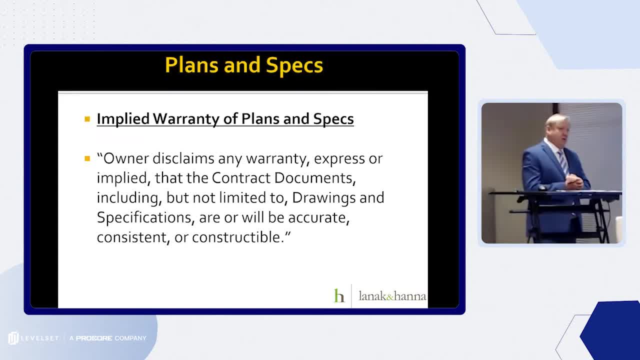 uh, all right, so this is the one i covered briefly a little while ago, so this is the last one about this, and then i'll call it. the typical clause holder disclaims any warranty. expressor implies the contract on blah blah blah specs are or will be accurate, consistent. 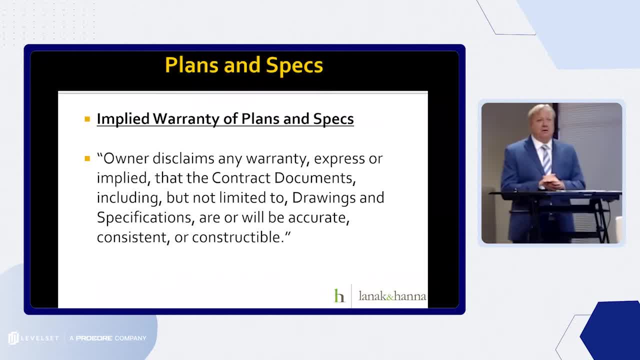 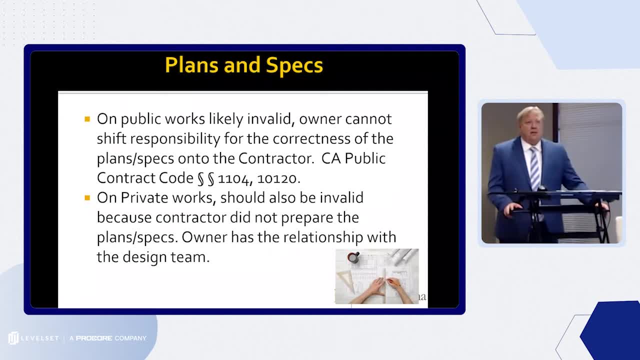 or constructible. in other words, these will give you these documents, but geesh, i don't know, i'm not very good. um, so now morning, once again is going to say that is not valid. california public contract code. the section by site will say that that is not valid. 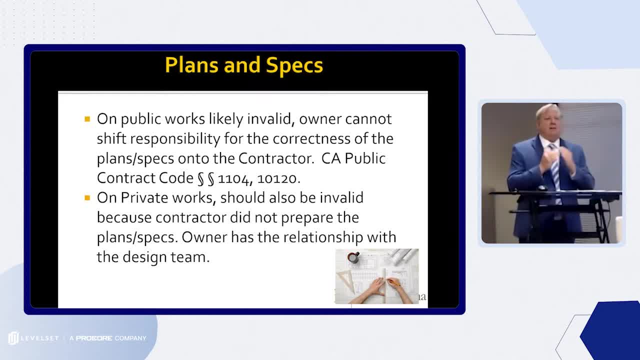 job. i think you have a, you know. let's just talk about something. try to negotiate something like that up front out of the contract. if you're dealing all these clauses that are bad, if you're on public, private work and you can negotiate, try to get them out of there. uh, if you're faced with 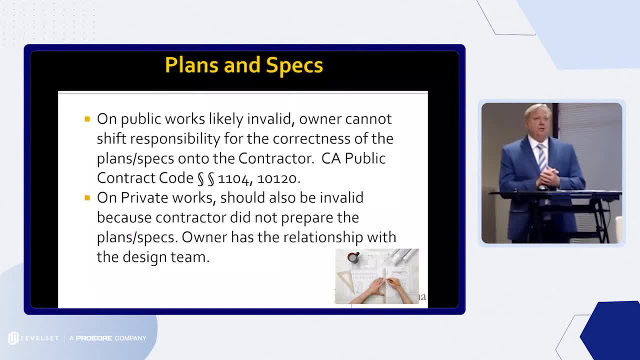 having to deal with them and they're in there. you, you know, you've got arguments. it's really like i say here: you didn't hire the con, you didn't hire the designer, you didn't hire the engineer, so it really should be the owner that should be on the hook for that. so that's where the equity. 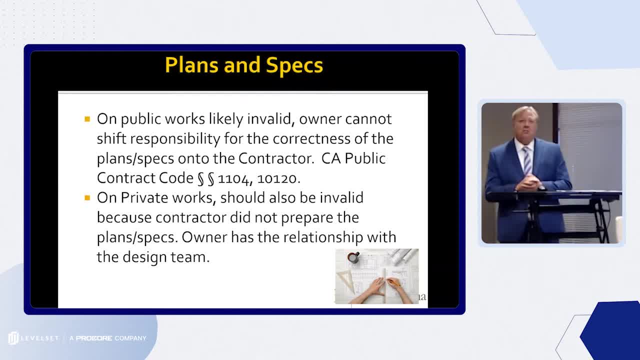 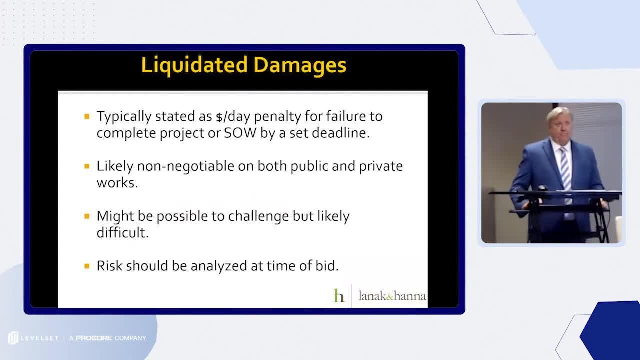 process comes into play. but it's much better off to deal with that up front and get it out of the contract rather than having to hire somebody like me go fight that thing for you. uh, liquidate damages is the last one we're going to cover. like i said, there's 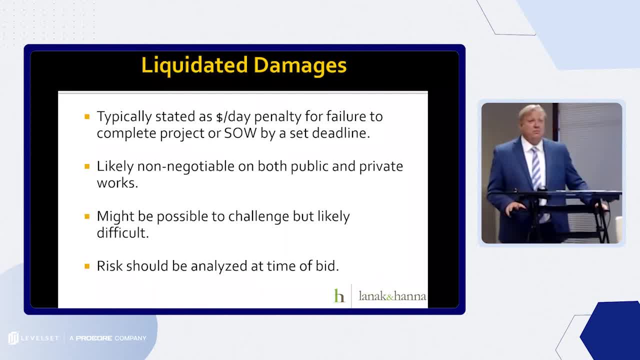 a lot more clauses we could talk about, but you know we're trying to limit it to some of the ones that are probably most problematic. all right, like i said, this is typically how this works is. contractor has a fixed period of time to do its scope of work, or sal if they shortened it there. 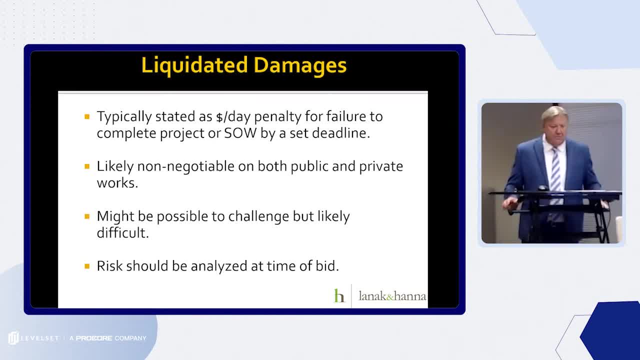 um and um. you know, just hypothetically, you've got 90 days to complete this project, the the scope of work. you don't complete it by x time, you will be subject to dollar day penalty. um, that's probably non-negotiable. it's probably non-negotiable on both public and private works. the reason i say: 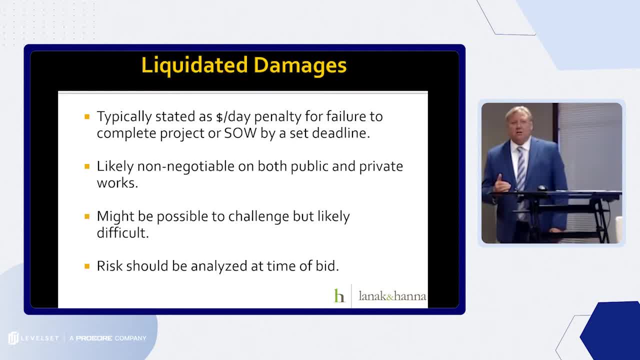 that is, typically. those clauses exist because they are tied into some other contract. for example, i've done litigation about power plant projects and the contractor- the owner- has made a deal with the, or the owner- developer- has made a deal with the, with the public utility that we're going to bring you x kilowatts of power by x date, and they're subject to penalties. 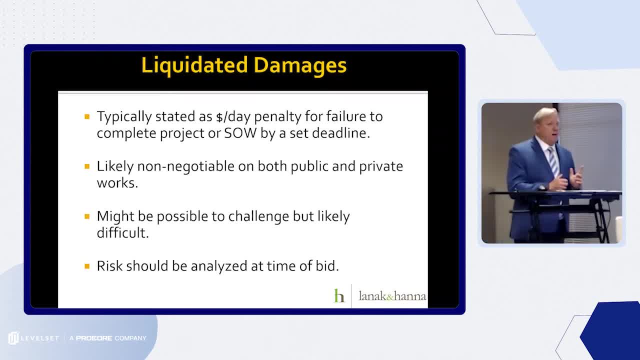 so that's why they're sometimes not negotiable, on either both private or public works jobs. Again, you know these are clauses that you might be able to, if you can negotiate them out. you should try to do that, Or, if you can, try to limit them. 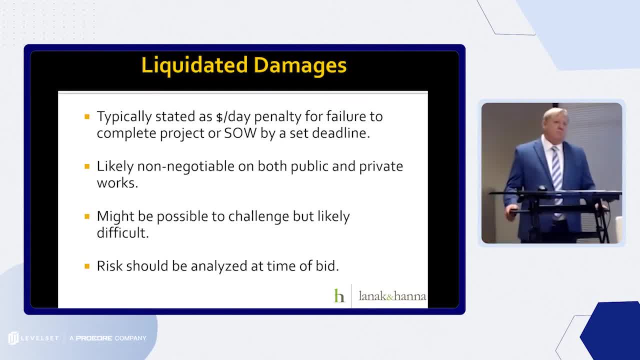 It might be possible to challenge, if you have to, after the project or if you're subject to a speed resolution provision. The way you do that is. there are requirements that how much liquidated damages are and whether it's fair. You know you can argue. 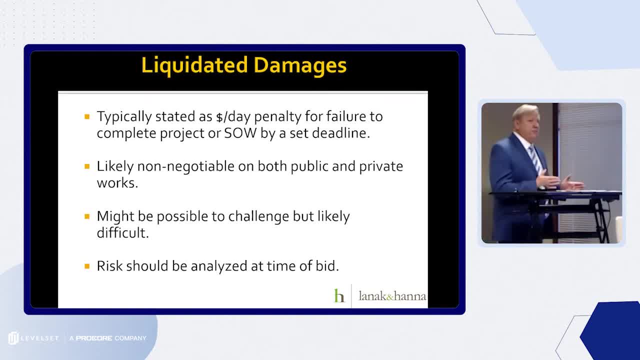 about whether you're actually the cause of the delay or whether you have some reason that you were delayed. It's not your fault. If you can blame on someone else, you might be able to also challenge the liquidated damage concept itself in terms of it being invalid In California, for example. 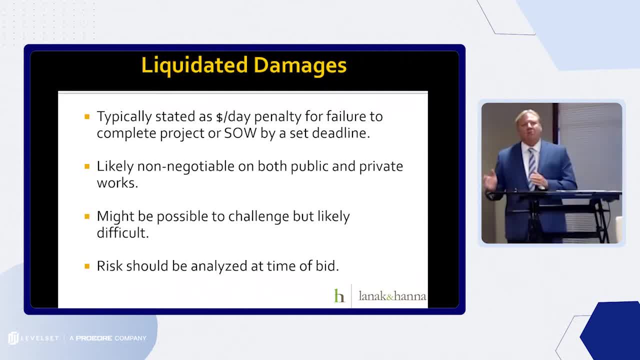 liquidated damages are only available if it is difficult or impossible to assess actual damages, and the liquidated damages provision There are reasonable or reasonably based on what actual damages might be. In other words, they're in the ballpark. So, for example, if you've got, let's just say: 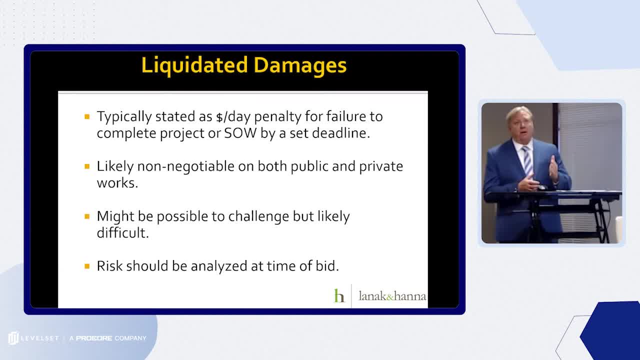 you've got a $1 million scope of work contract and the penalties are $500,000 a day. that's probably not a reasonable liquidated damage clause. But again, you know, try to negotiate it out if you can. There's some arguments you can make. 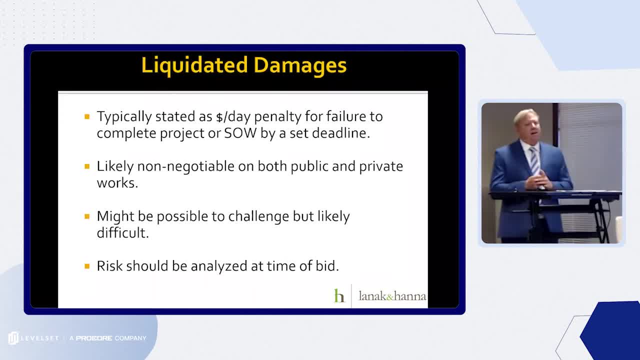 Final thing on that is: you really should. if you can't negotiate it out, you've got to analyze the risk and time of death. You know construction at risk. there's a reason why there's, you know people do it and there's a reason why people lose their shirts doing it. 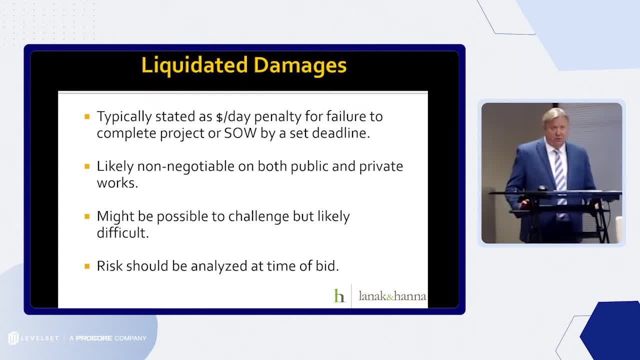 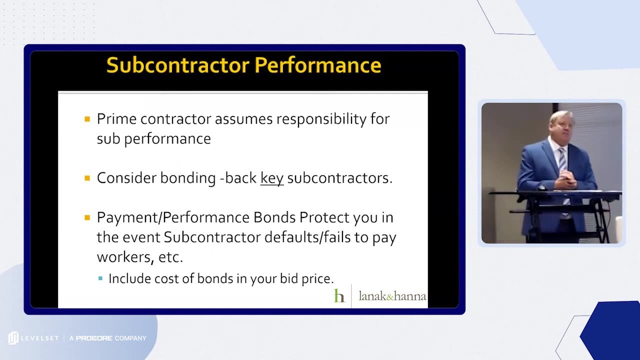 So all risk needs to be taken advantage of when you're making a bid. Let me grab some water here and then we'll go to the next slide. All right, So prime subconscious Contractor performance is so obviously. prime contractor assumes responsibility for. 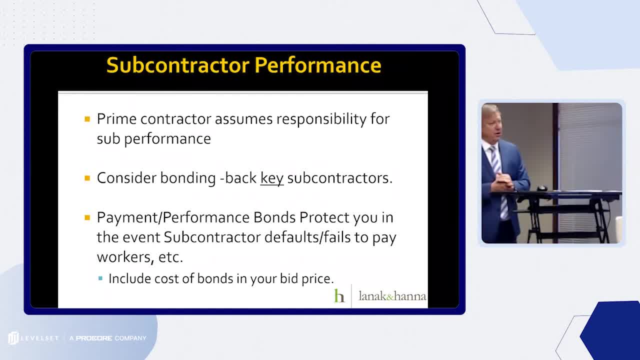 sub-performance. So when you're talking about the owner, the owner's going to say hey, hey, hey, hey, that part of this work is not good, Part of that work is effective. The electrical is late. The general contractor can't say: 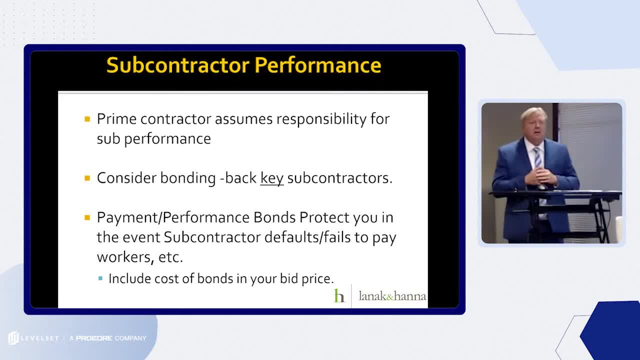 oh well, hey, I didn't do the electrical. Why are you talking to me, He or she or it? whatever you want to say is on the hook for the sub, despite the way they did the work, And obviously most of us know. 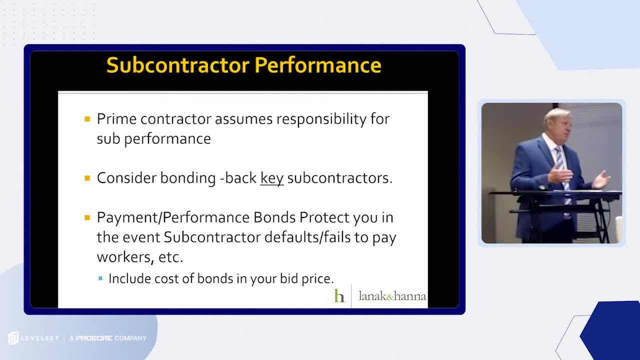 that general contractor. unless you're talking heavy civil, where there is some sub-performance, most general contractors don't actually do any physical work on the site. So here's another thing. So what all that first point ties into is you've got to make sure that if you're taking on a project, 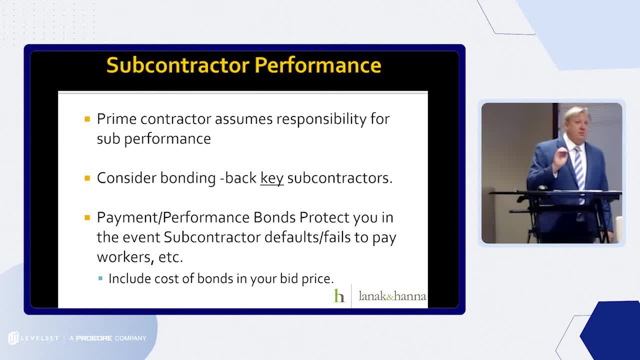 where there's substantial risk of performance in terms of penalties, in terms of you know no damage or delays, and a lot of clauses that can come back and bite a contractor when you're making a bid at the GC. you've got 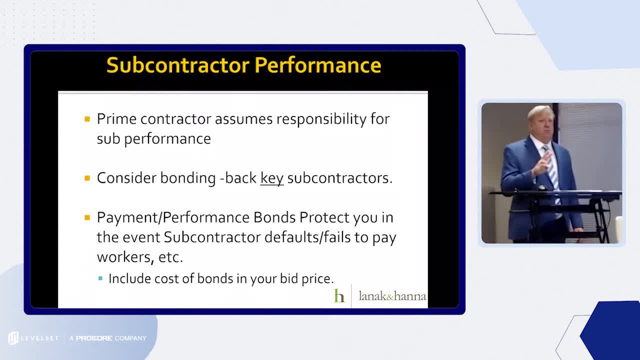 to consider. okay, my subs and I rely on my subs to perform, So there's a couple ways to help you out here. You can consider bonding bonding back to your sub, which means you get a bond in your favor on the subcontractor. 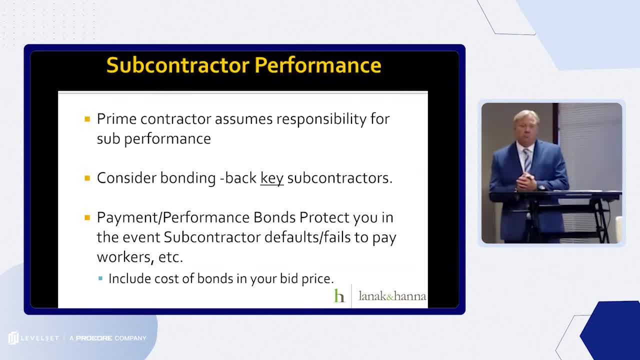 There's also something a little bit newer- not really newer, much newer- but it's something called subcontractor default insurance. We'll talk about another webinar on that in a little bit, But essentially similar to a bond, but the advantage is in a bond. 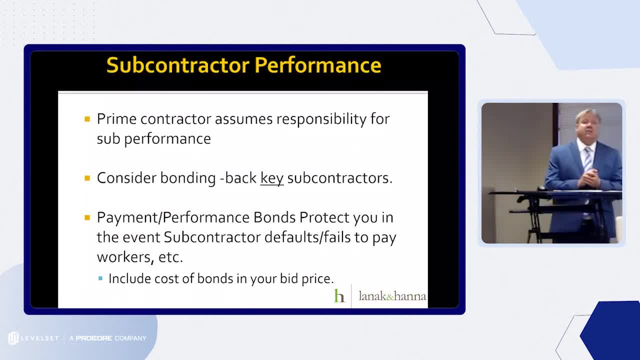 the bonding, the company or surety decides that there's actually a default and a subcontractor default insurance policy, the contractor decides that the subcontractor is then default. But once they do that they run the risk that ultimately the insurer will not agree with that decision. 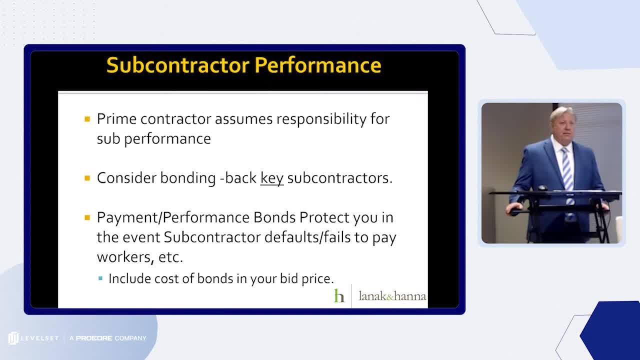 So that's a topic we can go into much more depth, but that'll kind of hit the highlights for now. So just because just real briefly and again, you folks probably know, payment performance performance bonds protect you in the events of a contractor default, fails to pay workers. 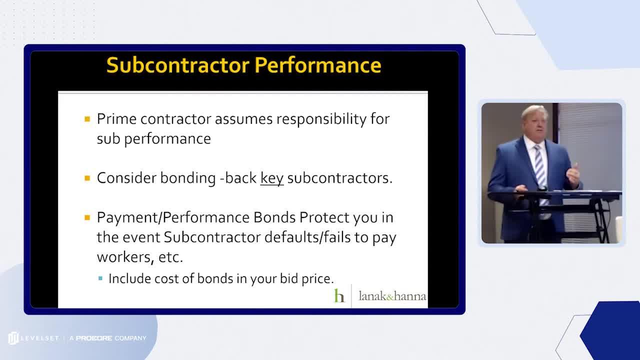 So when you're thinking about a payment bond, that is a bond that is there for a sub that says that if he or a buyer that says if he doesn't get paid he can go to the bond. Performance bond basically deals with if the contractor or subcontractor doesn't finish the job is in default. 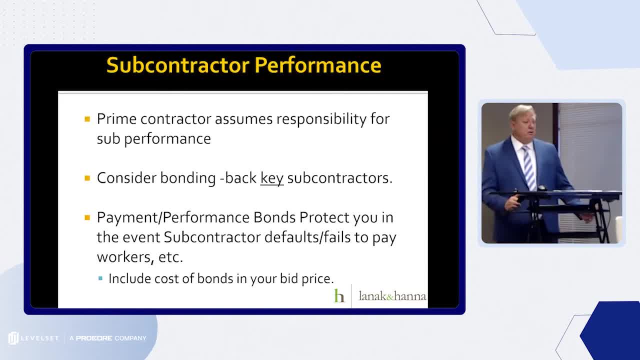 And then the bonding company takes over and does responsibility for the completion of the project. They hire the contractor, They can take over the project. There's a variety of remedies that a bonding company can take. If you're going to do that, if you're going to bond back yourself, you're obviously buying yourself some protection. 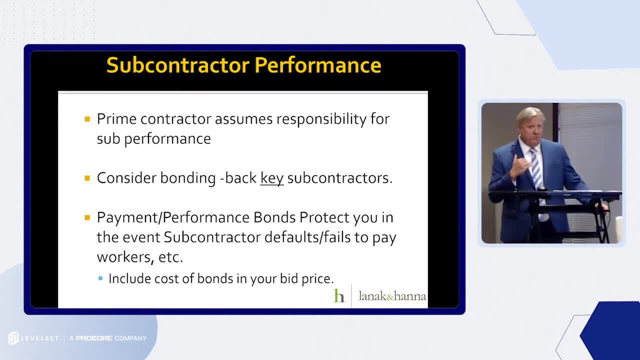 or if you decide to get subcontractor default insurance or SDI as it's only referred to, make sure you're putting the cost of that stuff in your bid price because you're going to be on the hook for that, Unlike the, you know you're not going to. 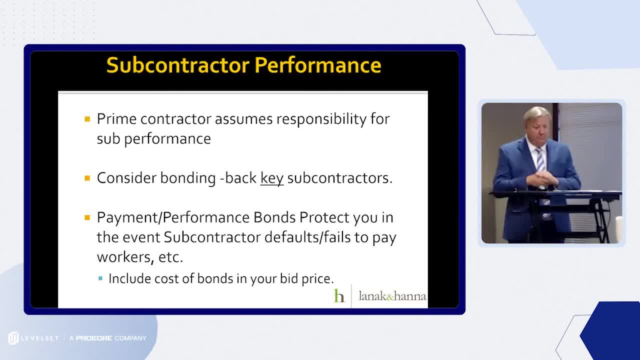 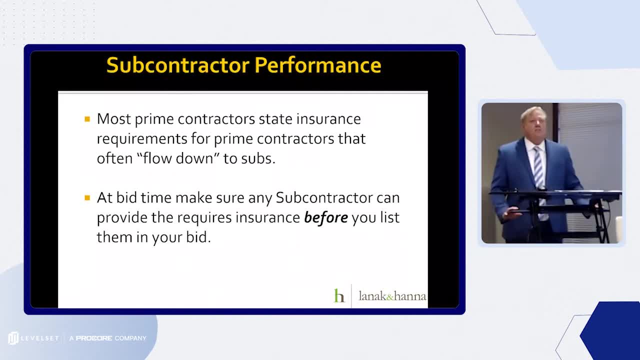 blatantly say that, oh, I'm going to add to my contract later. You're going to have to build it in, All right, next slide, All right. so this is the term flow down and it's more general than I've just stated here. but 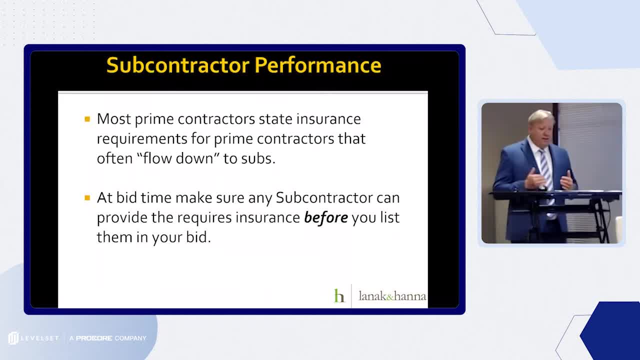 some- a lot of prime contracts and some subcontracts- say this term, which I don't really understand what it means, because I think it's very vague, And I think that if you, that if the clause is used, that if you're seeing a negotiation, you should try to negotiate it and get more specificity on it. But like 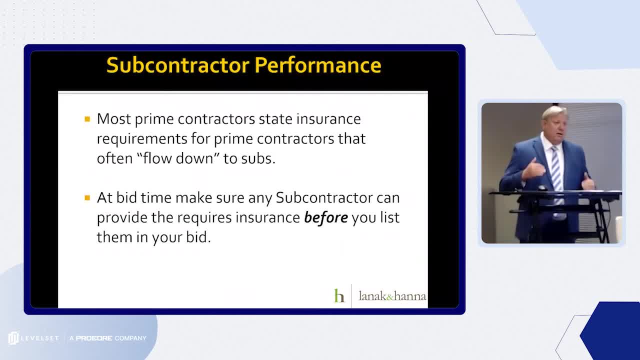 this one, this type. let me just say what the clause is I'm talking about. Many contracts say the prime contract flows down to the subs, as the prime contractor flows to the owner or worse, to that effect. Basically means that the terms of the prime 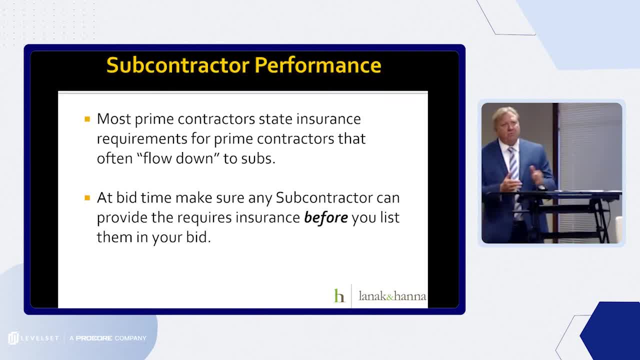 contract flow down to the subcontractors so they've got to perform as if the sub prime contract was part of the subcontract. Problem is that term flow down and there's terms that kind of mean the same thing. it's very hard to figure out exactly. 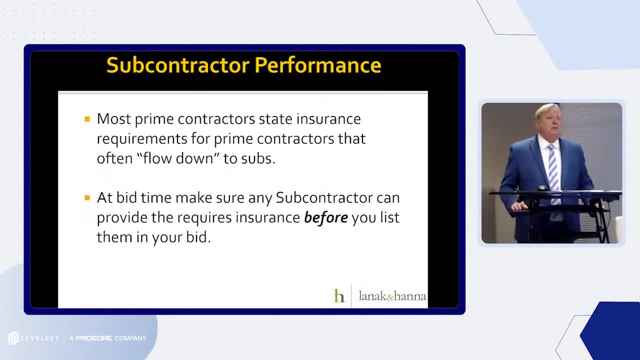 what is flowing down. So I would recommend that if you're talking about and you have the ability to negotiate this, you specifically identify what parts of a contract are in the subcontract. But I'll tell you if you go to court and you're going to argue about. 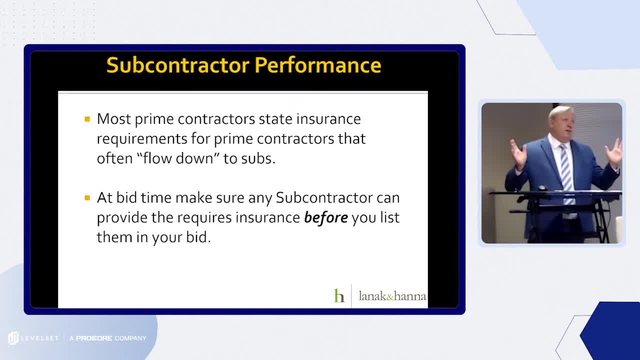 this. that clause- it flows down to the same extent it flows to the owner- is completely vague and meaningless. You've got to remember if you're in a court, you're talking to somebody who doesn't know anything about construction. so I'll tell you right now I'm going to 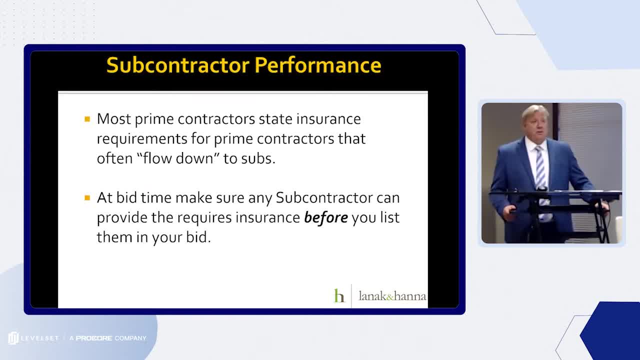 like I said, I'm in trial right now and doesn't know a thing about construction and frankly, it's like talking Greek. It's a whole different world that is very foreign to most people. So the way you try to make your contracts- and this is a general 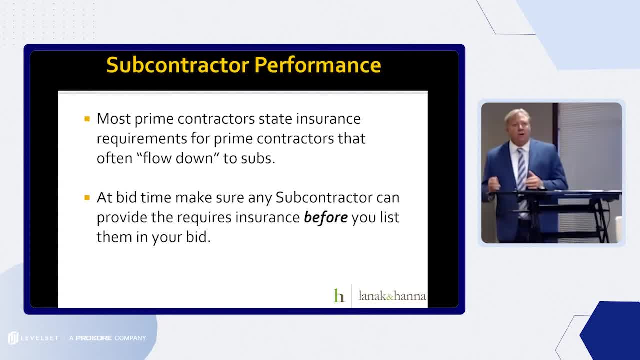 overriding concept. if you have the ability to negotiate or if you're drafting contracts, try to make it as clear as possible. Don't rely on hey, the subcontractor or that guy knows what I'm talking about, because ultimately, if you're in a dispute, 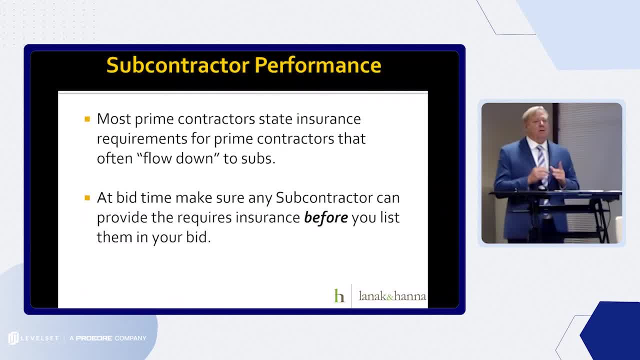 you're going to have to convince somebody that's not in the industry at all, so think about that Basically, make it so a layperson. I know that's a pain, but try to make it as simple as possible so that anyone can understand. 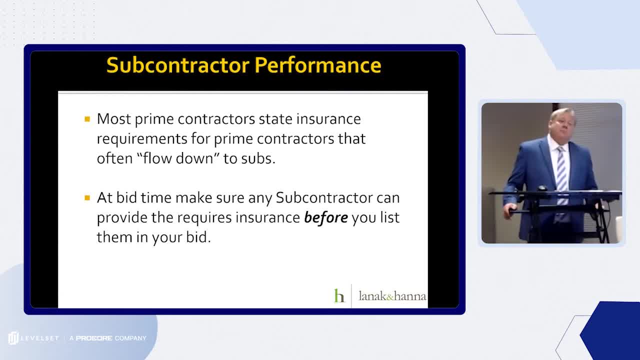 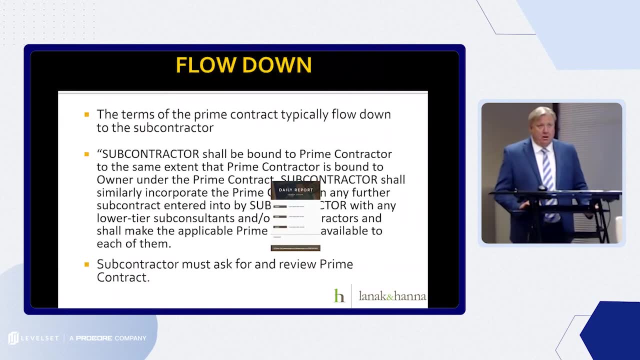 All right. so this is the last bullet point here is big time. make sure that the bonding requirements and the insurance requirements- your subcontractor can deal with them before you place them on your, include them in your bid. Blah, blah, blah. So 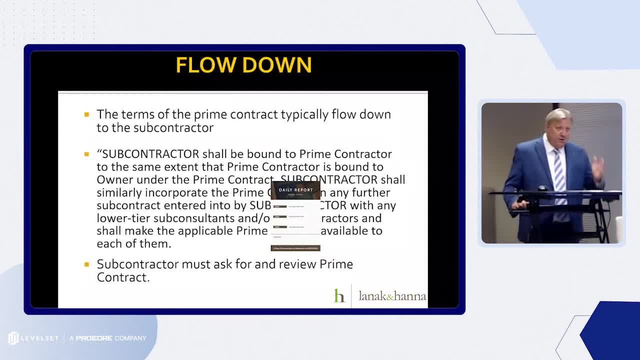 unfortunately I've got a little thing here in the middle of that clause, but here's basically the flowdown clause and the type I was mentioning. Like I said, if I could figure out how to get this thing out, I can. Now I'm in trouble. 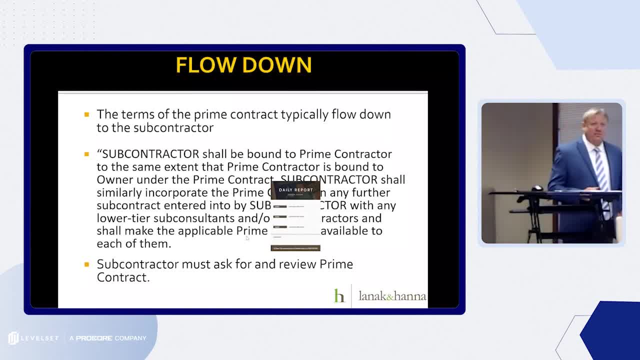 But anyways, my technical wizardry is on full display here. But that's the typical flowdown clause: Subcontractor. so we bound the prime contractor to the same extent the prime contractor is bound to owner under the prime contract. I frankly don't know what that. 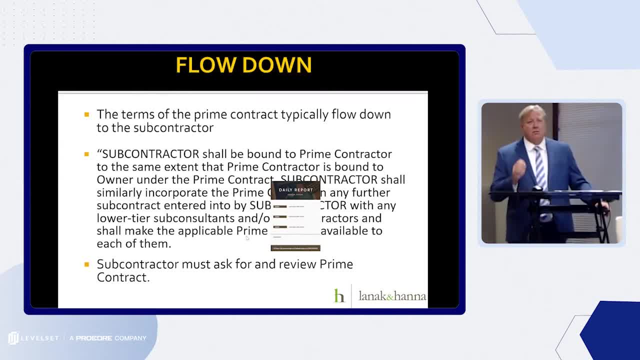 means, And I will tell you that I don't know what a judge means. So, the extent you can negotiate, try to nail down what that means. In other words, try to say: look, what parts of the prime contract are we responsible for? 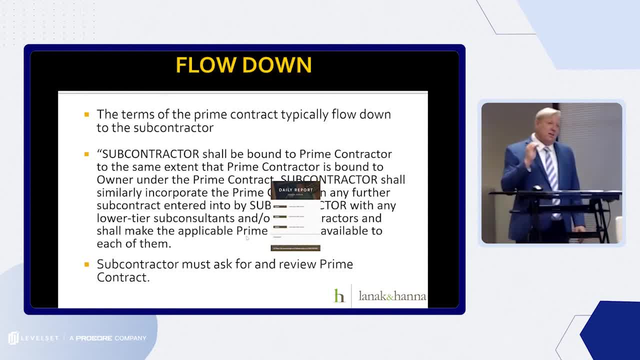 What parts of them flow down And then list those parts and say those are incorporated into the contract. This section here, about whatever that means, that first sentence, I think, is subject to interpretation and is vague. It's just to me it's. 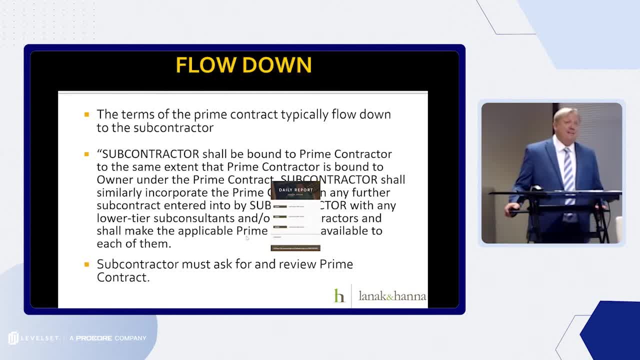 unfortunate. how many times that's in contracts and it's just not described. So I think that's something to be aware of when you're negotiating contracts. The last point, you know, seems kind of self-obvious, seems kind of intuitive. but if you're a 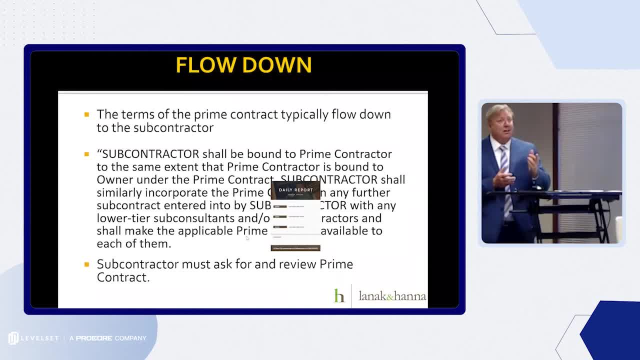 subcontractor and you're being asked to be bound to a prime contract. you need to see the prime contract. Lots of times in construction projects the sub never sees the prime contract. It's got a clause, like the slowdown clause, which a lot of them do. You need to. 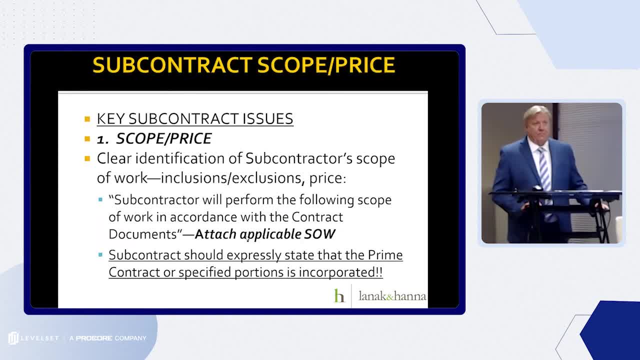 see the prime contract. All right, So on to subcontract key. we're on to key subcontract. We went to a whole other section. We're at key subcontract issues. So the first one obviously is scope and price. So if you are, 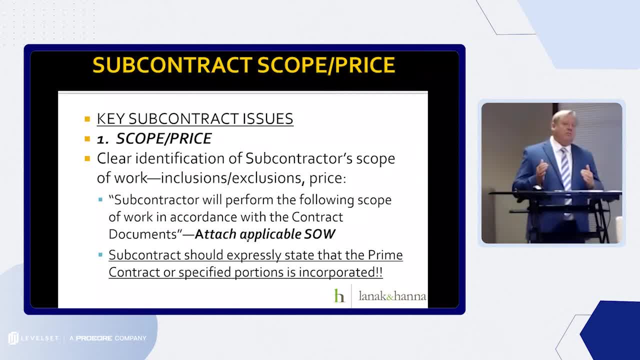 looking to make sure that, regardless of your general contractor or the subcontractor, make sure that what's going on here in terms of what the scope of work is and what's included or excluded in the price is clearly stated, Don't just say, for example, subcontractor. 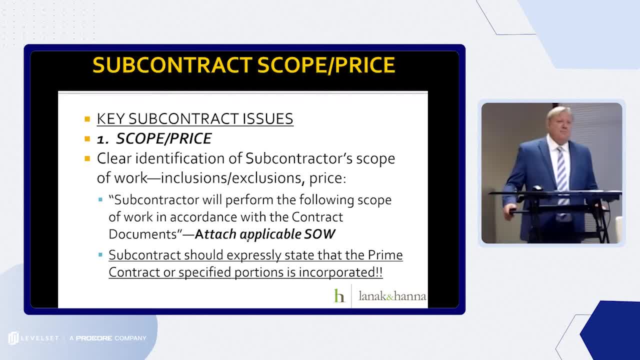 is going to do plumbing scope? That's too vague. Make sure you're saying subcontractor will inform the following scope of work in accordance with the contract documents And I would state, if possible, Subcontractor will do the plumbing work shown on sheets. you know: P1. 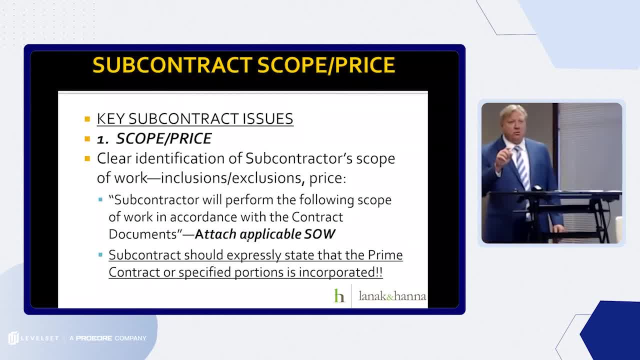 through 8.. Subcontractor will perform the plumbing specifications you know: 605 through 802.. They are attached here too. The key in all: you know: if you can make your contract as clear as possible, it's going to pay dividends in the long run. 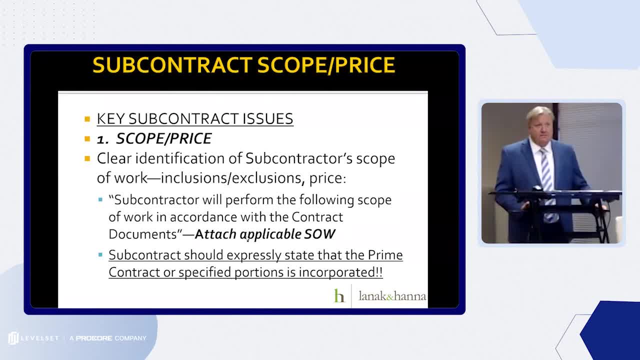 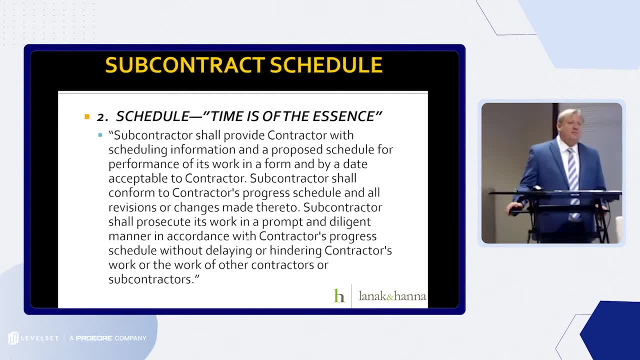 That's my final bullet point. I just covered it. So you know this is a big issue with construction projects. So schedule: obviously Subcontractor will provide contractor with scheduling information of proposed schedule or performance of a work and informant date. 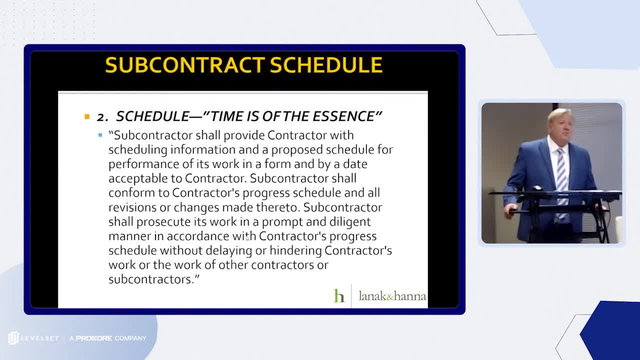 acceptable to contractor. Subcontractor- here's the one I probably should highlight. Subcontractor shall conform to contractor's project schedule and all revisions or changes made there to this project. That clause right- there is a clause I have litigated about, or similar ones. 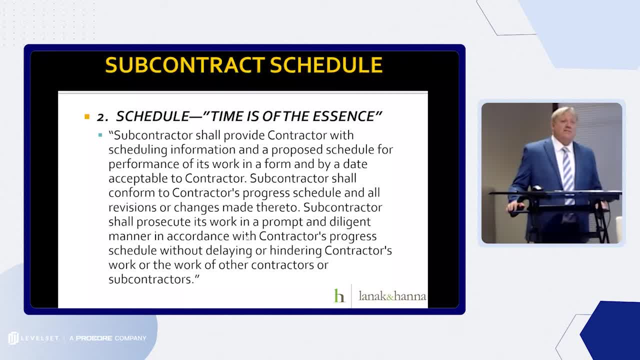 many times, And this gets into the situation: what is the contractor's schedule? and can the contractor just keep on changing the schedule and making jump through loops? The answer, in my opinion, is no, But the way, if you could, you. 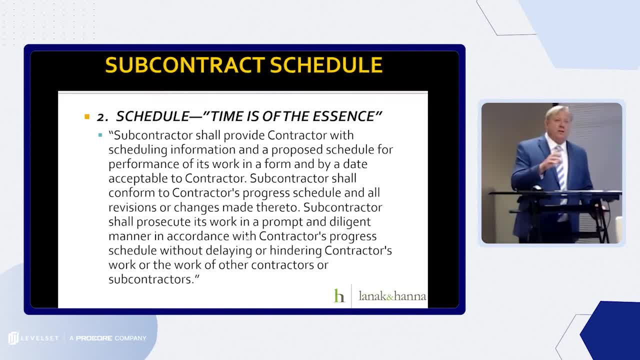 know, try to limit this to. you know, I'm only going to comply with the contract schedule attached to the contract at the time of bid, unless there's a change order or something like that. It's in your interest to do that. If you can't, then you're going to have to document. 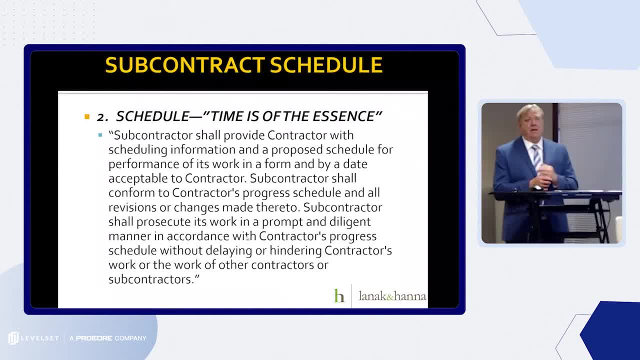 You have to document, document, document. You're going to have to document. hey, this is changing. This is changing my schedule. This is going to impact Your schedule is not accurate. Like I said, if you can try to limit, 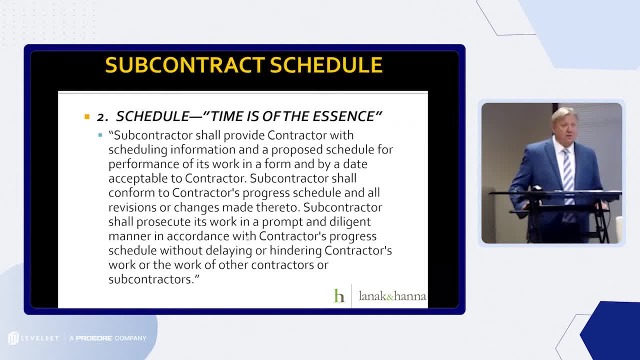 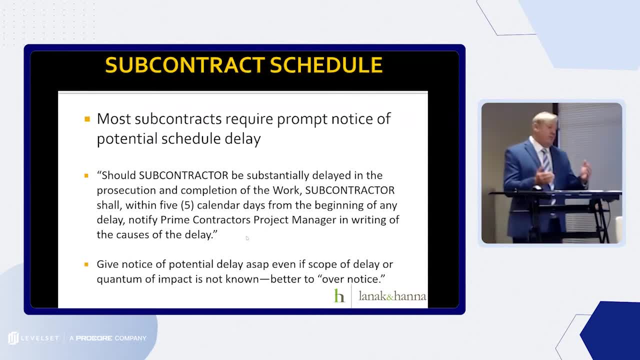 where you need to document during the project and make these things clear up front. it's going to pay dividends for you All right. So this gets into the next situation and ties into my document, document, document comment. So virtually all subcontracts are going to have 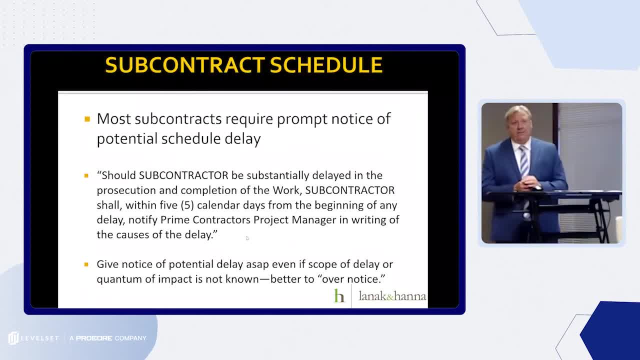 to accept revisions that say you're going to have to give prompt notice of schedule delay. You're going to have to give prompt notice of change conditions. You're going to have to give prompt notice of any condition you encounter that thinks you're going to have to seek extra compensation. 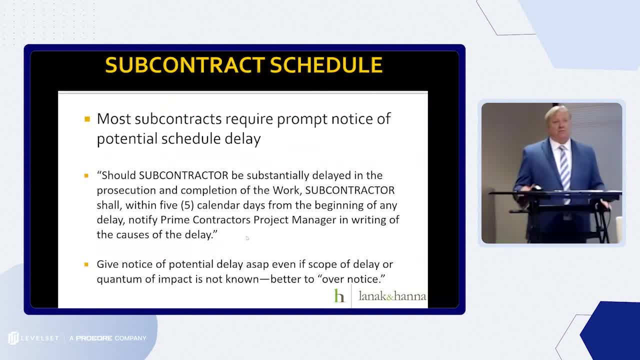 more money, or more dollars, or more time. So here's a substantial, similar, typical clause that's going to say that Should subcontractor be substantially delayed in the prosecution and completion of the work, subcontractor is shoveled in five calendar days from the beginning of the delay. 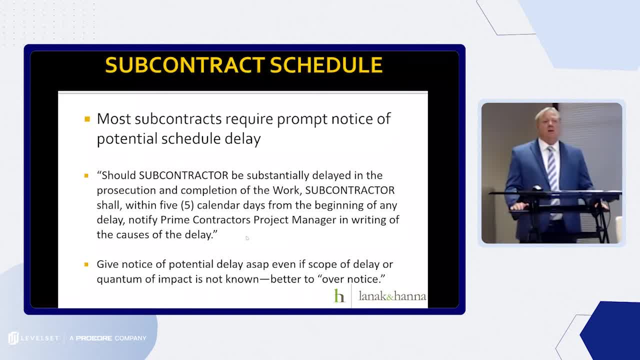 notify prime time contract manager of writing of the cause of delay. Last bullet: give notice of potential delay as soon as possible. even a scope of delay or quantum or cost of impact is not known. Better to over notice. You know one thing: that in my experience in litigation, 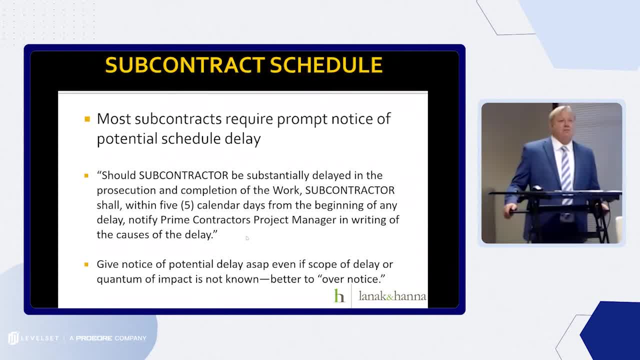 the big general contractors are much better at tapering the file than subcontractors are. They've got the resources to do it. when they've got people sitting back in there, off. hey sub, you're not doing this. hey sub, you're behind. 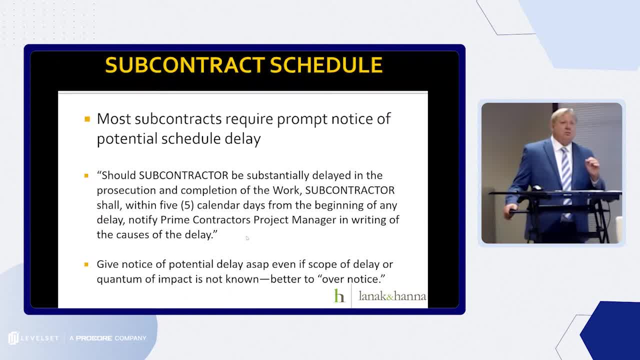 All this type of stuff. The extent that you can match them on that game or not a game, and that pruited course of conduct which would be correct about it, the better you're going to be going to be. so if you, if you come across something like my example way back when about you know we're 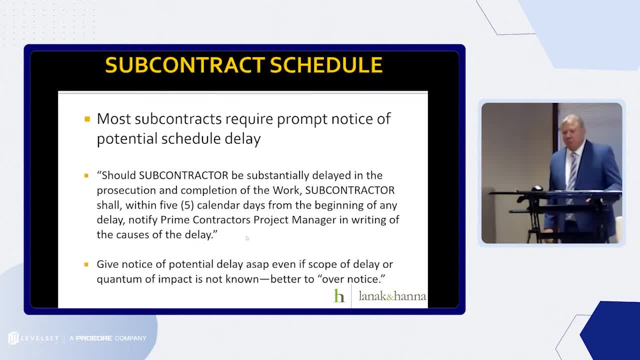 supposed to have sandy soil or regular soil and i'm having a bunch of boulders. when you hit those boulder, tell them: hey, we just hit boulder. that's a different site condition that is going to impact us. we are going to be delayed by this. we will identify later the quantum of that or the cost. 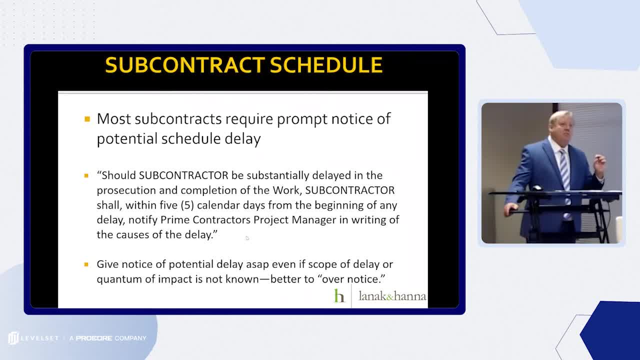 or the cost or the amount of the delay, but get your notice as soon as possible about that. hey, this is a problem. we are going to have an issue. try to meet this five calendar day thing as best you can. you know again, if you go to litigation, if you didn't do it in five days, can you get around? 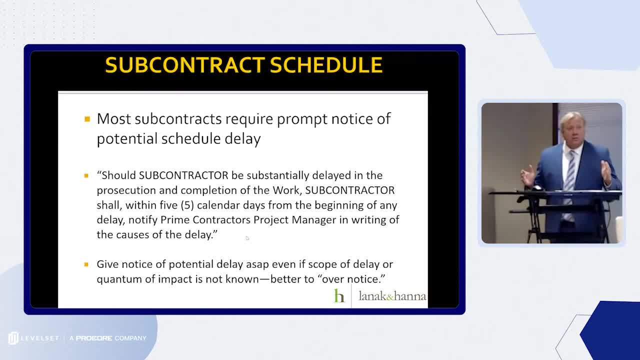 it probably, particularly if, hey, everybody knows that this was an issue i've told everybody. but don't, don't rely on you know, i told johnny when we're out, when we're out in the trailer about this. but very least send johnny an email saying: hey, johnny, i hit boulders. that's going to cause a delay. 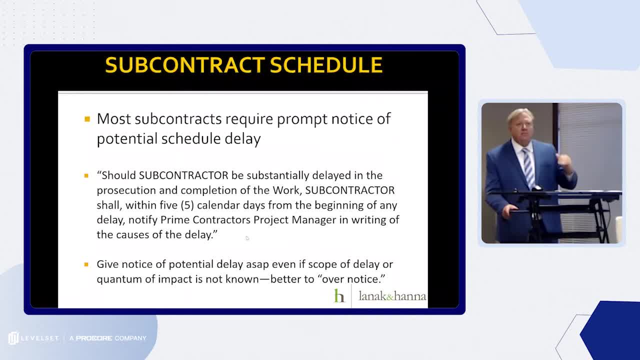 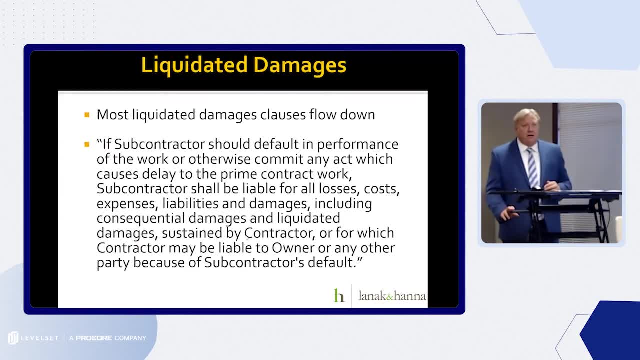 i'm figuring out how much. i won't know for sure until later, but it's definitely going to be a problem. all right. so we just talked about liquidated damages a while ago. they almost always slow down, so this is just a typical cause. so, like i said, if you can negotiate them out or if you can negotiate the limits on it, 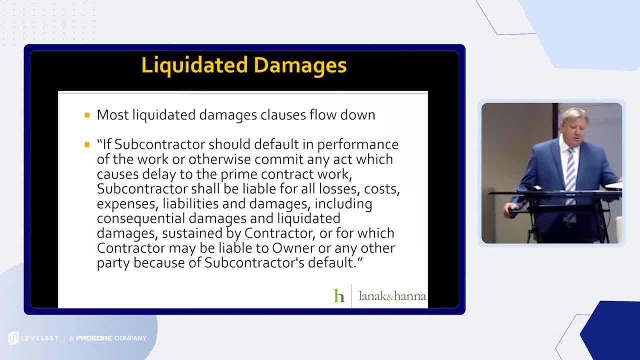 you know better off you're going to be. i don't know how you know whether you're going to be able to do that. it's going to be case specific. um, you know, obviously, even in the public works contest, in the public work context, while prime contracts are almost never negotiable, 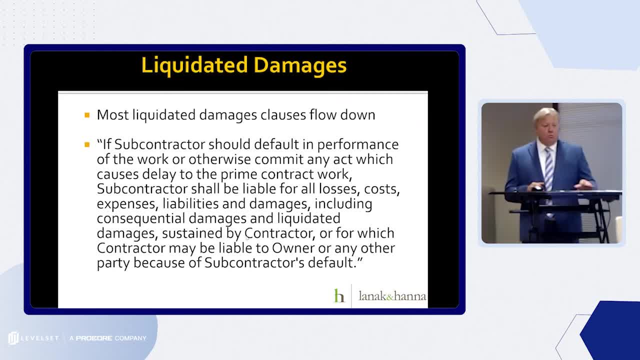 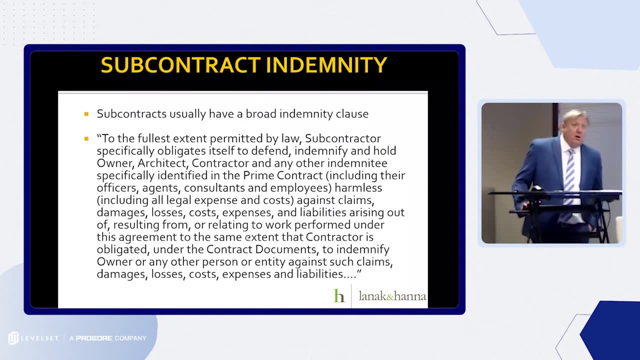 subs are not really subject to that. so there's probably is more room for a sub to negotiate, even on a even on a public works project, than than there is for a prime contract you're negotiating with public agency. another thing to be considered about is indemnity clauses. all- virtually every- subcontract is going. 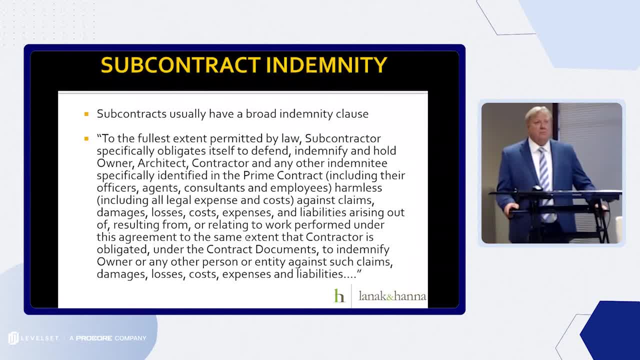 to have a huge broad indemnity clause. it's probably a similar one in the prime contract too, but basically says it just: you know we can read it. i don't need to read it, but it basically says: you're, you're on the hook for virtually everything, whatever goes wrong in that private. 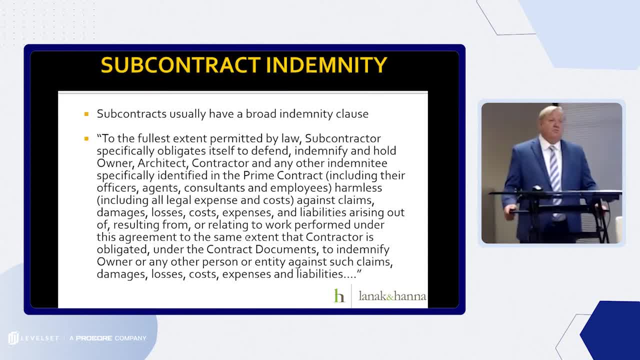 these clauses are designed to be a subcontract that's going to have a huge, broad indemnity clause to make it, so the general contractor can basically walk his hands of everything, say hey, there's a problem with your problem, so, um, so there are some limits by law. there are some. 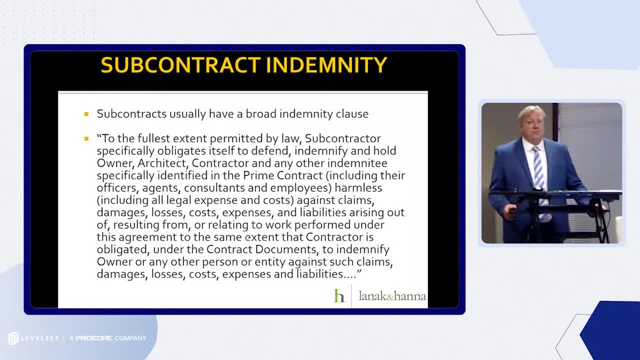 limits, ultimately that you're going to have to. uh, that you can assert, just in terms of going back to the concept of equity that we talked about early, but again, if you can try and negotiate these pause and limits, you're going to be better off. um, some of these clauses are so broad that 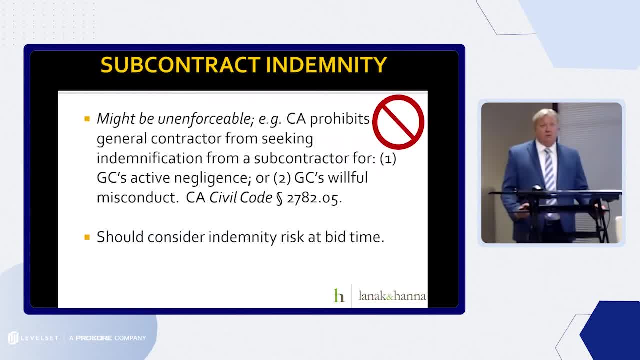 the law does help you out. so i think that's the next one. so some of these clauses are too broad, like, for example: um in california, you can't. you can't. um um, you can't. as general contractor, you cannot require a sub to identify, indemnify a general contractor for the general contractor's. 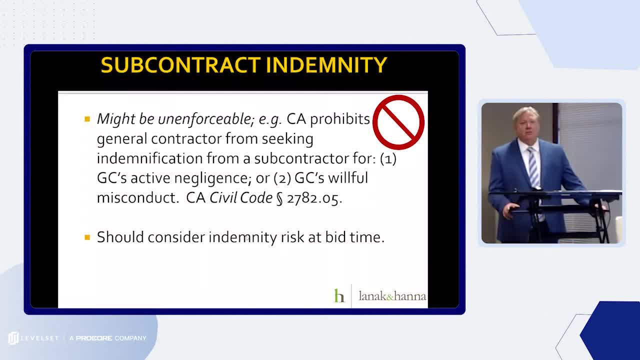 active negligence or willfulness conduct. i guess if there's other statutes in other states that would that would. that would provide that as well. you know some that it just depends again, if the equity concept does come into play, if you're going to go to the litigation on this. but you know it's going to be a problem and particularly it's going 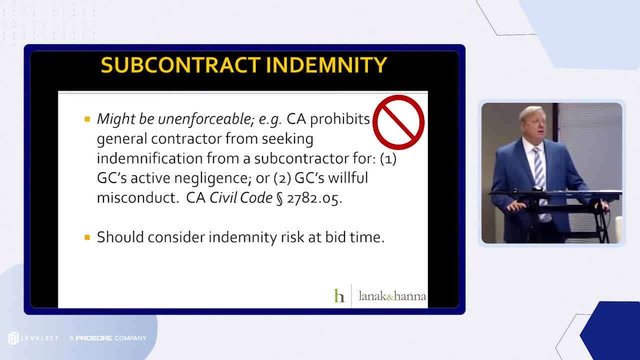 to be a problem in terms of the defense obligation. so how that would work is: let's just say, the gc gets sued by the owner for whatever delay or construction defect, anything. first thing they're going to do is they're going to send out notice to all their subcontractors and say, hey, we got this. 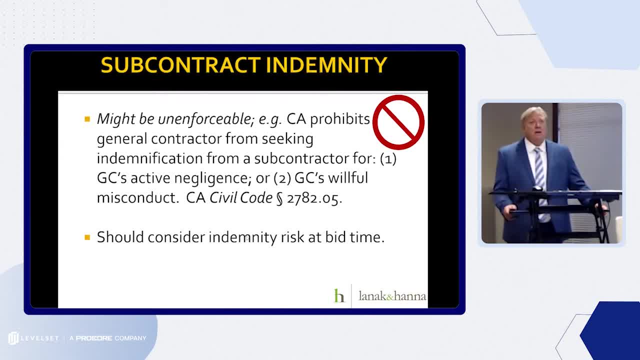 lawsuit or we got this claim. we're going to go to the defense and we're going to go to the defense. here's our, here's our demand: that you defend and indemnify. so defend again. you probably know this, but defend me. you're going to fight that thing and you're. 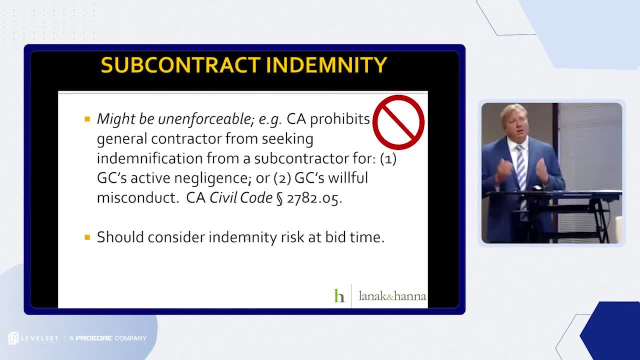 going to pay for my lawyers or you're going to bring in lawyers to fight it. for me, indemnity means hey, if i get hit with money or damages, you're going to pay the money. it's not me, you know. like i said, we can try to deal with this later, but you should try to. 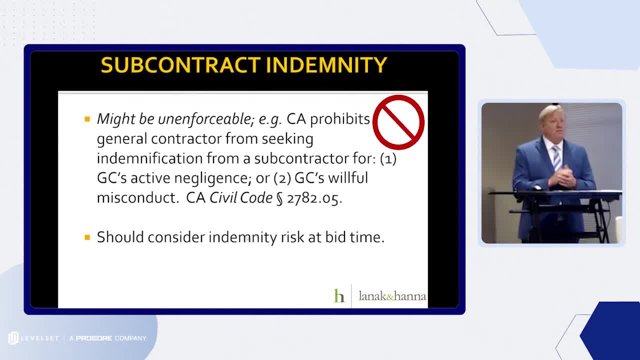 try to deal with it up front much better how they can. if you, if you either negotiate it out or definitely consider the indemnity risk when you make the bid and decide, hey, is this risk, the risk of problems on this project? am i really putting myself too far out by agreeing to this? 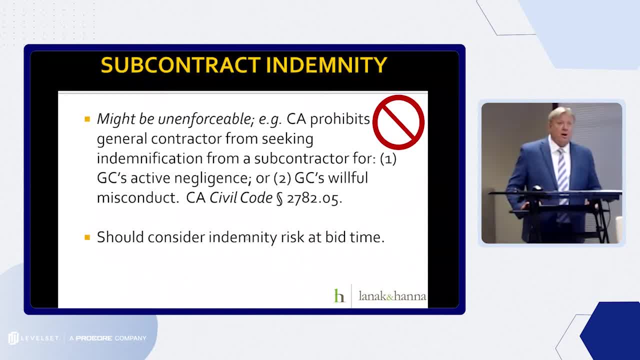 so, um, you know, bids are more than just what's the price, what's the scope. you got to consider a lot, of, a lot of things when you're making up, when you're making a bid, in order to make sure you're not not, you know, in a hole and in a problem later down the road. 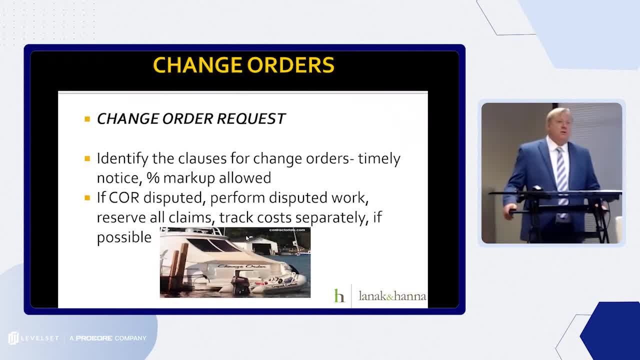 uh, so another one that's good, and you think of my or these change order request clauses? they're all going to have change over request things which are basic, very similar to very similar to what we just talked about. they're going to say: you know, if you you. 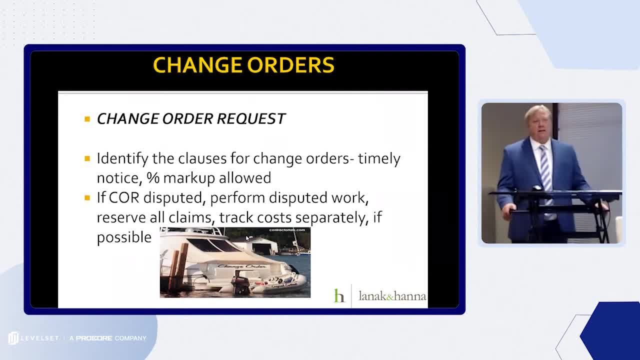 identified anything that that you think is a change, anything that you think requires more time or more money. you're going to have to notify the general contractor with a very short period of time. typically five days is really pretty common. the other thing to think about when you're looking at a change order, uh request, or a change order provision: 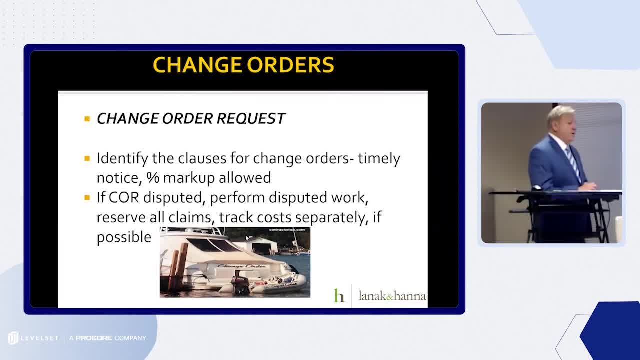 is. does it talk about markup? lots of these, lots of contracts limit markup. so your market. if you're trying to mark up a job, and you would typically mark it up 15 percent, hypothetically there may be a clause in that contract that says change order requests get marked up at five percent. 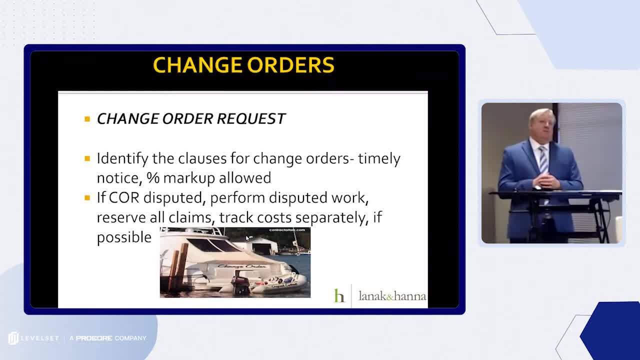 something about that nature. um, so you should take that into consideration again. if you can negotiate, it, great. if not, you got to think about it when you're making, when you make your bid. um, also, another clause to keep in mind is: um, virtually all contractors are going to say this. 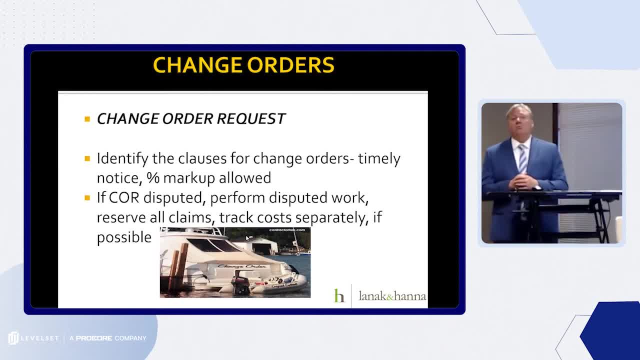 if a change order request is disputed, subcontractor will perform the disputed work right. so the last thing- and trust me this is i've dealt with this too many times- change order request because the contractor says he's not going to do it. that is going to be a 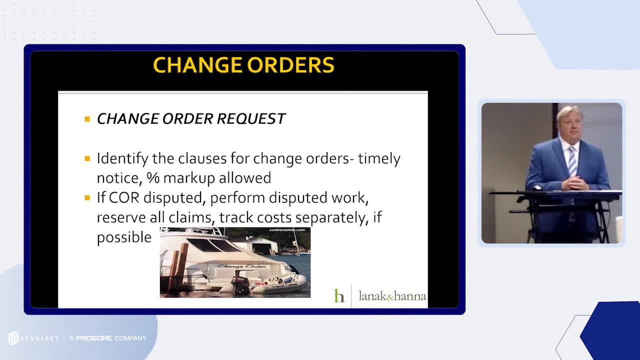 problem. that is going to be a huge problem. that is, particularly if you're dealing, if you happen to present this plane in a forum with experienced construction personnel. that's going to be a problem that is. that is very just, very uh, much disfavored to not do the work. um, and it can really 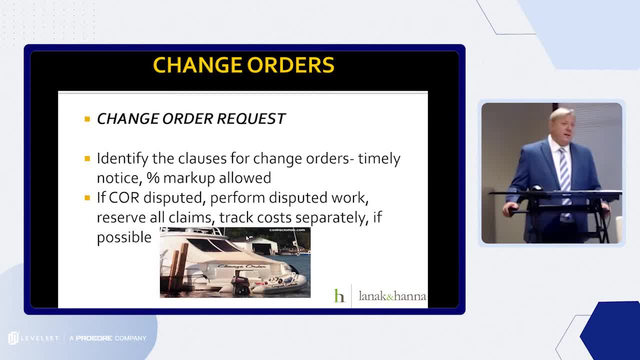 really cause big problems for you. so let's look for that clause. assume you're going to have to do it and do the work under protest. if you're in that spot, problem is that you went into on. this thing is document, document, document problem. a lot of subcontractors just say, oh well, i incurred a. 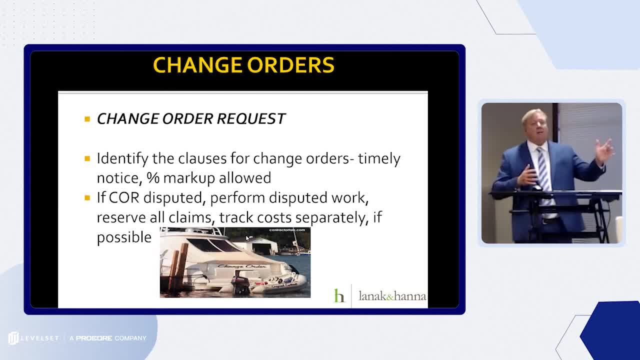 bunch more money on the project and some of it, or part of it, or a lot of it, do this change order not really going to be good enough. you're going to have to identify the specific work that was the change order work, and how much and why and how you included them. ultimately, you have to 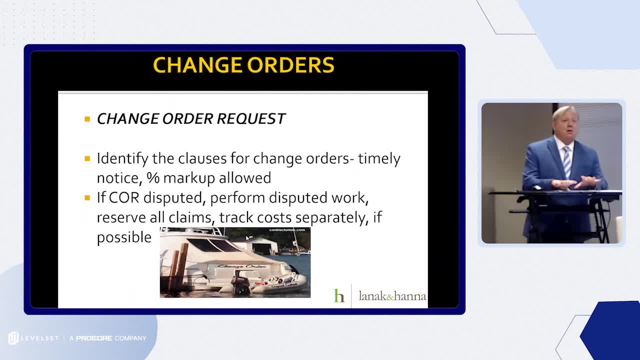 prove that your change order request, work was done for the change order and that the cost you incurred were reasonable for that. so you're going to dispute a word first. you reserve all claims. hey, we have encountered xyz problems. this is the change you have refused our change order. we. 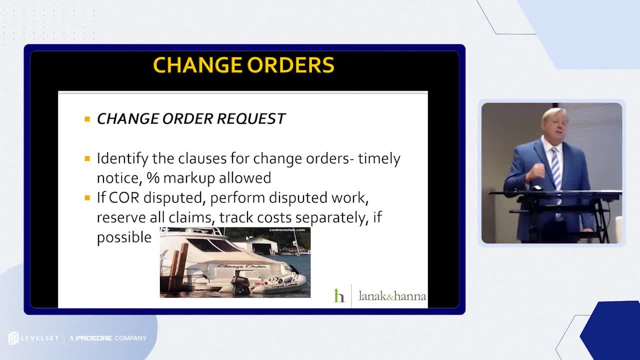 will perform this work under protest. we reserve all claims and then, to the best you can, try to track your costs separately for that change order work. i've even been on projects where if it's a big enough change or the contractor will actually put people with different 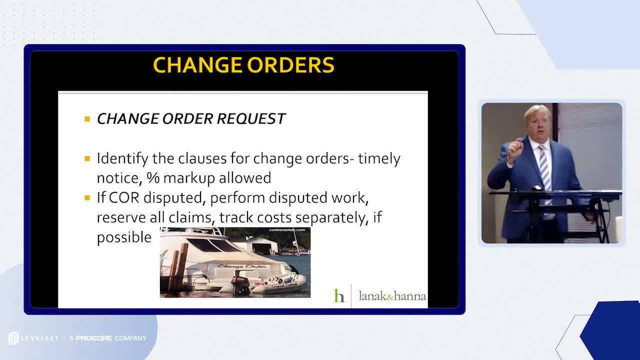 colored vests on the site and doing change order work and say all the guys in red vests are doing change order work and you track them separately. that's, the better you can separate out the cost, the better you're going to be in the long run if you have to fight about it. 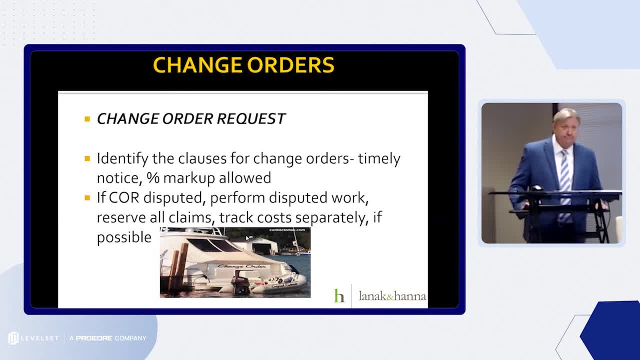 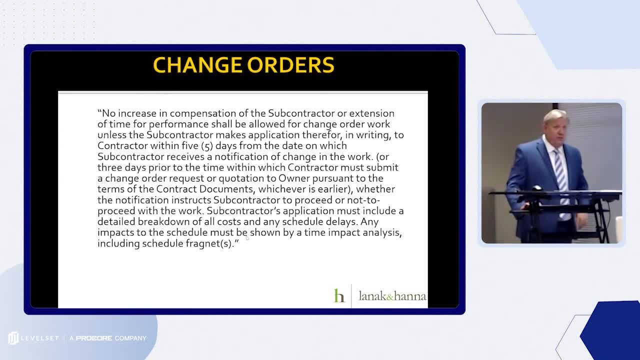 and probably are. we've already disputed your change order request. uh, all right, so here's. here's just another, basically a change order clause and giving notice of the clause five days, like i said, it seems to be the most popular five period of in these clauses, uh, but basically says: you don't give me notice and you don't get you know. 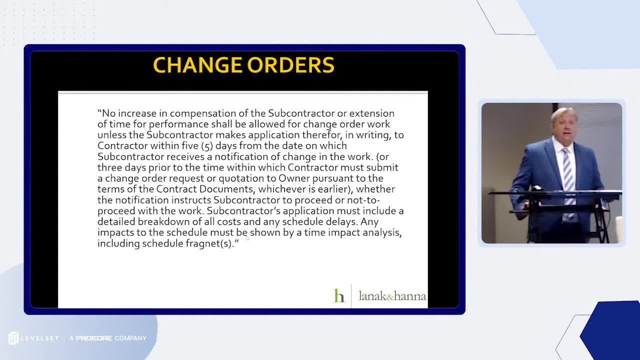 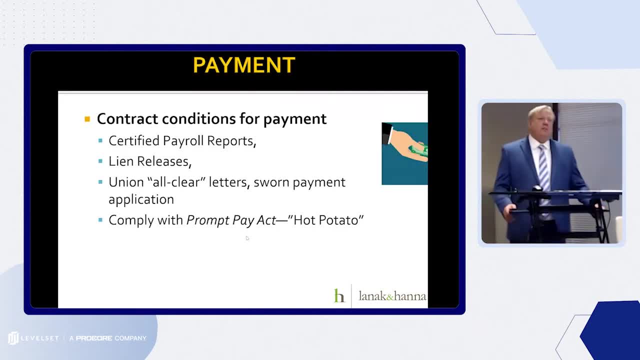 don't get blah blah blah, jump through xyz. you're not gonna get any money. you're not getting any time. all right, then let's talk about payment. let's talk about getting paid. look up the terms of what, what is required, what you're going to need to do to get money. if you're 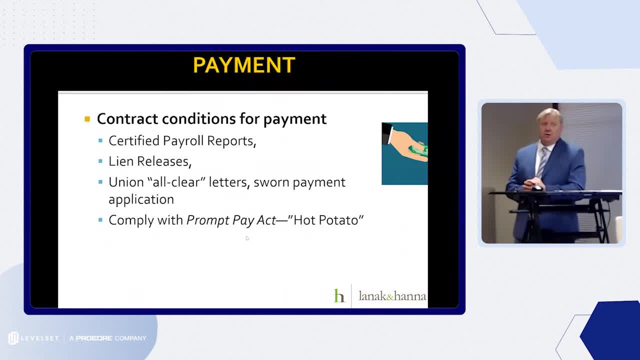 a sub. it's a public works project, a federal project. you're going to have to give certified payroll reports. you know they're required. i imagine a lot of states. they're certainly required in california. public projects are certainly required under the federal acquisition regulations on federal projects. certified payroll records are, you know, certified under penalty of perjury. 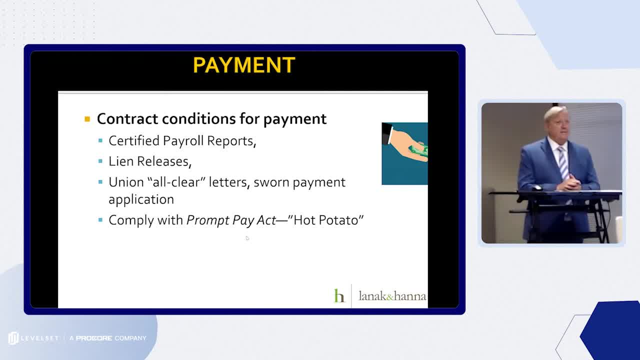 um, and they should be right, it should be accurate big problems that they're not including criminal prosecution. uh, and they are kind of. you know they're known as basically the bible in terms of what was the labor cost on a project. who did what? um, lean releases. this is basically: you're going to have to get lean. 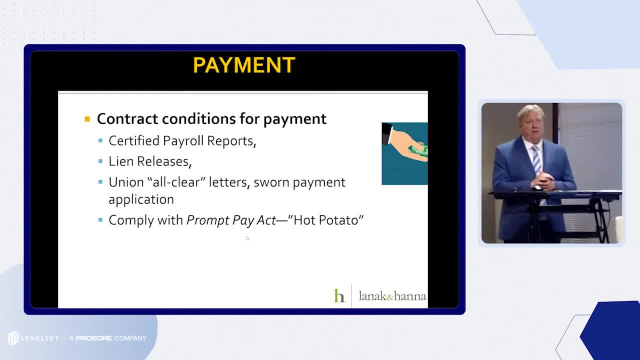 releases for your lower tier subs, your suppliers, on some of the dis-identified conditions that the contract is going to say: union, all clear letters, basically the letter from the union saying, if it's our union job, that you know, all union dues have been paid. blah, blah, blah. 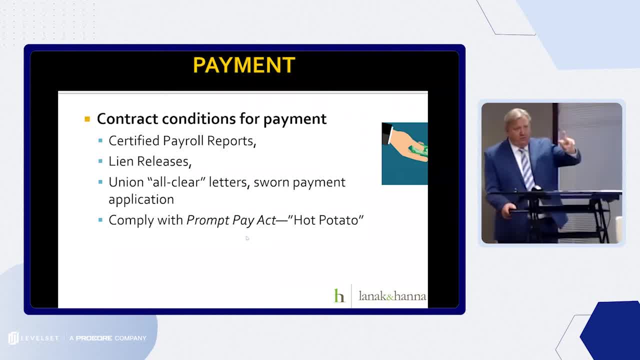 final thing to think about- so that's the first three bullets- were things that you're gonna that are probably in the contract that you're gonna have to apply with you before the GC has to pay you. The other thing to think about is look at the Prompt Pay Act. 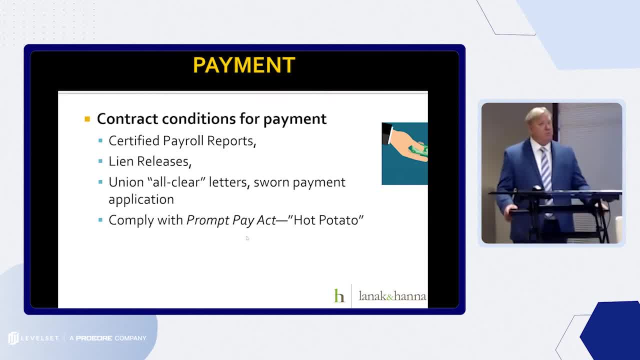 Prompt Pay. California has a statute that requires both public work and private work. that says if you get money for it, if the contractor or subcontractor gets money for the work of a lower tier summer supplier, they've got a certain amount of time to pay that person. 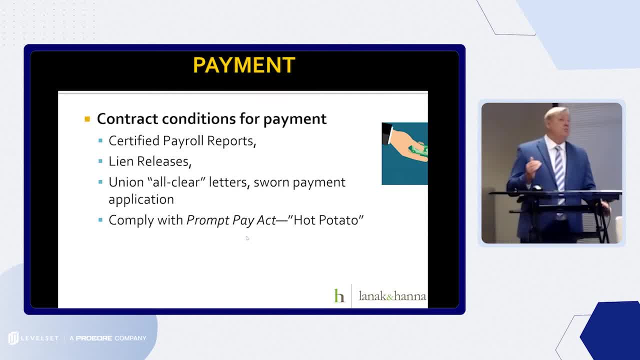 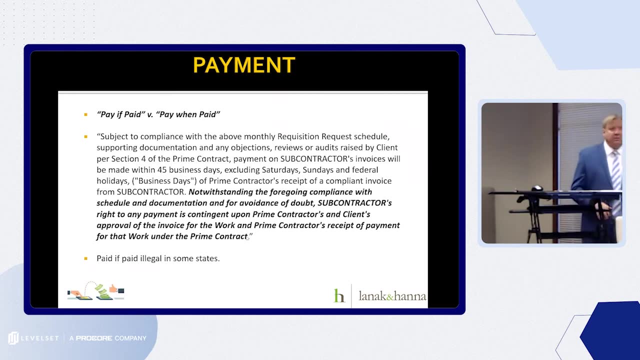 or they're going to be hit with penalties. California's 2% interest per month, which adds up quite quickly. So think about that when you're processing payment. where you are. All right, let's talk briefly. A lot of contracts have pay if paid, paid when paid, those types of things. 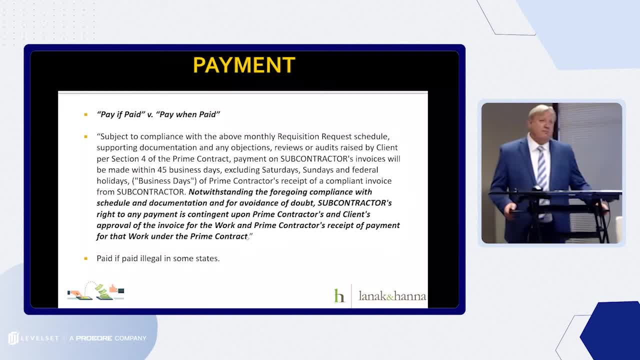 So pay if paid is illegal in some states. It's illegal in California. Pay when paid- Pay if paid, by the way, is legal in some states. I believe it's legal In Georgia. no, I'm sorry I may be wrong about that. It's legal in some states. Pay if paid is illegal in a lot of states. California is illegal. Pay when paid- That, I believe, is legal. It's legal in California. It's probably legal in most states, With the caveat that in California pay when paid means there's a reasonable period. 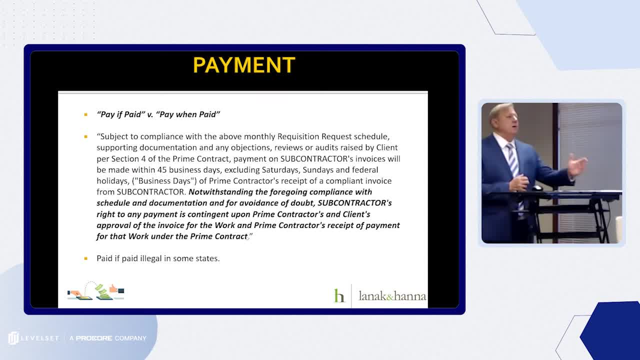 So in other words, yes, it's okay for the contractor to say, well, the GC will pay the sub. for the next days after the GC gets paid from the owner, There's a reasonable period when, if that doesn't happen, that the sub still has to pay the lower-tier sub. 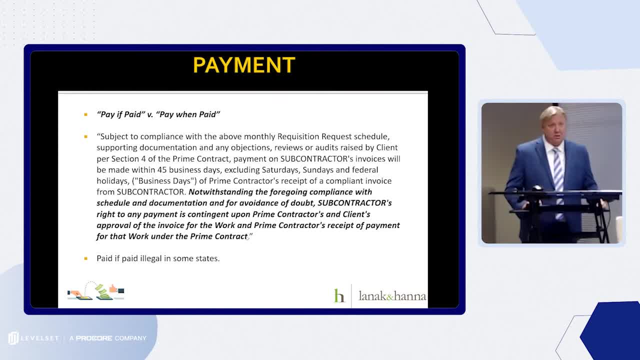 So, and like I said, I know California law much better than I obviously don't know many states' laws in California. Just something to look at, something to be aware of. All right, talking about payment, let's talk about how you get paid. 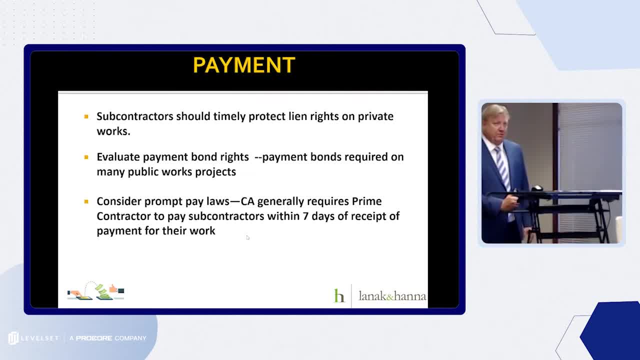 So let's talk about subcontractors and lien rights. You don't have lien rights on public works, but if you do have lien rights on private works, I'm sure pretty much in all of the states you do, California, you certainly do. 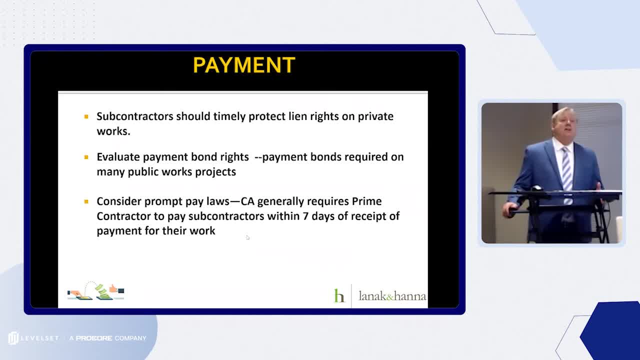 But in order to protect the process to have lien rights, you've got to step through the statutory requirements. The first one, being on a project, is you've got to give preliminary notice to the owner and general contractor. A lien is your ability, even though you're not in privity of contract. you don't have a contract with the owner. 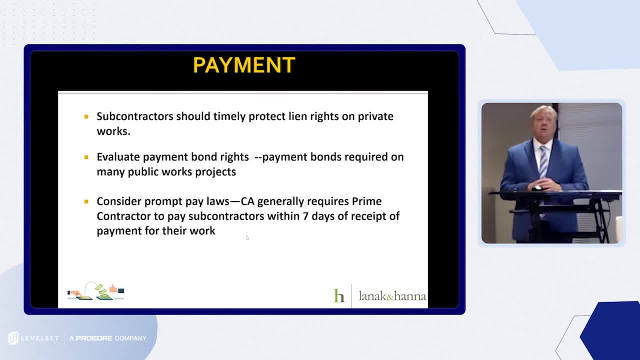 it gives you the right to pay the sub. You don't have the right to put a lien on the owner's property, but in order to do that you have to perfect that lien or under the terms of the statutes in your particular state. 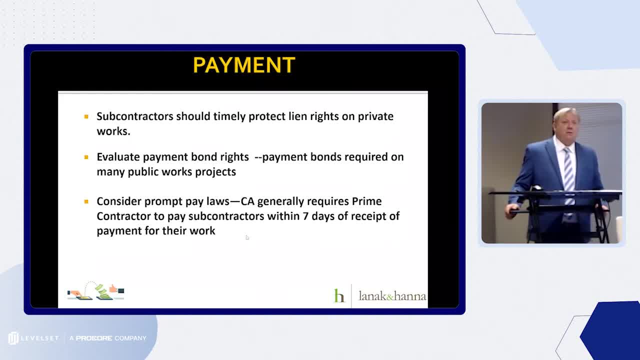 Again. we can have another discussion about all of these things for more than an hour, but generally you're going to have to within a very short period of time after going on the project. There's ways around this, but the prudent course is in California within 20 days of bringing stuff to the project. 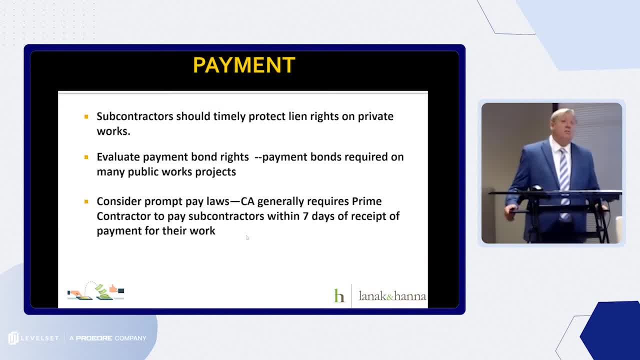 you get notice, a lien. you get to place a notice essentially on the appointment date or 28th or various names. but you want to give notice in accordance with the statute of your claim, the claim to lien rights on that property. 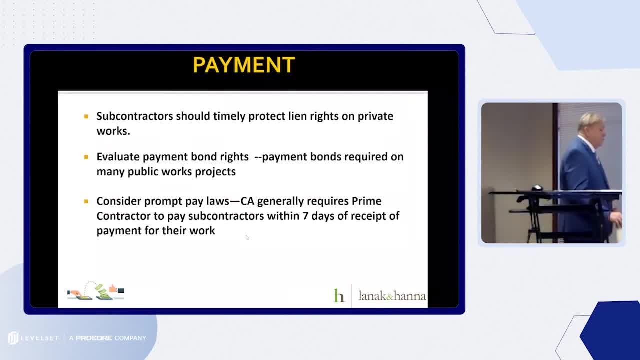 Some projects also have this. there are no lien rights in public works projects. Like I said, you obviously can't go placing a lien on the United States military base. You can't go place a lien on the White House. So public works contracts. 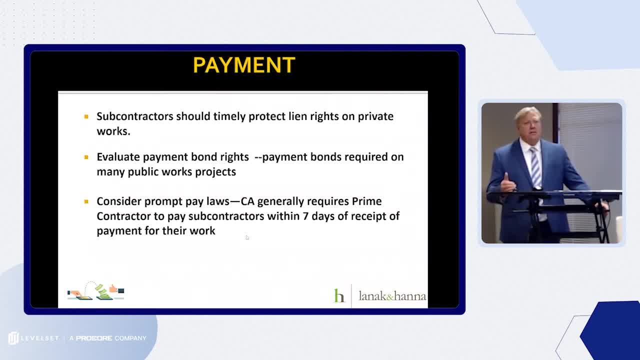 like i said in california, anything over 25 grand. i forget the cop and federal projects, but there's similar requirements there. they're gonna have to, they're gonna have a payment bond, and what a payment bond does is it basically gives you the takes the place of the lead. so if you're, if you, 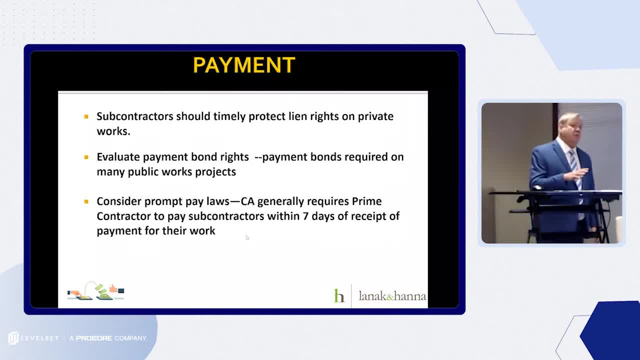 did not get paid on a timely basis by whoever owed you money- the dc or sub. if you're a lower tier subcontractor, the payment bond steps in and gives you the right to right to sue the bond company and the person that posted the bond- typically a dc or a higher piece here. so these things are very, very. 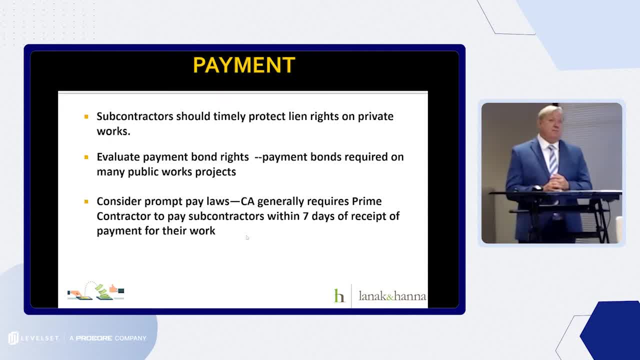 powerful in california, there is very limited defenses to obtain the bond claim. basically, if you brought, brought goods or services to a project and it was actually incorporated in that project and you're not paid within the contract time period, regardless of whether it's change order work in regards with disputed change order work, you may. 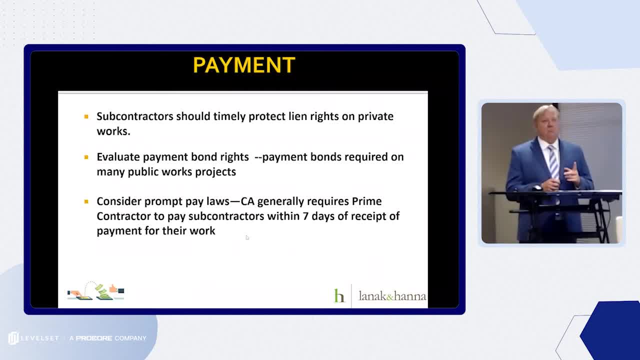 assert a payment bond, claim against the surety. it's a big hammer and it's, i think, in practice, underused. um, so, consider that, consider if you've got a payment bond, consider that you've got a hammer and consider whether to use it or not. uh, once again, i mentioned it briefly, but there's. 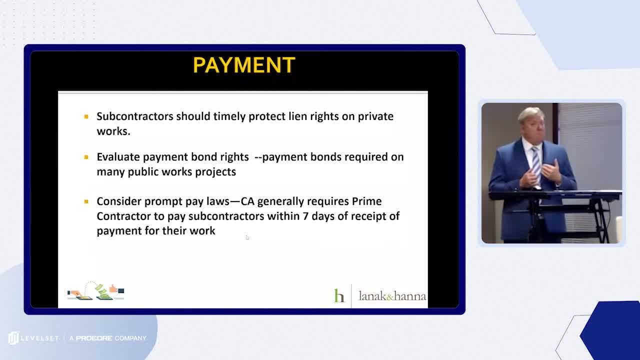 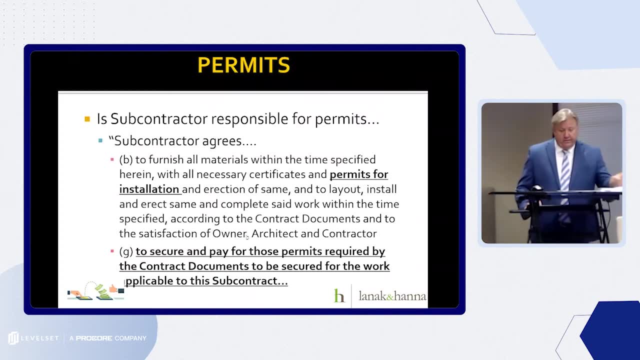 prompt pay logs. you got to think about if you're getting paid and you've got money that you got paid for a lower tier sub, you better think about whether or not you should be passing it on the seven days or whatever time period applies in your estate, otherwise you're gonna be sending some penalties. uh, or could be something? penalties, um. 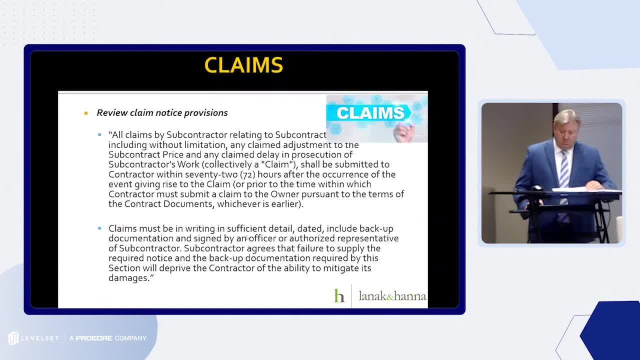 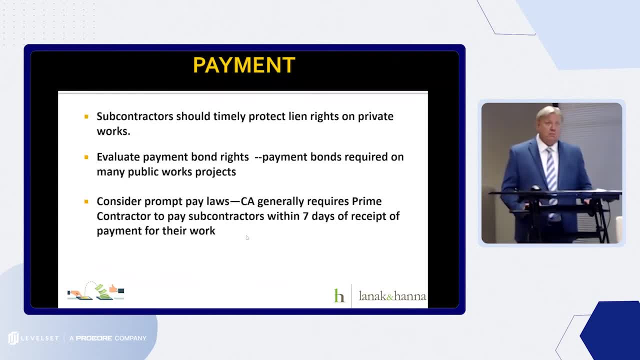 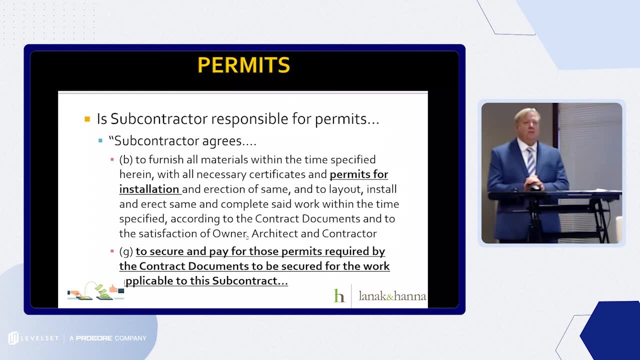 let's see where we are here. slow down. uh, this is just um, um. some more clauses to think about. when you're a subcontractor, a lot of times you know they get, so let's just figure out up front who's responsible for getting permits. um, typically that's a dc. 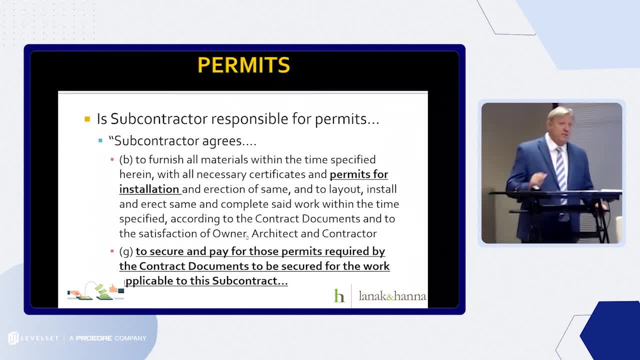 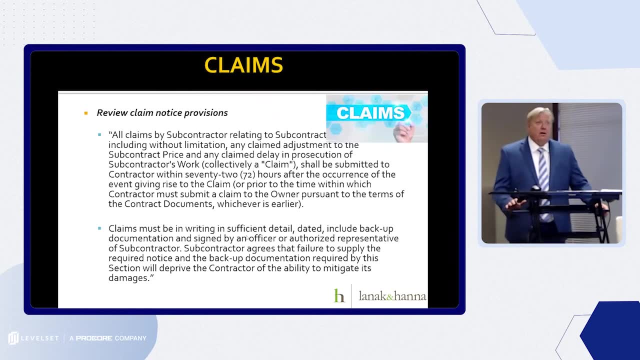 that's responsibility and you probably assume that if you're a subcontractor, watch out, some contracts do require the subcontractor to do that. again, if you can negotiate it out, great. if not, um, you know. back to the game when you're making your bid. uh, basically, you know what i've said about claims provisions. they notice provisions they apply to. 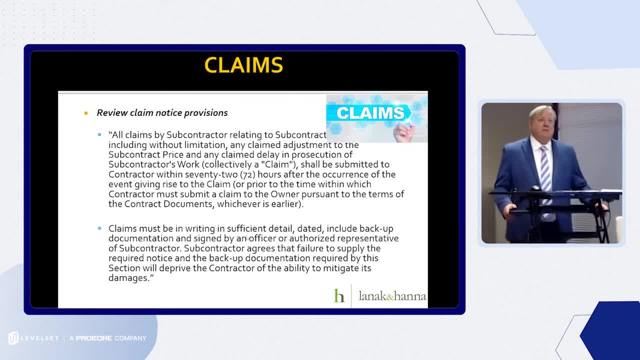 the prime contractor. they apply to the subcontractor, um, you got to be aware of them and and you got to try to comply with them as best you can like. i said giving what the contractor or owner would call the effective notice, because it doesn't state how much time or how much cost is involved in the 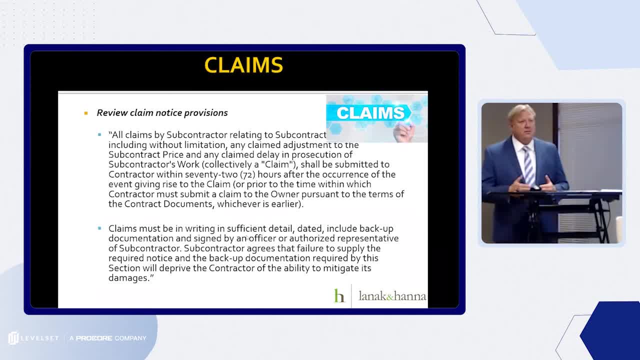 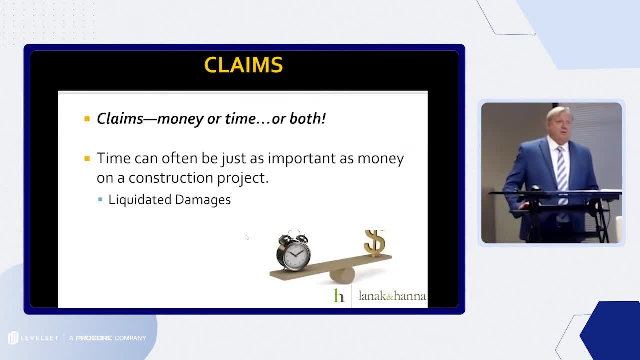 notice. giving a notice that doesn't provide those details, it's way better than no notice at all. that's, that's the key from my perspective. uh, so, yeah, so claims just probably everybody knows you got money, you got time or you got both, so you know, make sure you're covering when you're submitting a claim if you're. 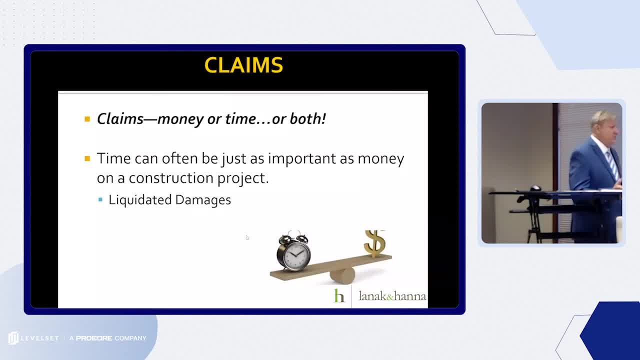 only asking for money. let's just say after that: if you submit a change order request, if you're, if you don't know how much time you want, don't submit a change order claim or a notice or anything that says: or change order request that says, hey, i want 25 bucks for. 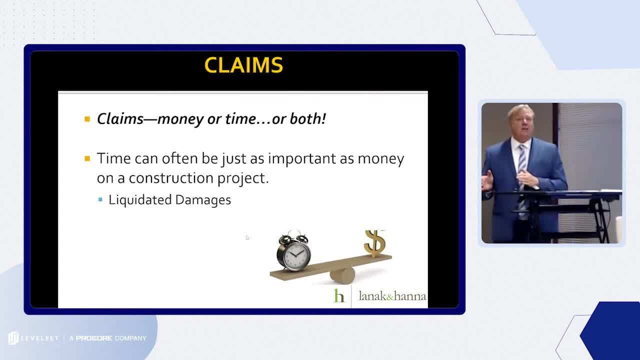 hitting that rock. if you're, don't say anything about time. there's gonna be an argument that you don't want time. so if you want time, if you don't know how much time, and you send a claim in, say i want 25 bucks- we are evaluating the time impact of this condition. we reserve our rights. 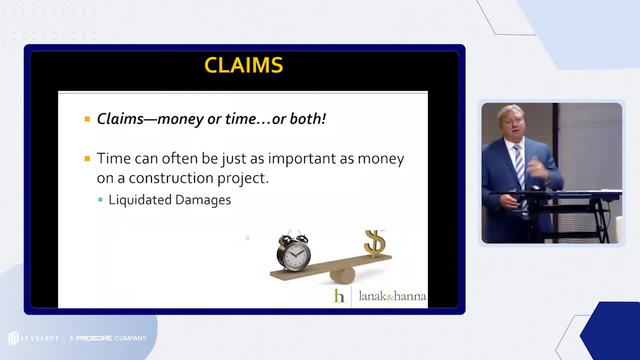 to a certain time. once that has been determined, you know, particularly if you're dealing with a contractor that's got liquidated damages or if you're dealing with a contractor that has gotten is. time is often just. this is important: preserving time and getting time extension. this is as important as getting money for the change condition. 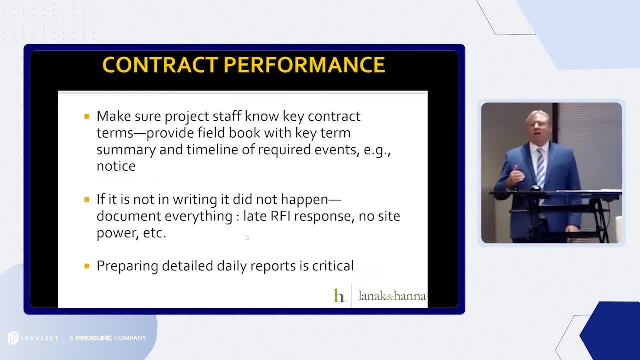 all right. so i can't tell you how many times i've gone to a project site and asked to ask for the project team. hey, what is the change order, uh, notice period on this project? when do you have to give notice of a different site condition, what's the contract, say? and they say i don't. 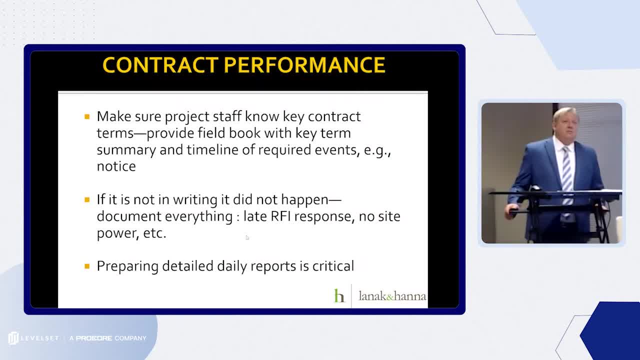 know i've never seen the contract, so so this contract performance tip is: you know the contracts they're all, unless it's a very simple project, most contracts are very detailed and very long and frankly, it's unrealistic to spend that. most project executives or project field teams. 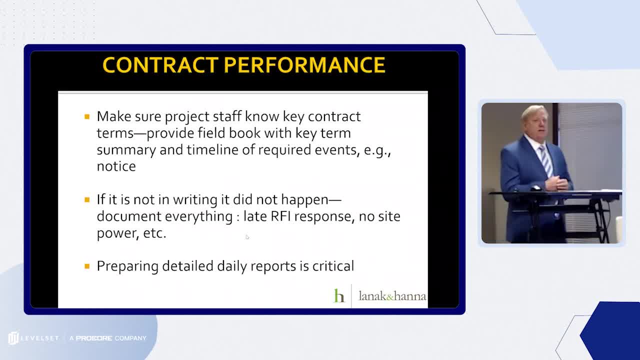 are going to read it. so try to shorten it down, try to give the highlights, as i say a little, a little bullet point that you can hand out to people that we should know. hey, here's our schedule. hey, if you encounter different site conditions, you've got you know. 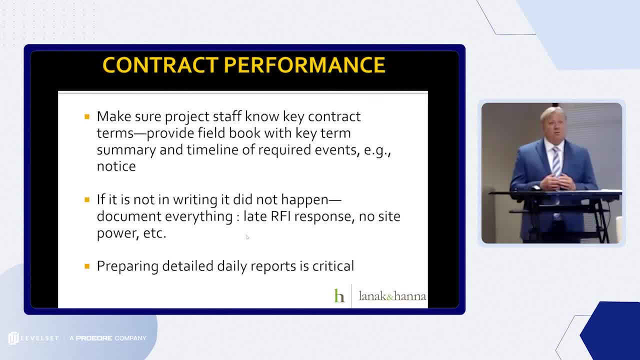 five days to tell people a little bullet point thing that everybody knows what to do. you know you can give that. um, you can, you know, make sure everybody's on board with what the contract says, at least the key provisions of the contract, and maybe make a little something they can. 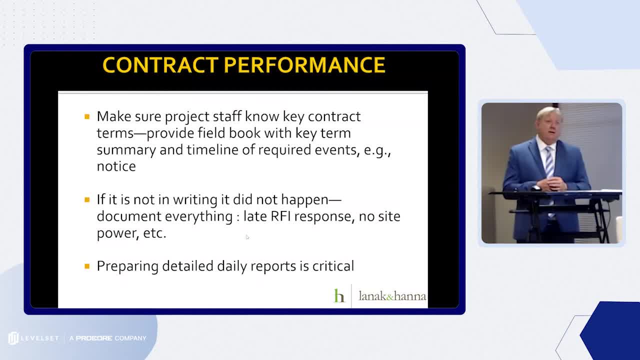 send out in the field so that everybody's on board with what to do. um, next bullet point in terms of contract performance. if it's not in writing, it didn't happen. you know the idea that, hey, i had lunch with johnny and i told him in the trailer or whatever, or over a beer that you know we 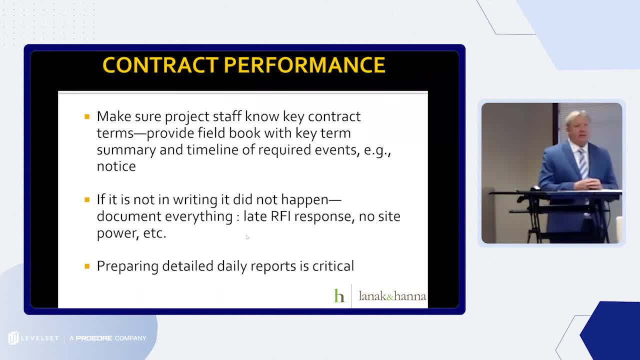 we're. you know we're having problems because we're getting delayed, because the electrical stuff's not doing x, y or z. put that in writing, um. make sure that everything is documented. if they're responding late to rfi, put that in the file. say hey, we're out here putting on our thumbs because you know. 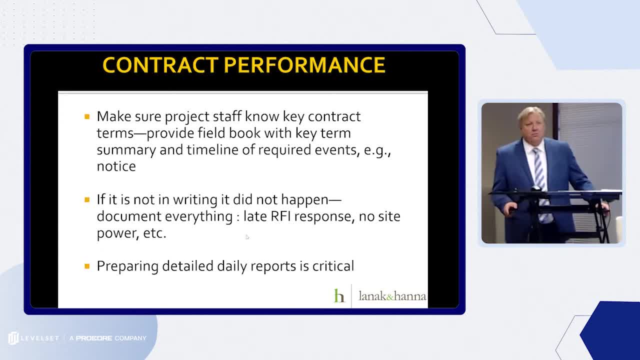 your dang architect won't respond to our rfi, got no site power. you know we can go on and on and on, But if it's not in writing, it didn't happen. Make sure you know. win the document game. Win the document game. 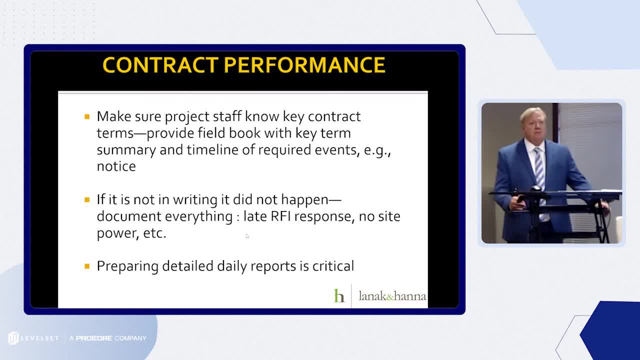 I know it's a pain. I know that a lot of subs don't have the staff to do it. To the extent it's very important, To the extent that you're going to, you know. in my view, you know, the best way to avoid being in a long-term or heavily litigated dispute is to assume up front that you have to be, that you will be the one and prepare yourself. 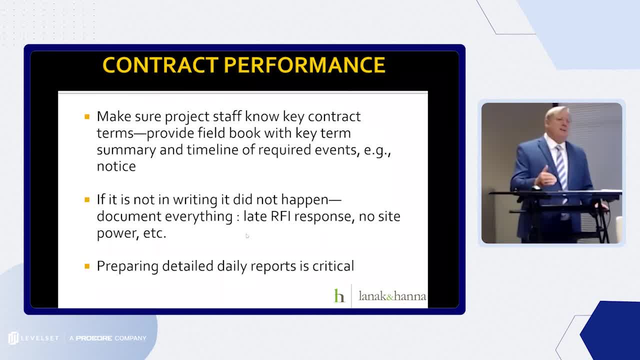 Kind of like a Boy Scout motto: right, Be prepared, or whatever it is. So same thing applies to contracts: The more you assume or the more you prepare to fight, the more you're going to be in a position to fight if you have to. 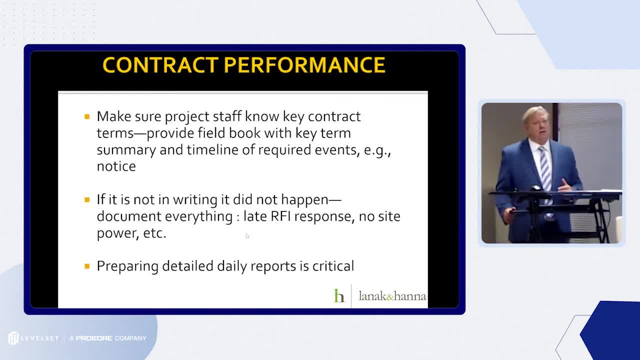 Daily reports are really critical. They're going to be- you know they're going to be used for or against you in the litigation. If you were to say: you know we couldn't do that work because we were delayed by the you know that drywall, it wouldn't hang the wouldn't hang the wouldn't hang the. 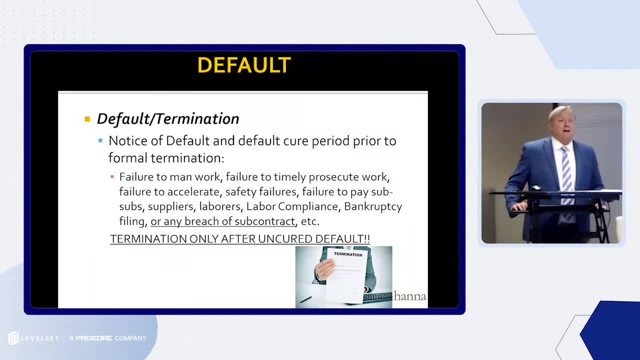 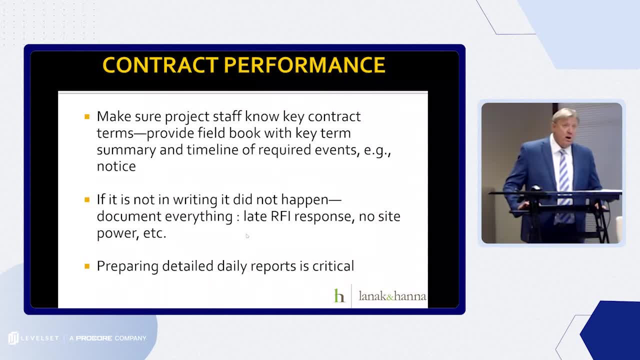 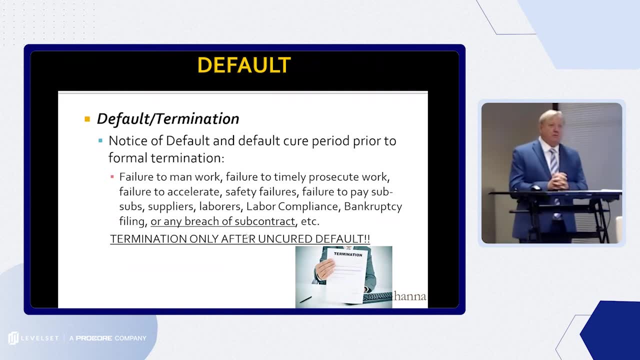 the sheetrock and so we couldn't paint the thing. You know, if there's not an explanation as to why you're not doing the work, then then that's going to be a problem. In writing. excuse me, Default default termination. you know, obviously nobody wants to hear about this, but that's the you know. this is. you know, if you deal with that situation, try to see if you can cure during the cure period. 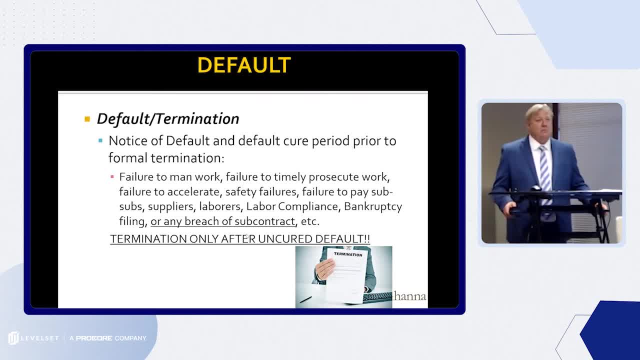 If not document why it's not, why it's not, Why you're not able to cure, why you're not- it's not a default- Why you're not able to cure the time period. There's not a ton more to say about that. 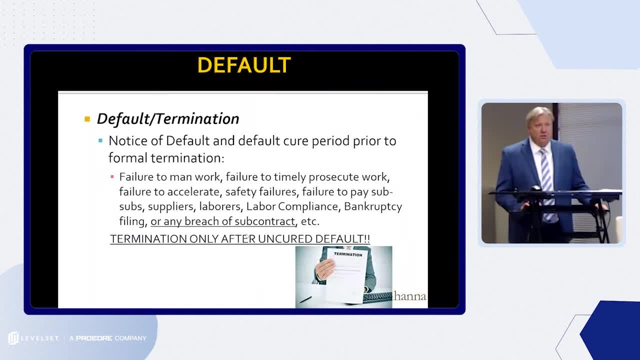 There's one thing I will add to that is the failure to man work So, or failure to prosecute work, if that's what the default is. if you dispute that, the level of work or manpower resources you're bringing to the site, that the contractor is putting you in default. 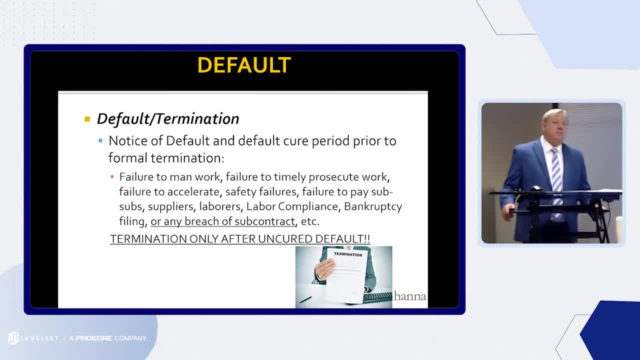 guns. you are below 1.5, attachment fee. what the contractor is saying is the resources required. The solution to that is to continue on site with the resources that you believe is adequate according to your schedule and your expectation of the work. 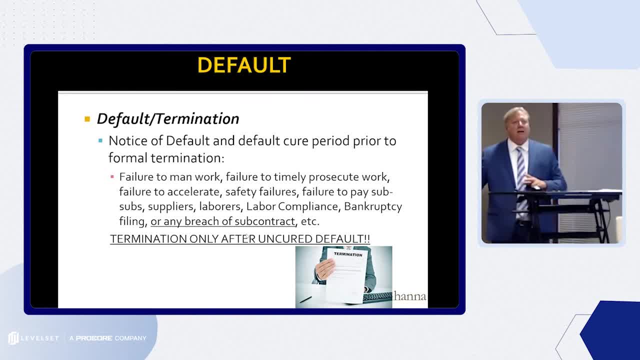 The solution to that is not to say I'm not going to man up, I'm not going to do that. You don't have to man up to what the general contractor asks for, necessarily if you believe it's excessive, But you should keep resources on site that meets what you can arguably say is your foreseeable requirements at the time. 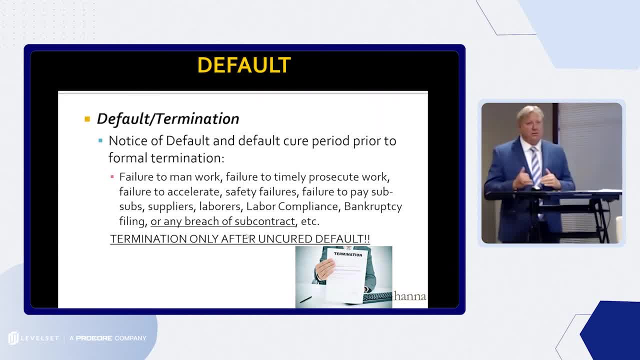 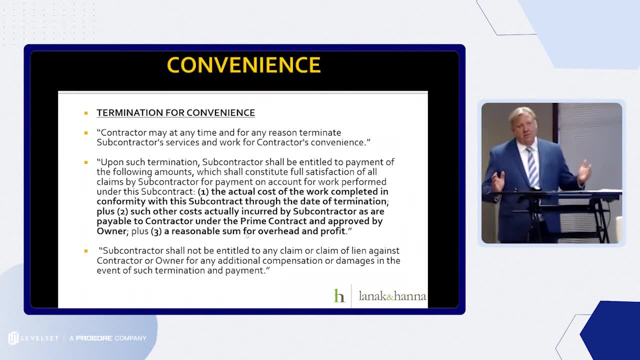 Because that's like I said, the worst thing to do is to leave the job and not perform the work. Termination of inconvenience: A lot of contracts have these. Just be aware, when you're bidding your projects, whether or not what the terminations are for convenience are. 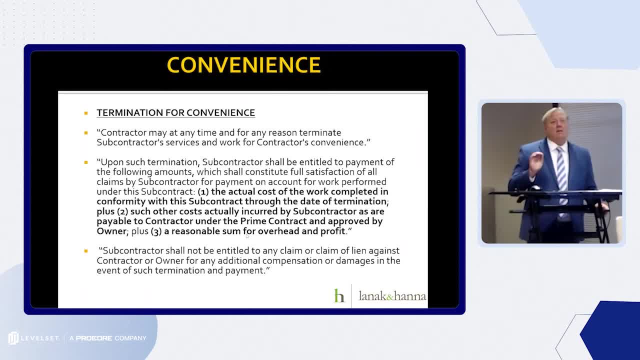 for them. It's pretty easy for someone to terminate for inconvenience. The thing that's critical is the highlighted portion below, which is what you get if there is a termination for convenience. This one has a reasonable sum for overhead and profit. That's fairly typical. 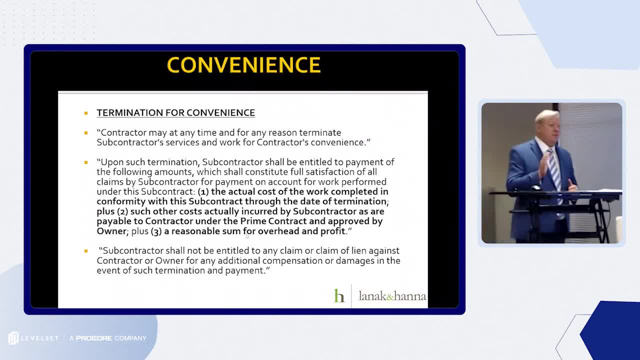 What this clause is doing is: it's taking away the right to get profit for completion of the work. So just bear that. when you're negotiating a contract bidding order, Look at what the default for bidding It says. look at the cure periods. Look at if they can terminate for convenience and what you get if that happens. 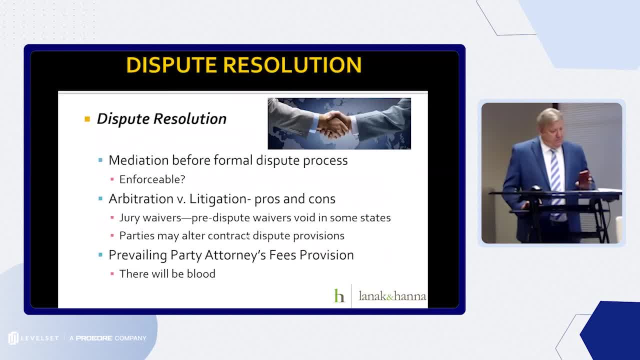 All right, All right. I think we're getting close here to the end and I'll just be obviously just be resolution to be, you know, maybe a day that the situation here, So let's just go through it quickly. So a lot of times it's become kind of a norm. 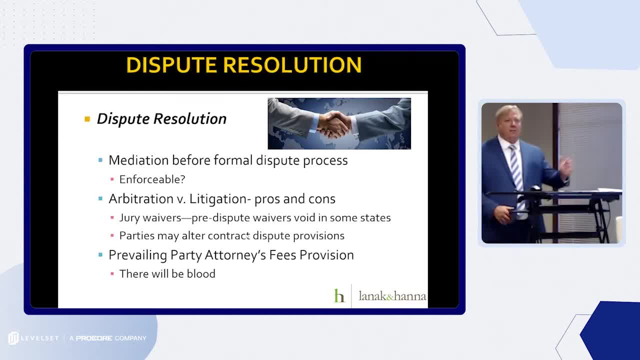 It's a new thing to do that A lot of contracts have a clause that says, before We engage in arbitration or litigation, the parties will attempt, with a good faith effort, to mediate the dispute. So my next question: is: that enforceable? 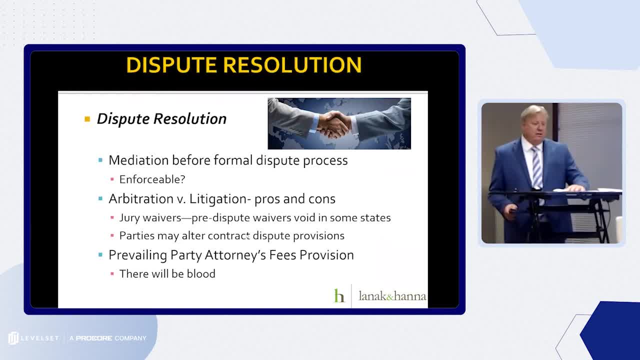 And the question is: if you don't mediate, is a judge or an arbitrator going to say you can't go to arbitration because you've got to go to mediation? My view on that is: maybe, maybe not. It's very judge dependent, hard to get. 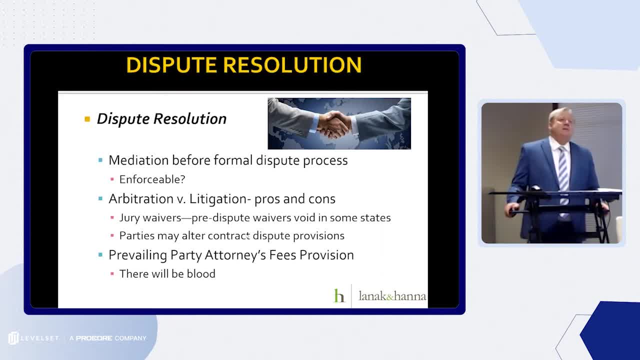 But the reality is- And let's talk about this- Mediation in general, mediation before formal dispute process. It's a great goal, It's a great concept. I have no problem with the thought. The reality is is that mediation only work if both parties are willing to accept some degree of compromise. 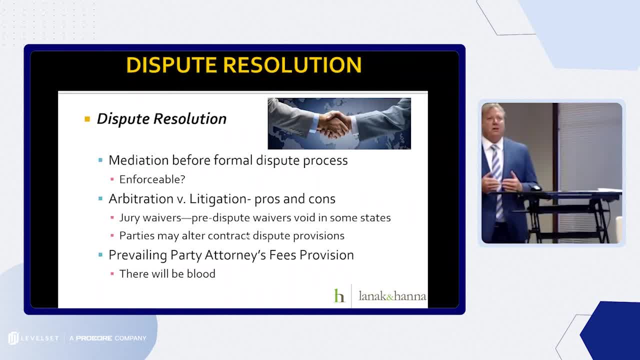 Can't go into mediation or any settlement negotiation and expect you're going to get hundreds of dollars while the other side give you hundreds of dollars. In contrast, if you are the party that's being asked to pay money, can't go when they're expecting this. 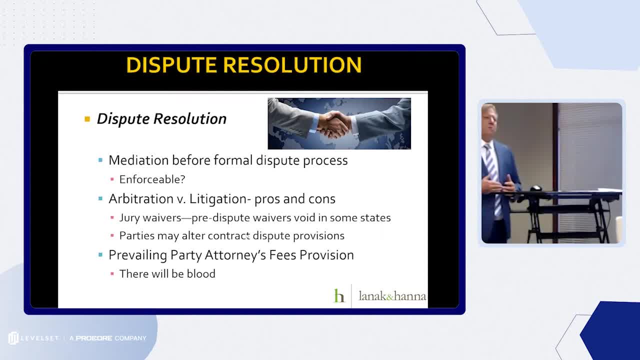 Have The Guys say, oh yeah, I'll take zero. You're right, buddy, Not going to work. There's usually a compromise needs to happen And sometimes that compromise people aren't in a situation where they're ready to compromise early on in the project. 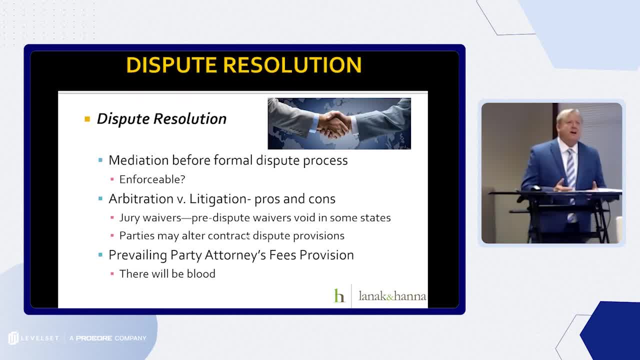 They need more documents, They need more facts, They need more, practically, the hassle of being in litigation to make them in the right mood to to solve the situation. So there are a lot of them go. Are they enforceable? I don't know. 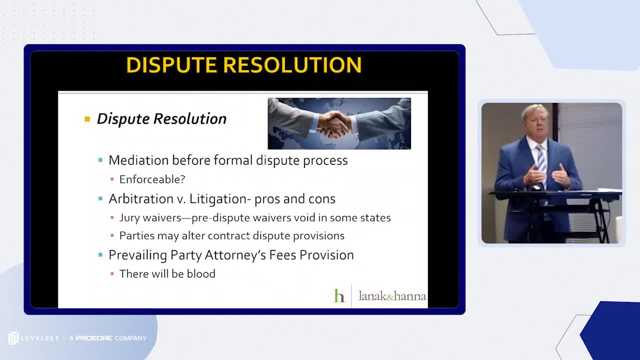 I'm not saying they're not a good, they're not a good thought process. I'm just saying sometimes they're effective, sometimes they're not. Next thing is arbitration versus mediation. I've done them both ways, Lots of ways. I'll tell you. the one thing I would say is that arbitration or a bench trial is is significantly preferable to a jury. 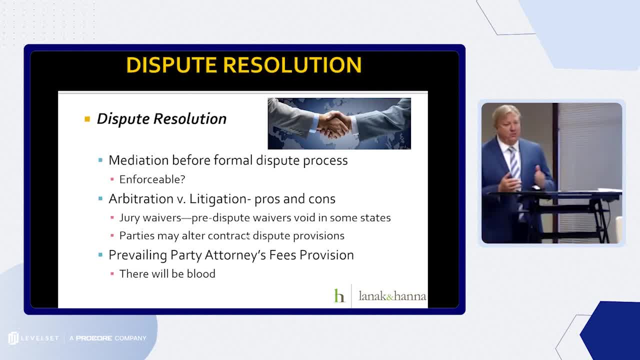 A jury, if you just think. I mean when you're litigating for a judge, you're dealing with someone that doesn't know construction. It's much easier to put on a case in front of various construction arbitrators and go with the lingo. 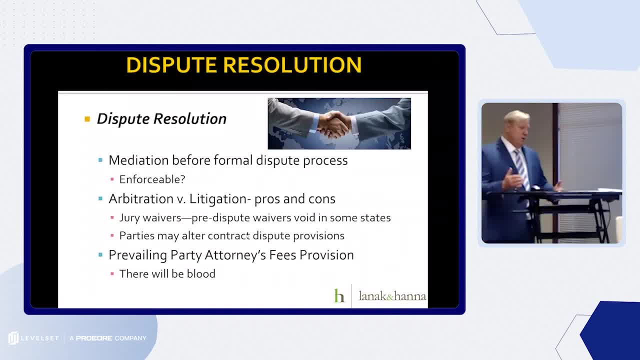 You don't have to go through everything like what the change order request was. You know whatever. There's a million things that you can think about in the construction industry that are really terms of art that people in industry speak like they're just talking, you know out of hand, which are very foreign to most people. 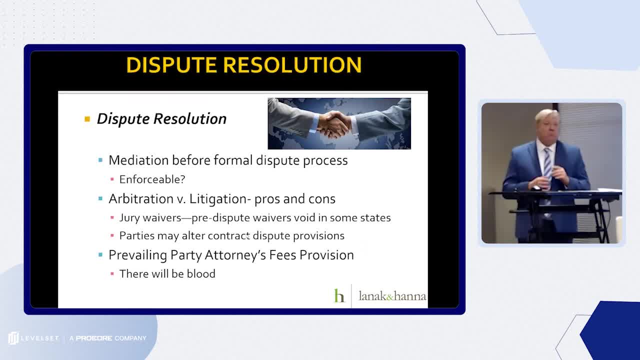 One thing I will say about juries is that a pre dispute jury waiver is illegal in some states. It's illegal in California. So you- there's a lot of contracts that say this- is that we all agree that this is people who handled in the Superior Court of Los Angeles County. 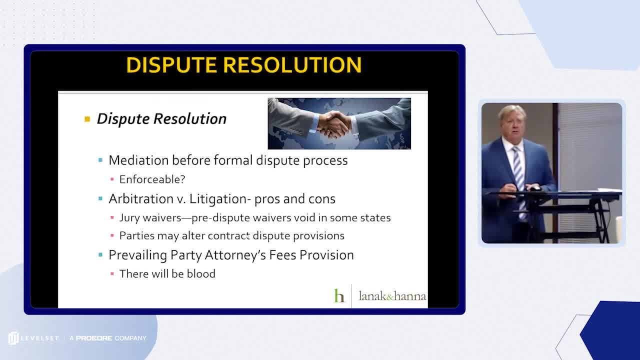 Both sides agree. Both sides agree to waive jury. That's illegal in California. What's not illegal is that after dispute happens, you can decide how you want. the parties after dispute happens can decide however they want to decide their dispute. In other words, if there's an arbitration clause in a contract and after you guys initiate arbitration, off that process and you say you know what? 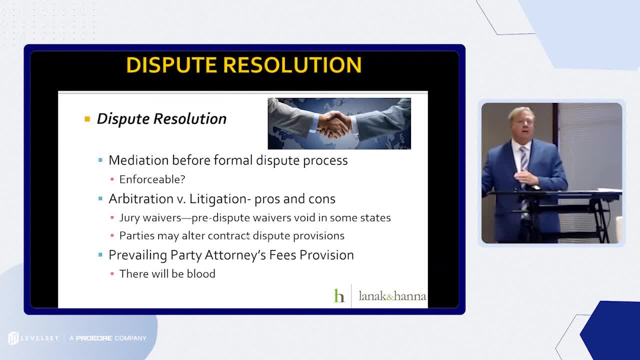 We don't want to go to arbitration, We want to go to litigation. You both agree? Fine, The same thing is true in the reverse. Frankly, if you would choose litigation or arbitration, you decide, Let's go out, and you know, draw straws. 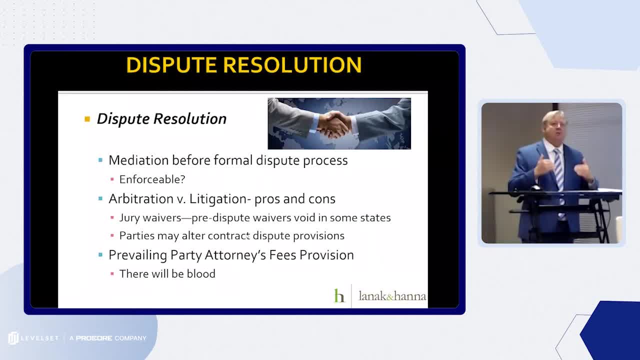 Fine. Whatever you want to do, that's fine. Once you're in the dispute, you basically control your own destiny. Arbitration versus litigation- Just real quickly. a lot of times people say: wait arbitration. what I don't like about that is there's essentially no appeal rights. 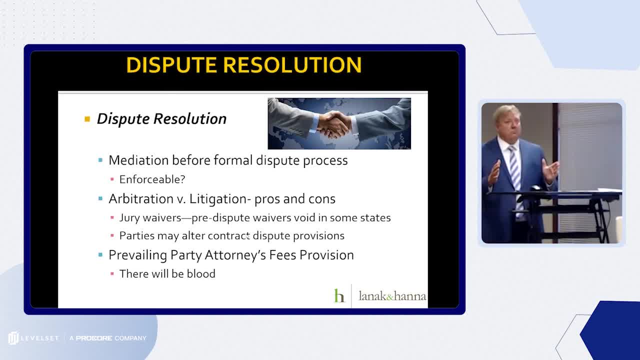 Very hard to appeal an arbitration decision. That's true. It's also true that the arbitrator, at least in California, can get the facts wrong, the law wrong and there's no appeal from it. You're stuck with it. That's obviously not good. 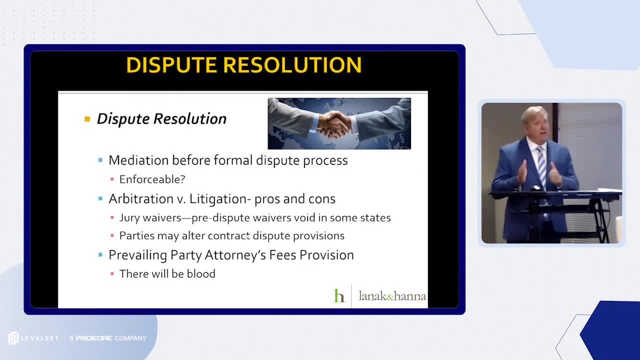 What the pro of that is- obviously the pro of that- is an end. There is no appeal. You're basically stuck with the situation. Litigation does have the advantage that you can appeal, But as a practical matter, if there are findings of fact made in the litigation process. in other words, yes, that was in the scope of work or no, that was not in the scope of work. 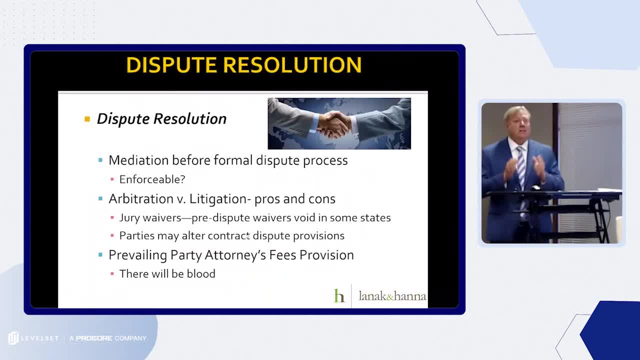 It's going to be very hard for the public court to overturn that. If it's an issue of law, you have a much better shot of getting that. getting that overturned, In other words, issue of law being like, for example, the delay clause, is not enforceable, something of that nature. 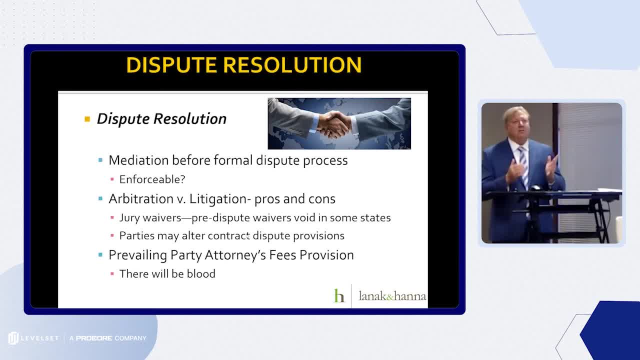 But you know so arbitration has its pros. You know, the great advantage of arbitration is that you control the arbitrator. you select it and you decide when and where the arbitrator is going to happen. Largely, litigation is pretty much a crapshoot. 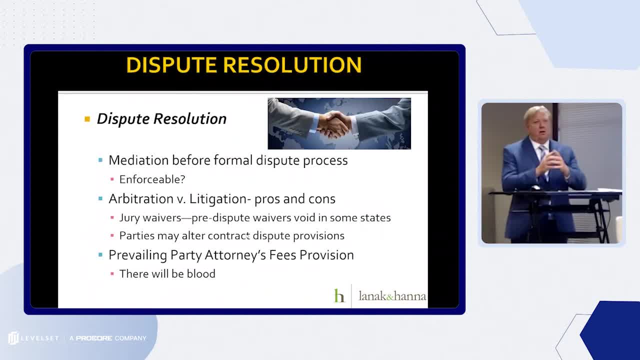 But you know, like I said, there's no appeal, So there's pros and cons for both ways to go. The last thing I'm going to talk about, I believe, is prevailing parties' turnkey provision, So there will be blood. 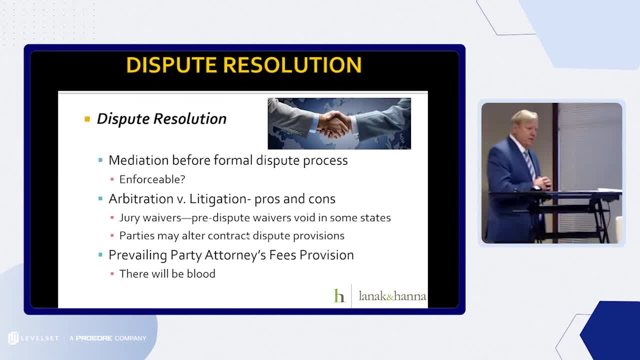 If you're deciding whether you want an attorney to get revision, think about this. There will be blood means that litigation is incredibly expensive. It just is. It's one of my former partners used to call it the blood spore of the rich. 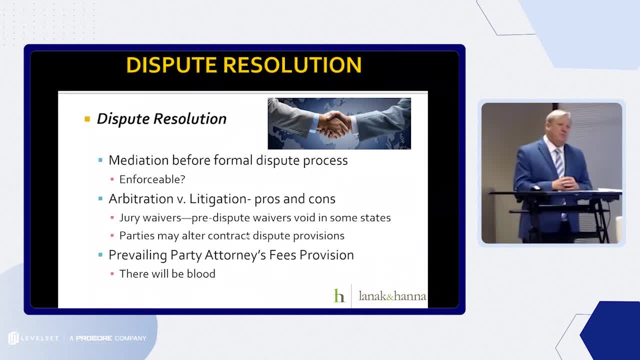 And what that means is, If you're thinking about attorney's fee revision, if you are the big guy, if you think you're gonna have more financial wherewithal than the party you're gonna be in dispute with, You probably do not want an attorney's fee revision. 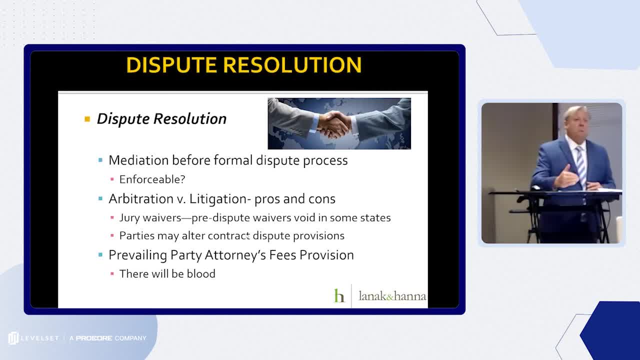 The reason for that is if you, because then you can flood in the other side, frankly, by having more, more attorneys throwing more things at the smaller guy, so that you basically beat him up through a war of attrition If there's an attorney's fee provision. 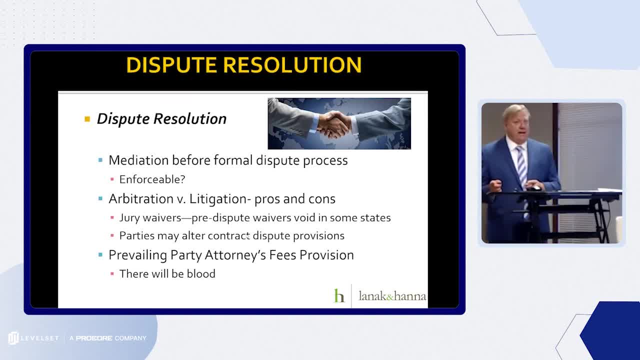 That's fine. That former guy may be willing to engage in that process. If he thinks he's an upside, he gives the 30-piece back. So maybe it's somewhat counterintuitive. but think about who benefits if you're negotiating a contract. 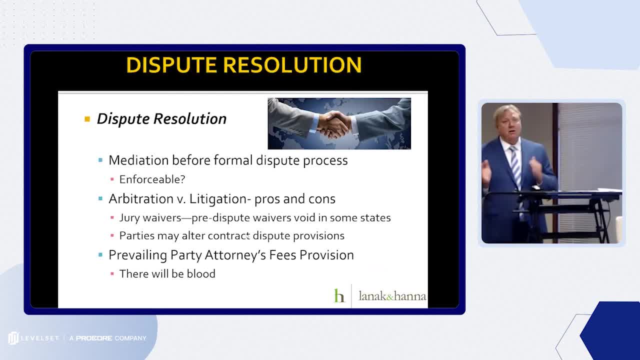 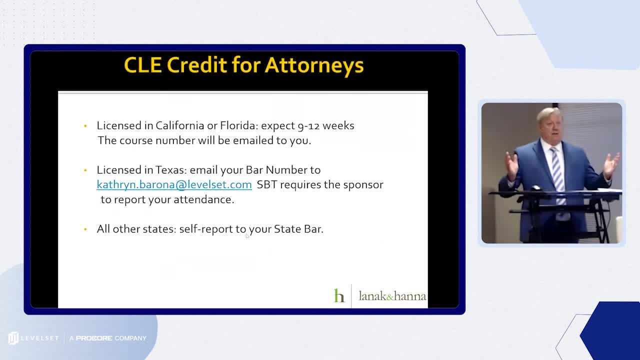 or if you're deciding whether a 30-piece division should be in a contract, Think about that dynamic And let's see. I think that's the end. Maybe I'm on the wrong side. Thank you, No, that's it. 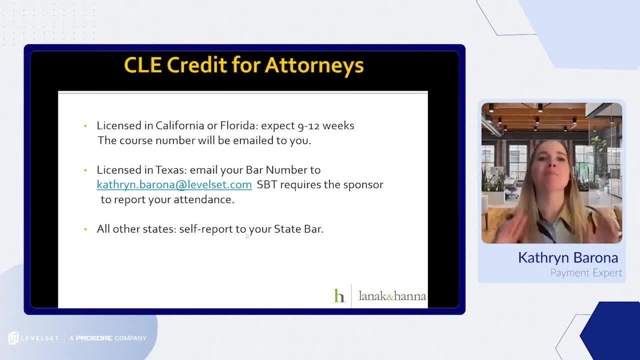 It looks good. I have a question for my last slide. Yes, Here we go, though For the attorneys you can go one back, Mark for a second. For the attorneys, you will get this information in an email as well, with the follow-up email that's coming Friday. 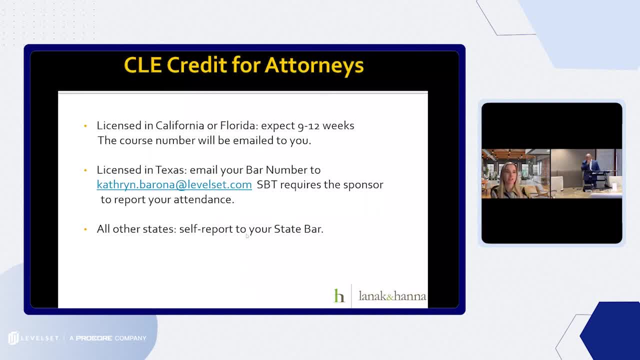 But right there on the screen. if you are an attorney licensed in California, Florida or Texas, there are special instructions for you, Especially Texas. you need to send an email to me, katherineverona at levelsetcom, with your state bar number. 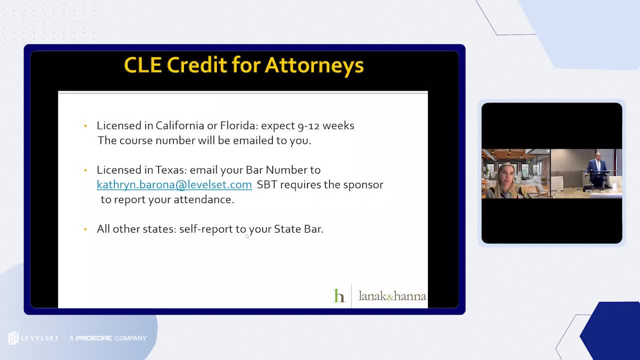 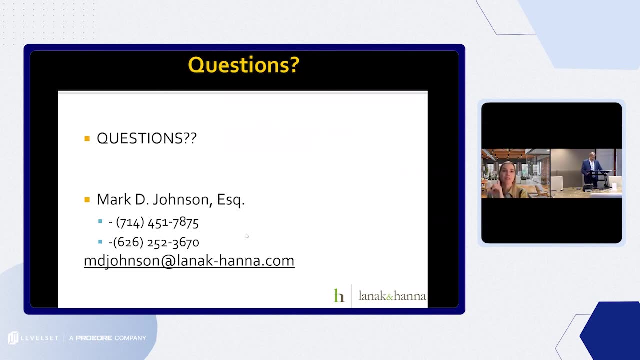 And all other states. you're going to self-report to your state bar, so check with them for the instructions. And, Mark, we do have several questions. Are you able to pull up that Q&A box at the bottom of your Zoom screen? 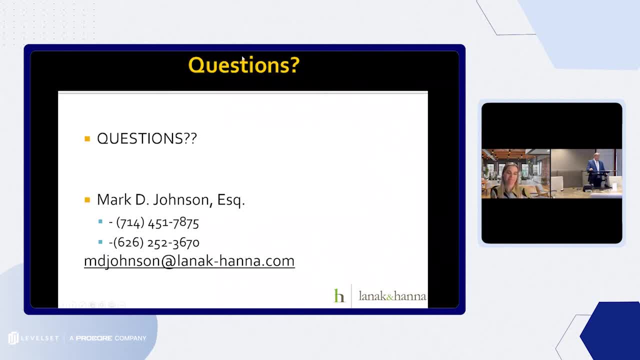 That's where the The questions are typed in. Yeah, but I can't read them, so Okay, Well, I'll read them off. So Wait a minute. There's like 30 questions. Well, there's. 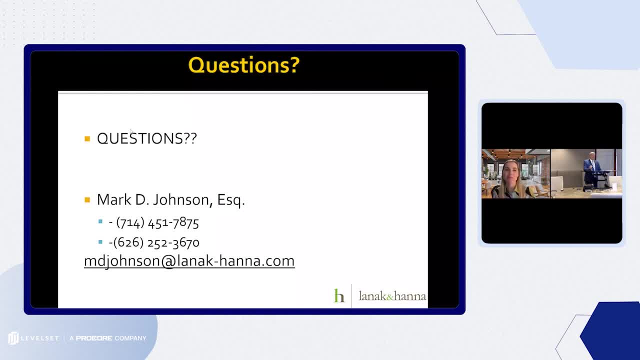 Okay, there's 18, but I was going to tell people we don't have time to get to all of these. We're going to hang on for however many Mark can get to, but if you, That's fine. Katherine, I will say my contact information is on the screen. 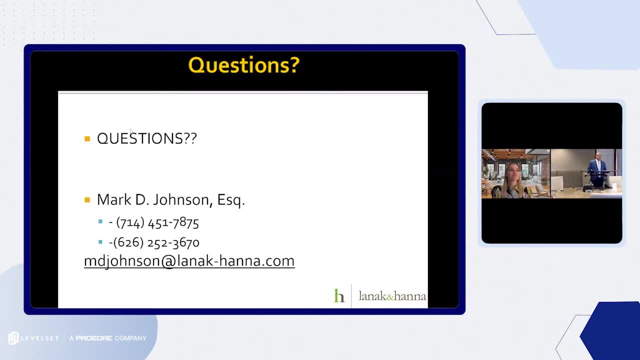 Yeah, If you guys want to send it to me, If you guys want to send me an e-mail, I'll be happy to answer questions, But go ahead. Sorry, Sounds good. First one from at 120 was: what about the Spirin Doctrine on Defects and Inefficiencies in the Plans and Contract Documents? 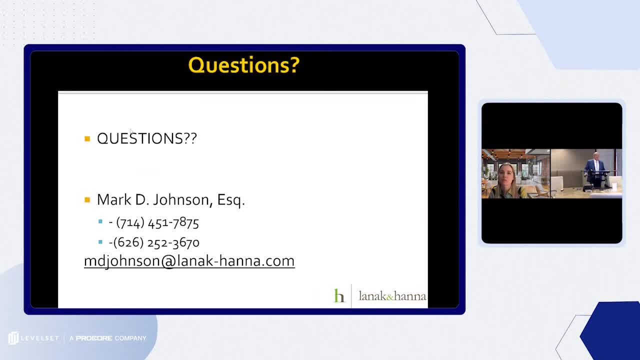 Spirin. you know, I don't know if Spirin does apply, but Spirin is basically the case that talks about what kind of costs and damages you can get And how you deal with deficiencies, But also it's most notably cited for the proposition about how you get investigation costs. 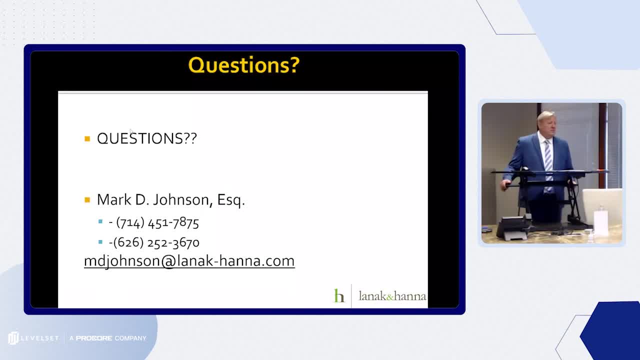 I'm not sure if I answered the question, but yeah, Spirin Doctrine applies in California. Okay, Next question: Does Great Western drywall versus rural construction serve as a good precedent for not equally spreading back charges or LDs? I think, ultimately, if you get into a dispute about who's responsible for back charges or LDs, contract provisions that talk about splitting them equally or something of that nature, you can probably defeat. 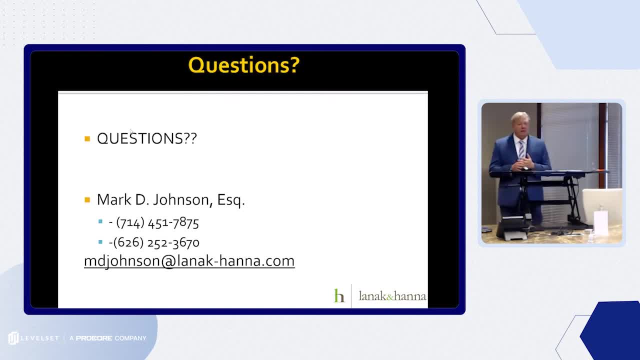 Because when you think about how it plays out really, you're probably going to have cross claims that go back and forth And there's going to be a finding of who does what. Now, that's probably, That's probably not a very likely situation in terms of actually litigating about that. 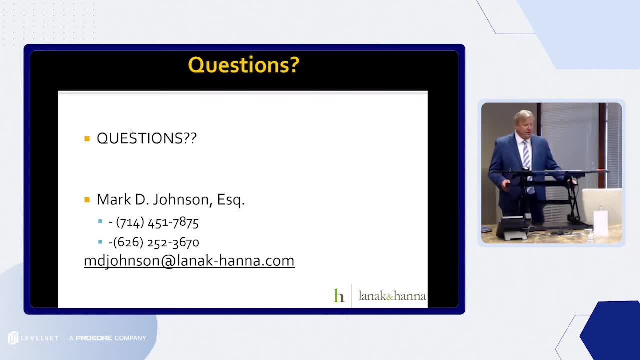 But my answer would be that I think that you're actually going to be able to talk more about equity again in terms of how that's dealt with. Okay, Next question is: most flow-down clauses is usually a one-way conduit. Should we fight for the same rights remedies? 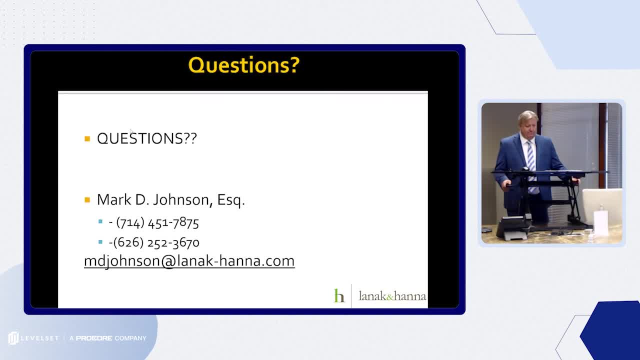 And redress towards the contractor that the contractor has with the owner? The answer to that question is sure. I think it's a. So first of all, yeah, you're right, The flow-down provision typically is kind of a one-way street. 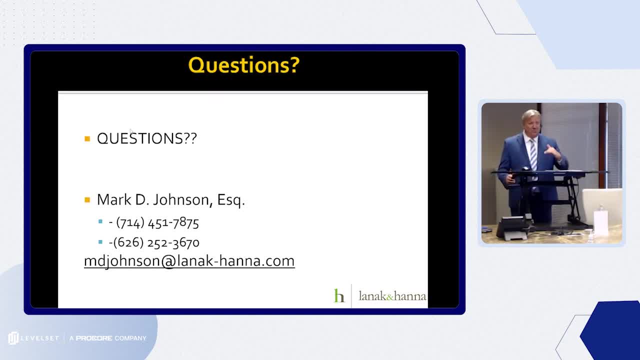 And basically the contractor decides what provisions he thinks are helpful, but he can flow it out to himself. So would it be ideal if we could have a reverse concept? Sure, Whether you can negotiate that or not, I don't know. 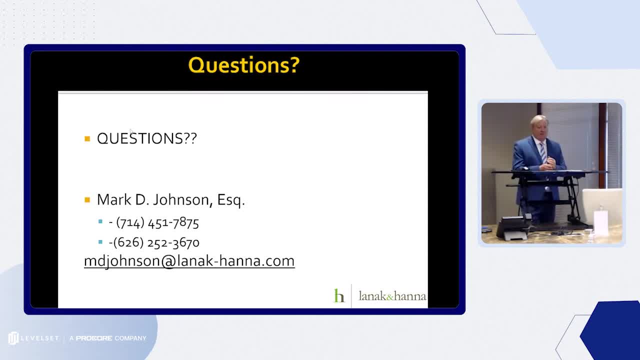 For example, like the damage or delay clause. I mentioned that a lot of them say there's no damages for delay for a subcontractor But in turn the subcontractor is responsible for any delay that he causes, and then that the owner hits the contractor with. 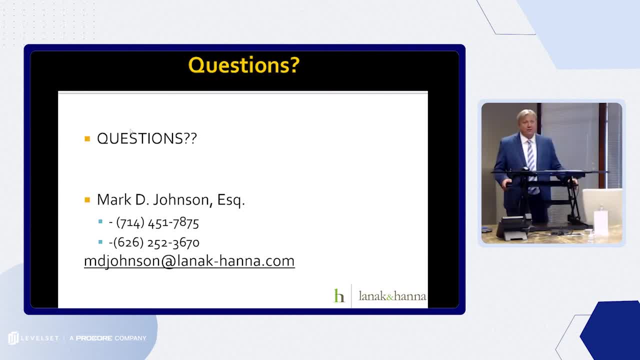 So sure It would be better if you could make it a two-way street. I just don't know if you're going to be successful doing that. All right, Thank you. Thank you, Julie asked: how successful have you been at negotiating out LDs and how are you handling anti-indemnity states? 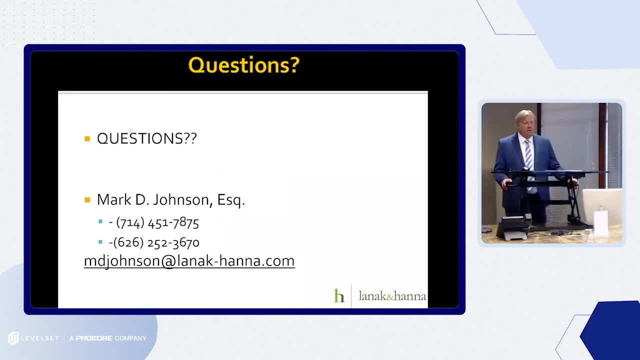 So the answer to that, negotiating out LDs, I would say a public works project, zero In private works. you can try to get a better luck, And I have had better luck in limiting it or making it more specific and at least carving out provisions. Anti-indemnity states. I mean, I'm not sure exactly what the question is, but I guess I'll just say that, yeah, in states like California there are provisions that I wouldn't call anti-indemnity, but definitely provisions that limit civil indemnities. 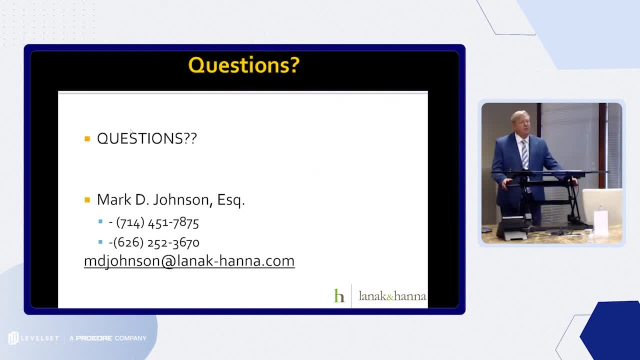 So certainly be aware of what I mean. rather than having an indemnity clause that contains circumstances that are arguably void or illegal in your particular state, the extent you can try to negotiate them out, that's easier. It's just easier to deal with. 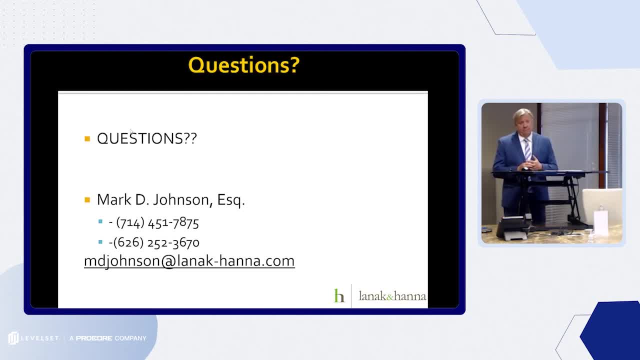 It's just easier to deal with everything on the front end in my experience. Okay, thanks, If I get paid late, but I already gave the prime a release, can I sue them for prompt payment penalties? I got paid late, but I already gave the prime a release. 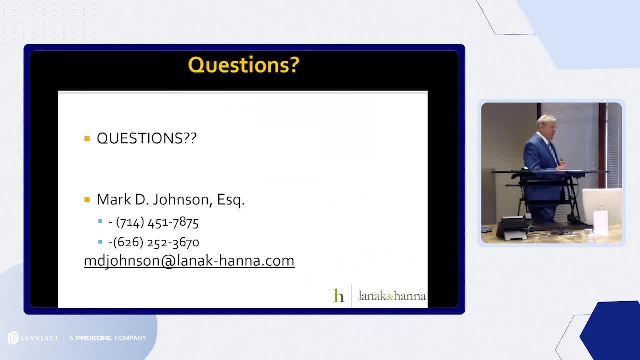 Of your own. The question's a little bit vague, but if you got, If you gave this, Well, so I think what you're saying is I gave the prime a release saying that I got paid, but I later sued the sub, the prime, if, in fact, I gave the release without being paid. 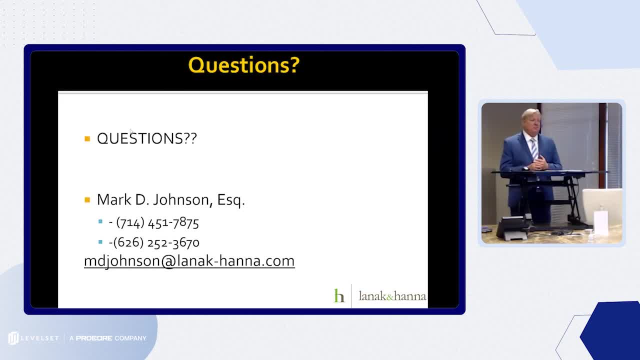 That's the question. I think the answer is yes, because you effectively gave the release assuming or conditioned upon the fact that you would get payment, and if that condition never happened, then you would argue release is invalid. I hope I answered that question correctly, but if I did, that's my answer. 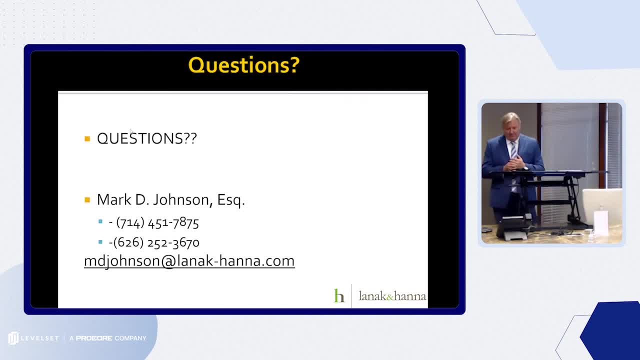 Okay, what can a subcontractor do to avoid forced mediation? and no arbitration or litigation clauses, That's all. So what can a subcontractor do to avoid forced mediation? and I'm sorry, what was the last part? No arbitration or litigation clauses. 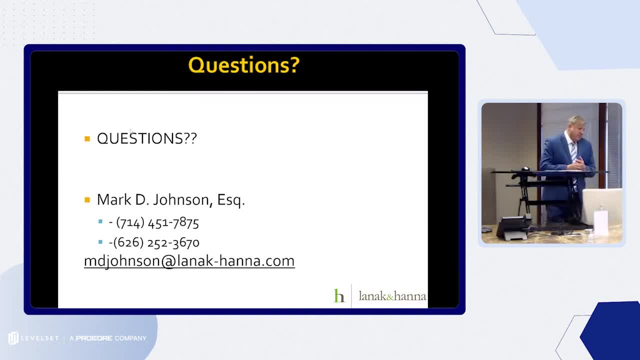 Okay, so forced mediation I mean basically if you don't want. Well, first of all- again assuming you negotiate out that in the contract, if there's a mediation clause and you don't want to do it, you can basically proceed to go to mediation and then, if you are the party that has a claim to assert, you can proceed and file a lawsuit or arbitration and just argue why it's not enforceable or why it doesn't matter. 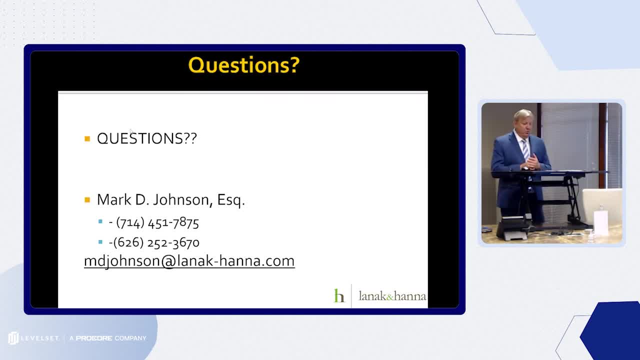 Frankly, I think a lot of judges view Mediation, pre-mediation clauses is kind of the check the box, so if the parties don't want to go to it, there's really no sense to make them go to it. So that's not a. 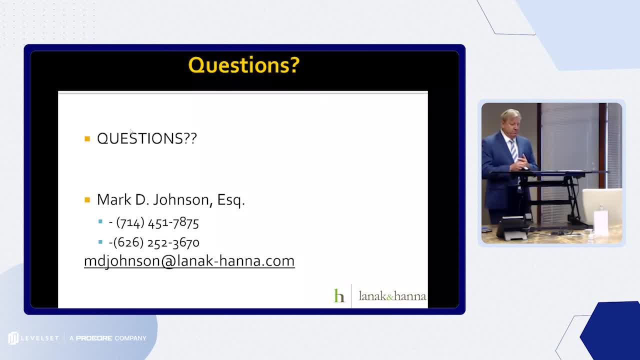 That's more of a practical answer than a legal answer. I suppose The second part of that was: what if there's no arbitration and it requires litigation? The answer is: if there's not an arbitration provision, you cannot force a party to go to arbitration. 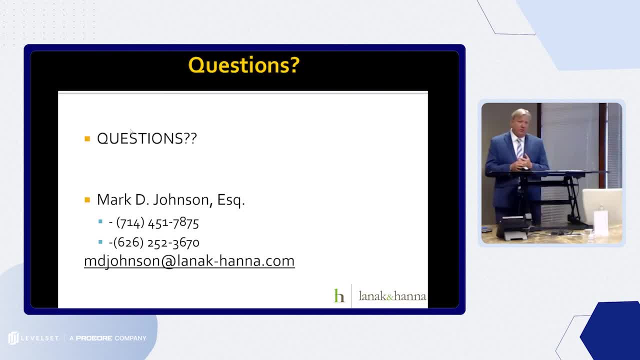 Arbitration can only be enforced if there's a contract calling for it. Arbitration can only be enforced if there's a contract calling for it. The flip side, though, if there's an arbitration clause in a contract and you don't want to arbitrate and you don't want to go to litigation- you can bring a lawsuit under the contract and then deal with. Sometimes maybe the other side doesn't want to go to arbitration either, and once you're submitted to the jurisdiction of the court, you have waived your arbitration clause. The other side wants to enforce the arbitration clause. 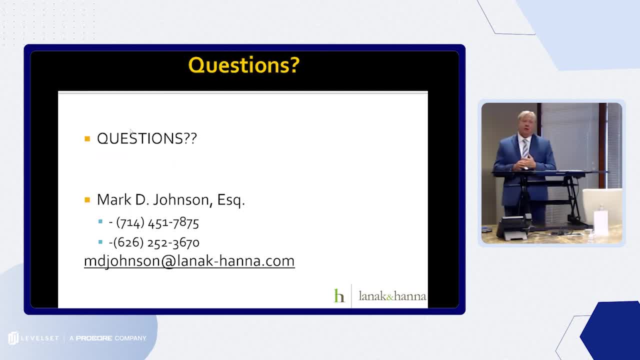 It would be his or her burden to Compel you to go to arbitration. Okay, Next question: How about mobility charges on a contract, Mobility to be paid by a certain percent of the contract is completed. That's part one of the question. 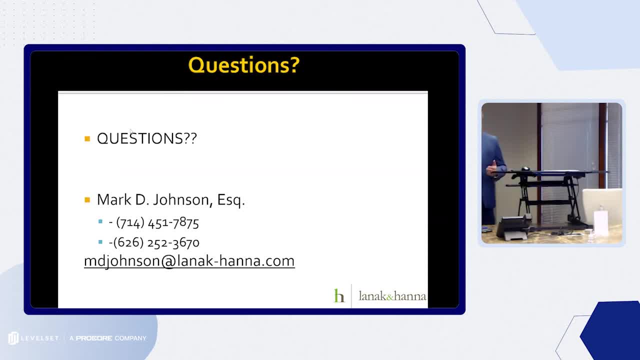 Well, I assume mobility means mobbing and de-mobbing, but I'm not exactly sure. But if that's what it means, the contract certainly can specify certain provisions and what you have to do to pay. That would be no different than you know. we're going to pay you based on percentage work done in a particular time period. 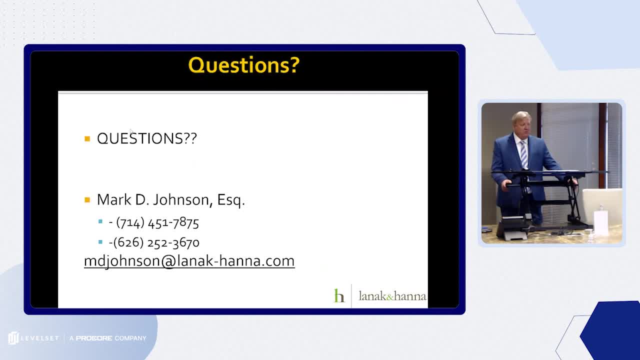 So I'm not really sure what the question is, but the contract can clearly specify time period when you get paid. It can be by a certain, you know, period of time, every 30 days. It can say that you'll get paid a certain percentage based on completion of work.